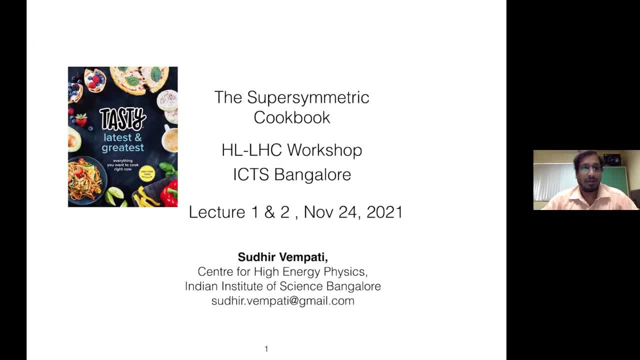 neutrino masses, dark matter and other things, And it's a pleasure to have Professor Bhempati today. He's giving this lecture- the two-hours lecture, And amongst the many accolades, he is honored with the Bhatnagar Award in 2016.. And today he's going to talk about the SUSY spectra. 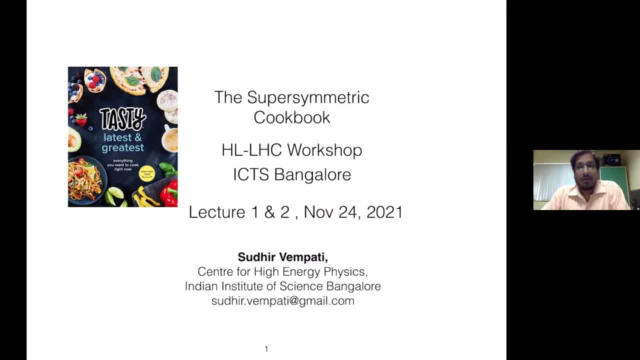 generation and Higgs, et cetera. So, without any further delay, I request Professor Bhempati to deliver this lecture. Thank you, Pradaya, very much, And thanks to Rohini Seema, Sanjay and all the organizers. 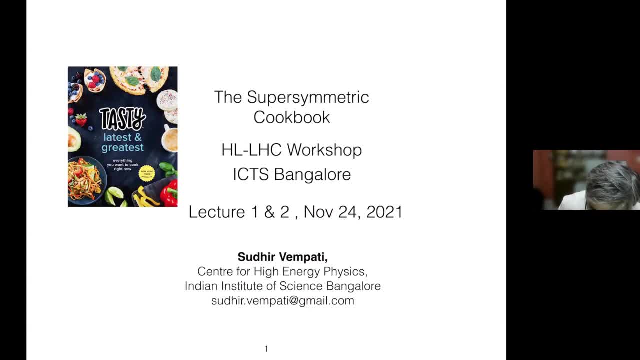 for giving me this opportunity to talk about supersymmetry, which is a topic which I like very much. Okay, I have no qualms in saying that And I believe I think there is some hope of seeing it at some point. actually- And the conference is addressing a very important 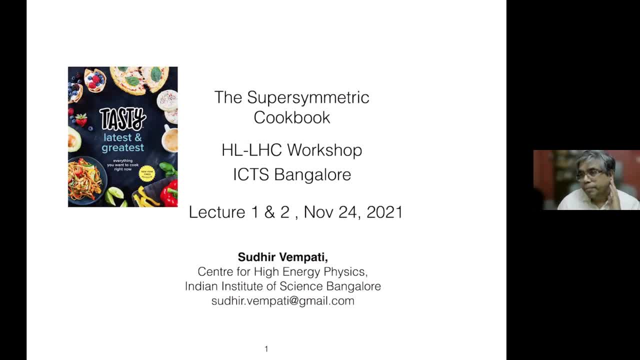 issue whether we can really have some implications of supersymmetry in, say, the Highland Monastery run of Large Hadron Collider. I have been asked to give you some sort of pedagogical lectures on how to build the supersymmetric spectra. how does one build the supersymmetric? 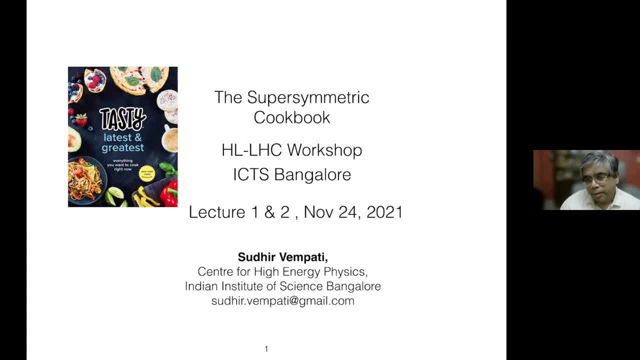 spectra and then compute the spectra and then say if you want to get the Higgs mass out of it, how will you do it, And then compare it with experiments. So my lectures will be extremely pedagogical. I'll go slowly. Ideally I wanted to do it on the blackboard, But so first part of the slides: 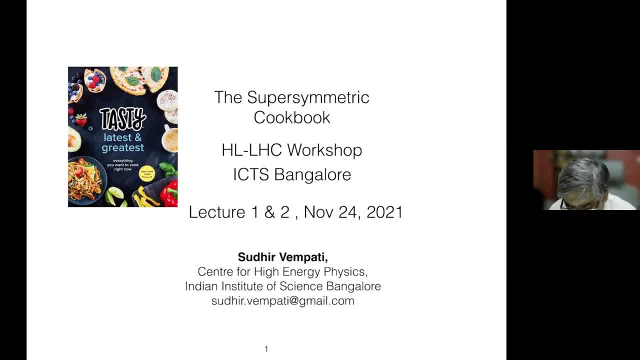 I have made some slides and everything and I'm using an iPad, So feel free to stop me at any point. actually, Just feel free to stop me at any point, ask any questions And I'll be trying to do it. I'm trying to do as much pedagogical as possible And if there are any questions, just ask me. 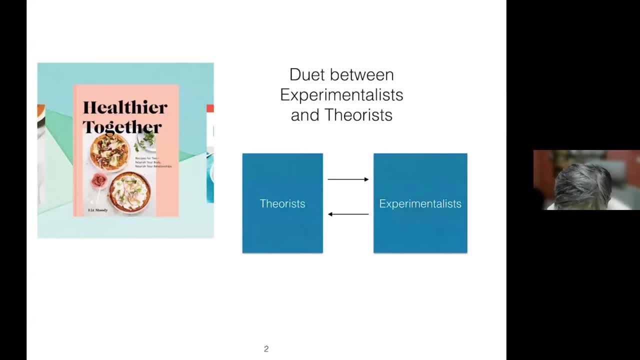 So, to start with, actually what we have in high-energy physics is some sort of a deal between experimentalists and theorists. So theorists build some models and they have these nice theories and everything and they make some predictions, And the experimentalists 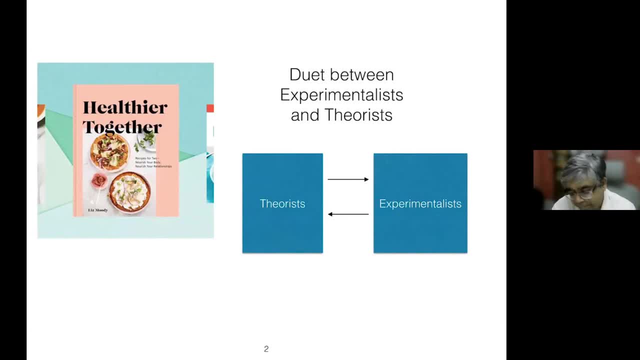 test them. And then, of course, they say, OK, this model is wrong, this model is correct, this model is so-and-so and so-and-so. On the other hand, you have both the cases. In the case, you find some very smart experimentalists. 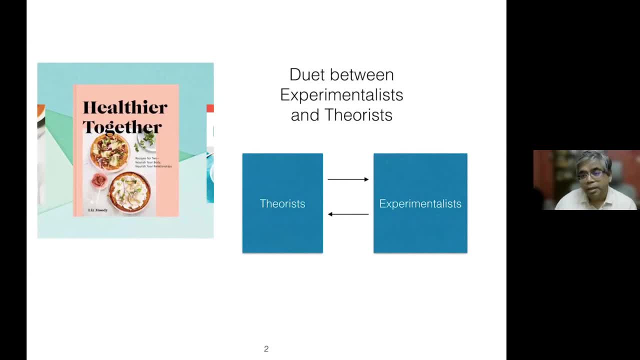 find some signals and everything which cannot be explained by the present theories. So the theories have to go back and rebuild the things. OK, And they have to rebuild the things and the models and everything, OK. And so all the physics beyond the standard model, they have to go back to the drawing. 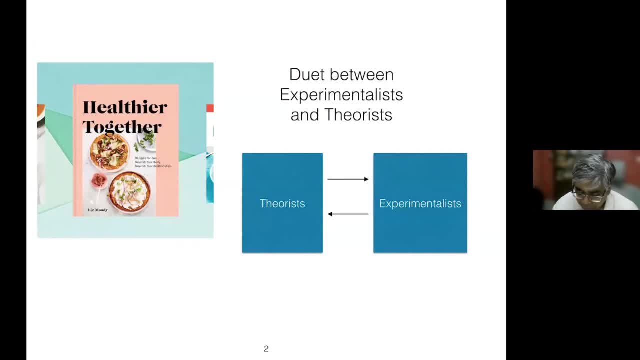 board and then come back to again modify your theory, existing theory. So anyway, it's some sort of a deal between experimentalists and theorists, And I don't think one should. I personally think one should work with each other rather than criticize. 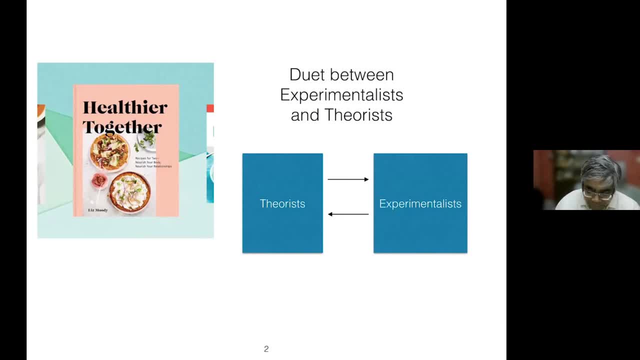 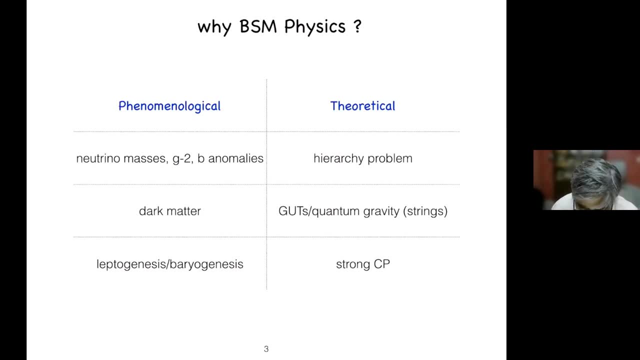 each other, I think. So my thing is that why do you need to go to a physics class? Why do you need to go to a physics beyond standard model, Say, for example? you have various reasons. OK, These are all the reasons, which are both. 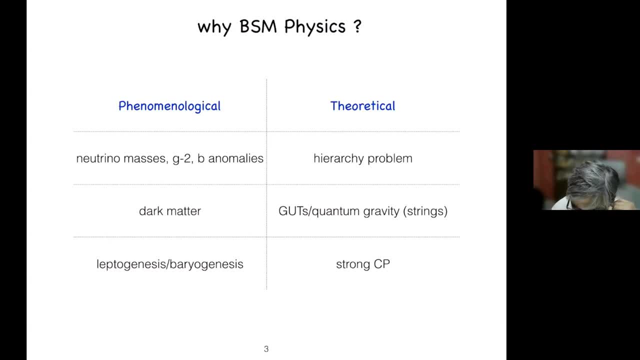 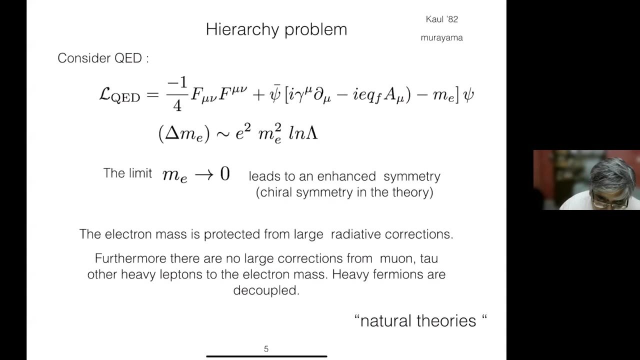 phenomenological and theoretical. There's a hierarchy problem. in the theory, then there's a grand unification, that's a strong CP problem and so-and-so. On the phenomenological direction, you have non-zero neutrino masses. In fact, what is interesting is this, the first set of this list. this is completely 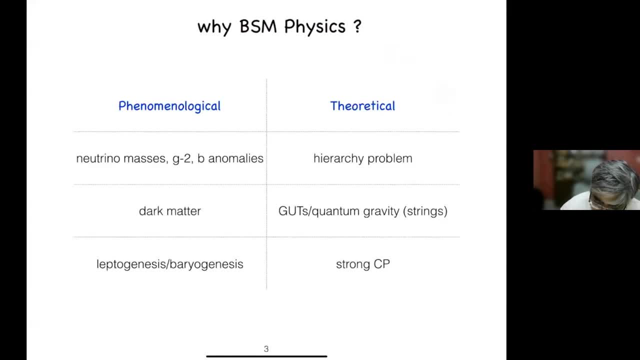 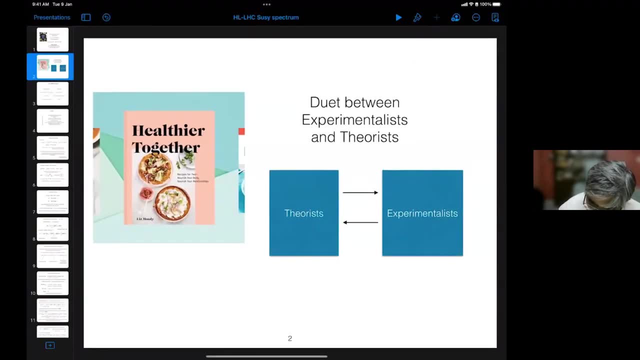 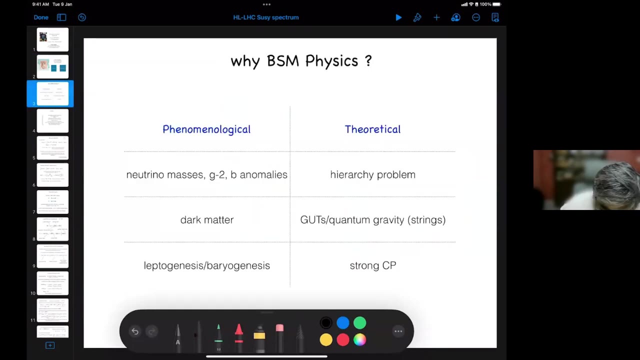 a One second. OK, let me just go into something. So in this first set, all these things have no analogy in the standard model. So, for example, the recent measurement of g-2, updated measurement of g-2, the physics. 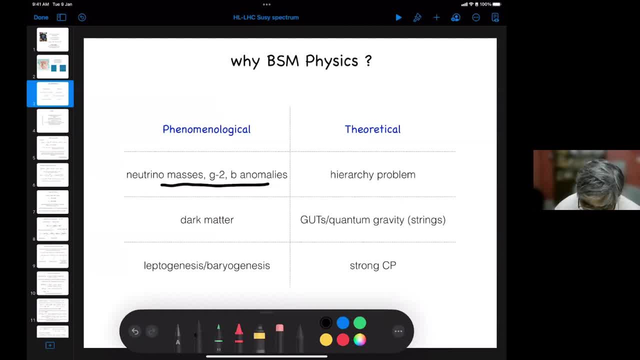 anomalies, So-and-so. They don't have an explanation in the standard model. Similarly, dark matter, Of course. then there is the issue of leptogenesis and baryogenesis or baryogenesis. For all these reasons, we need to build some models to go for physics beyond standard model. 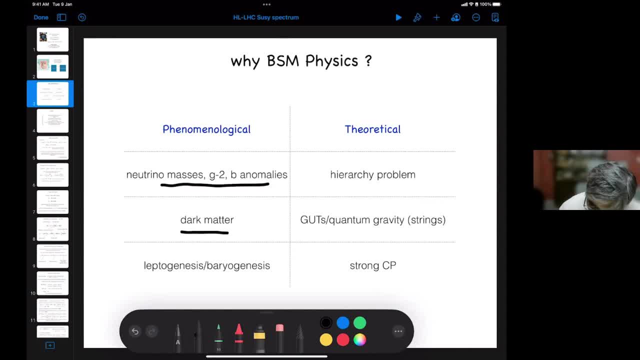 And one important thing I want to mention is the discovery of the Higgs. My belief is that the discovery of the Higgs- OK, The discovery of the Higgs, which is very light, OK, If you want, theoretically, the Higgs could be extremely heavy. 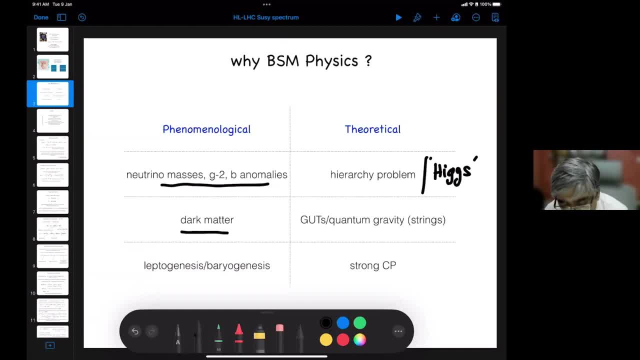 There is no limit on the Higgs mass, But the Higgs mass is very light. It's actually lighter than the top core mass. So what? it means that there is some symmetry which is protecting the Higgs. OK, this could be some non-perturbative symmetry, like composite Higgs or so-and-so, because 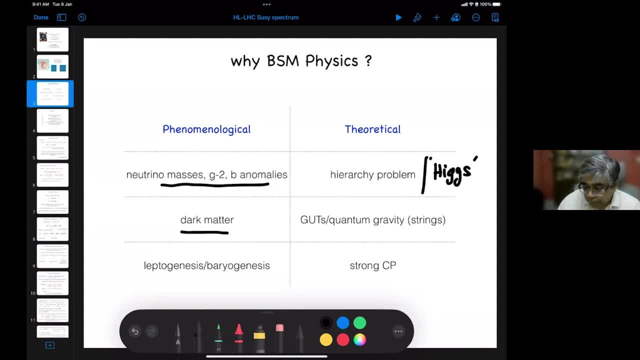 in turn, it could be like a pion or so. on the other hand, there is a symmetry which protects the Higgs mass very, very well. it's a different matter that we don't see it. okay, we don't see it in the exponent at the present. 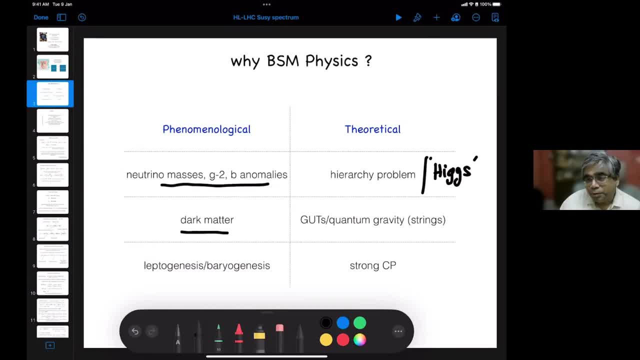 exponent element, and the reason why we don't see it also is because the Higgs is around, almost at the edge of what is predicted by the MSSM matrix. so why we don't see the rest of the supersymmetric partners or something is also because the Higgs is around 125 G. 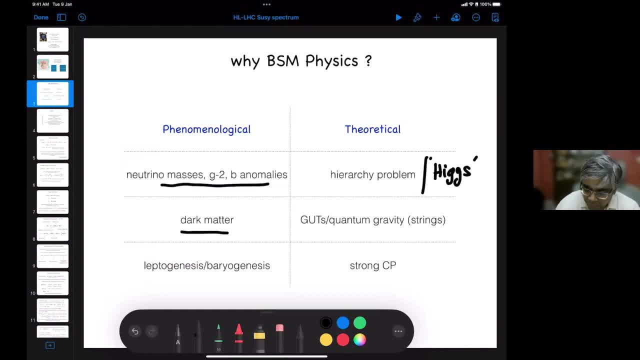 V, but just purely from the standard model point of view. you have a light scalar that's around 125 G V and then you have a hit. the fermion masses are also much heavier when you talk about this, heavier than the Higgs. so it looks like there is some symmetry, which 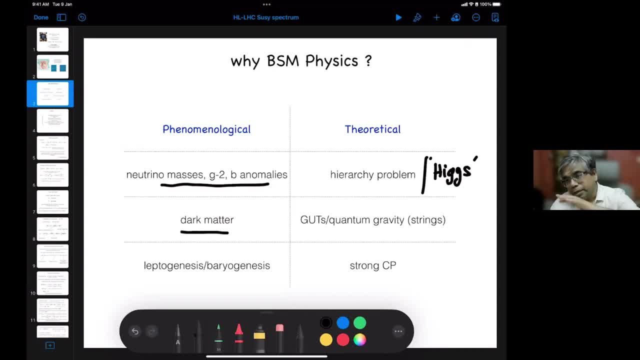 is protecting these things very well. so it's protecting the Higgs mass very, very nicely. so this symmetry, one of the best symmetries you have, is supersymmetric case. the supersymmetric theories really protect the Higgs mass up to large radiative corrections and so on. so 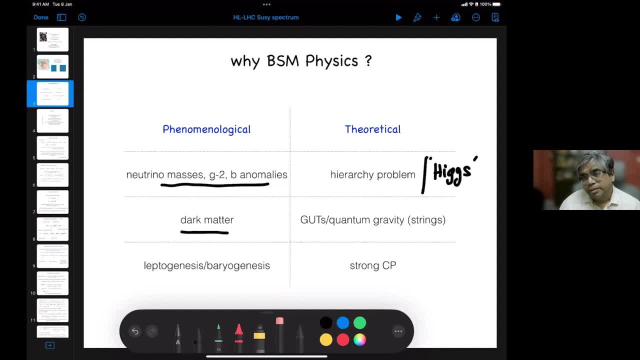 and once supersymmetry is broken, it's actually those radiative corrections which play an important role for the prediction of the Higgs mass, those radiative corrections which play an important role. so, anyway, since you already know most of this thing, this why we will motivated. 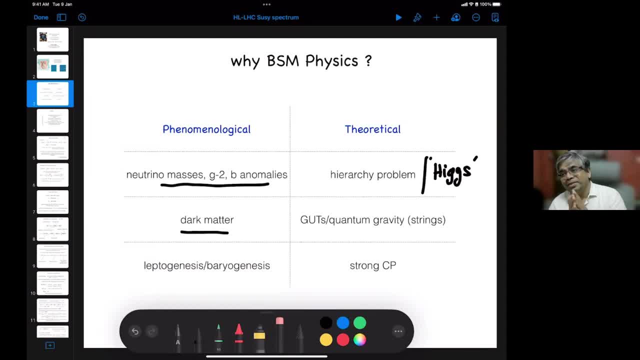 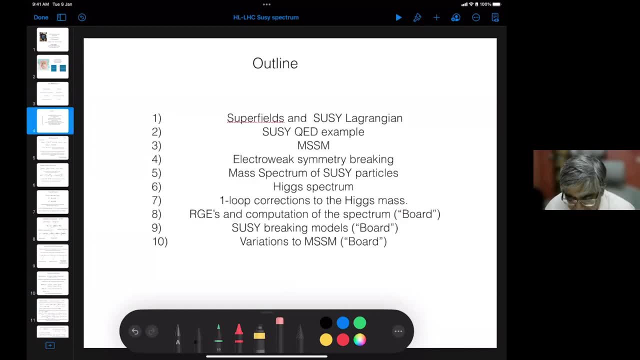 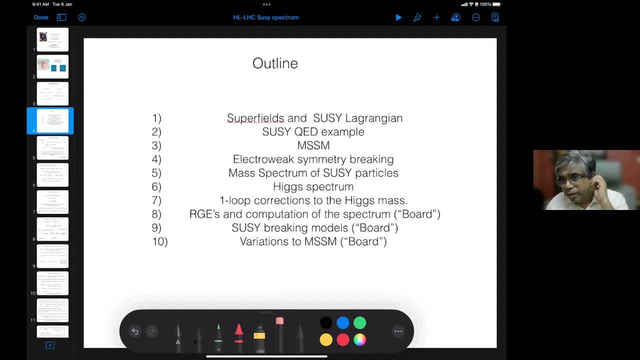 how do you write a supersymmetric Lagrangian? and I'll give one example, because that way we can understand how to derive the spectrum for a supersymmetric theory. so, since my mandate was how to derive a spectrum and how to compute the spectrum, so I'll give you a simplest example. 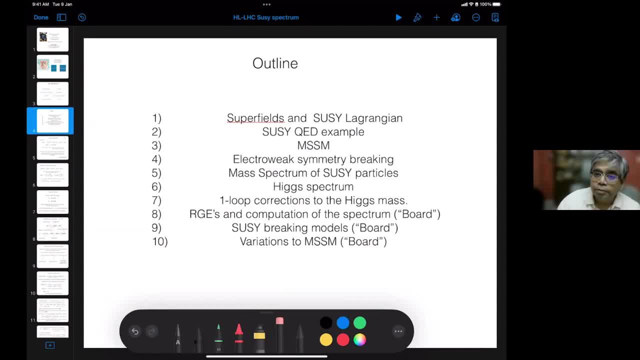 of supersymmetric QED And then generalize it to MSSM. I'll talk about how to introduce electroweak symmetry, breaking the mass spectrum of supersymmetric particles- Higgs spectrum- one loop, corrections to the Higgs mass and the remaining topics are also extremely important- and how we compute. 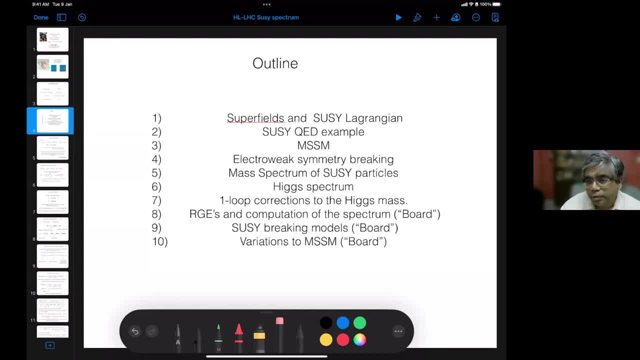 the RG equations, computation of these are all things which I'll do it on the board, many on my iPad, actually, at least I wanted to do the full thing on the board. So I'm going to do it on my iPad. actually, at least I wanted to do the full thing on. 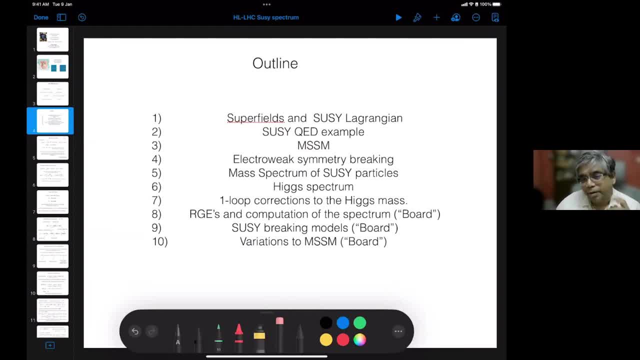 the board, So I'm going to do it on my iPad. actually I've got an iPad, but I don't think I'll have enough time. actually, Then I'll talk about how do you write what I want to end essentially. I hope I'll reach. 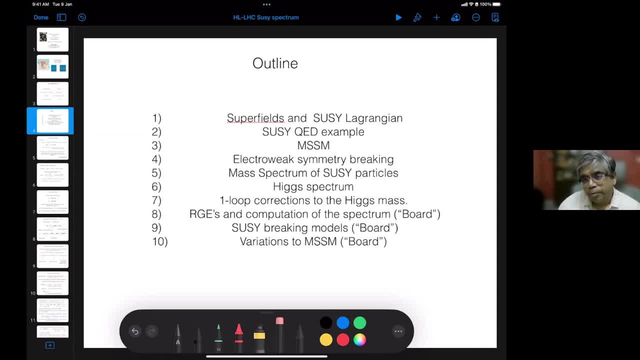 that point is that if you want to modify MSSM, if you want to modify the supersymmetric theories, how do you? simply modify them? because supersymmetry is such a powerful symmetry that, knowing a few techniques, you will be able to derive the entire full spectrum. actually, you can. 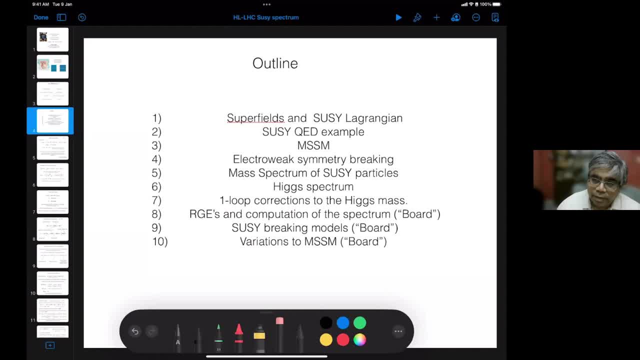 derive the spectrum, you can do the computations, execute. it's not at all complicated. actually, If you know some few techniques and few physical calculation techniques, you can do this computation very easily and you can build your own supersymmetric model, maybe with three Higgs doublets, or say, for example, NMSSM or modification. 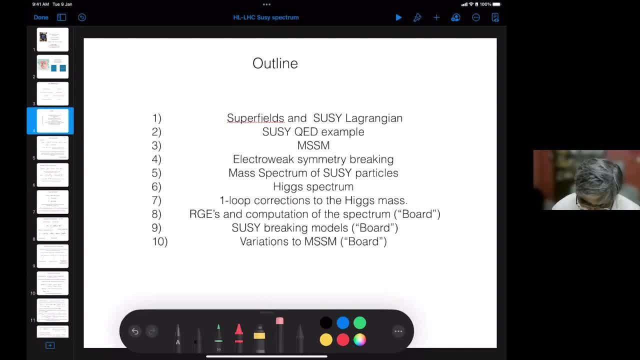 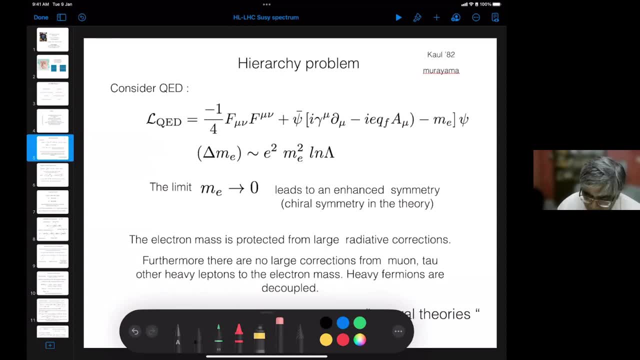 of NMSSM, with the U1, so on. So we'll see some examples how to construct them. So why do you need supersymmetry? This is a well-known problem of hierarchy problem. So, the hierarchy problem, there are several ways of looking to it. The traditional: 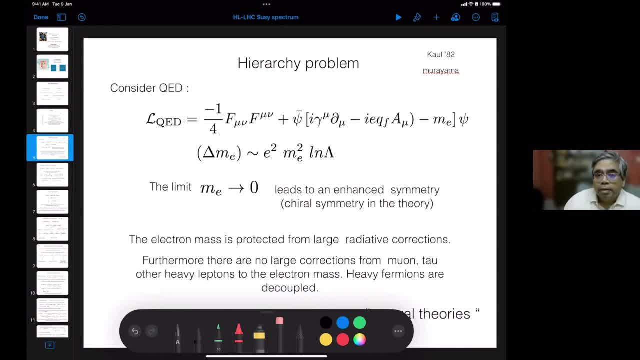 way is to look at it inside a grand theory, but one can look it into various ways. Say, for example: let's start with the QED example because we use supersymmetry, this model. so that's the reason why this is the QED example. QED is nothing but a simple theory. 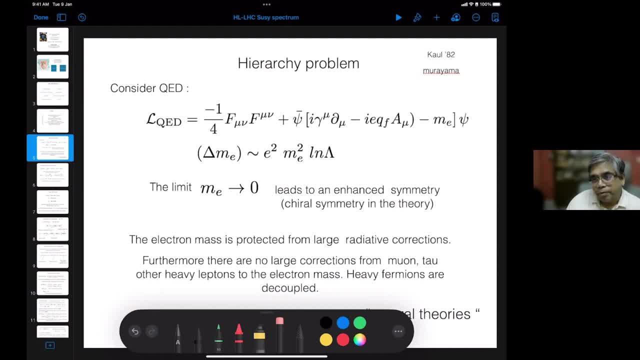 of a photon and an electron. okay, and if you take this calculation and and if you do the one loop corrections, so the self-energy of the, of the, of the electron mass, which you do in your quantum field theory course one, If you compute it it goes as alpha times. 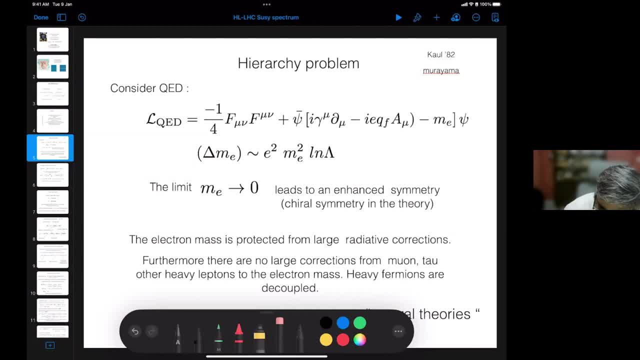 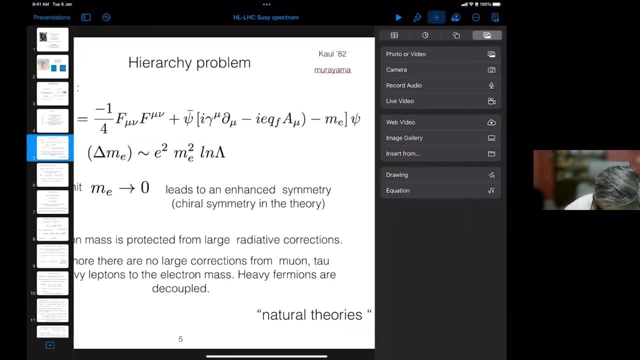 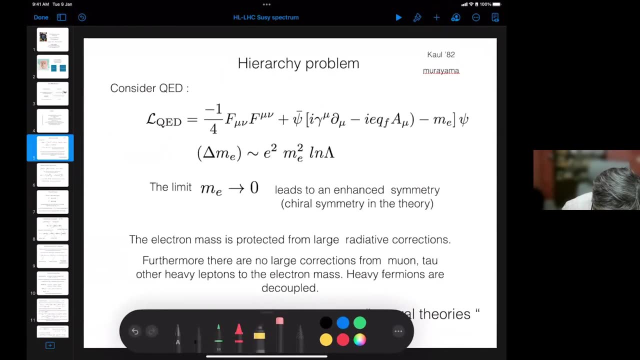 m e squared. So this goes as this particular thing. Sorry, So it goes as alpha times m e. So in the limit the electron goes massless. okay, The theory is chiralism. There is a symmetry in the theory which is called the chiralism. 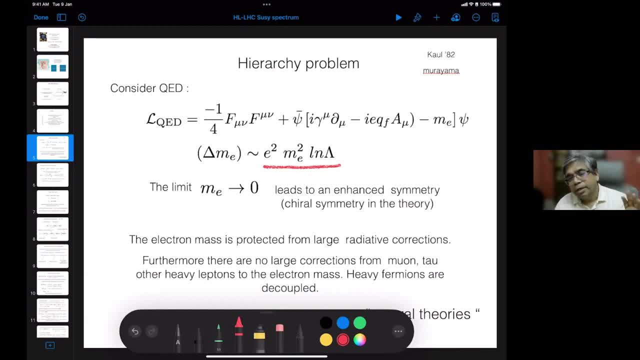 So that means the left-handed electron doesn't talk to the right-handed electron and so there are no large corrections. So if you look at any electromagnetic corrections, so to masses of these particles, they are not very large, They're proportional to themselves. Now I'm insisting this kind of a, why I'm repeating this thing again and again, is because 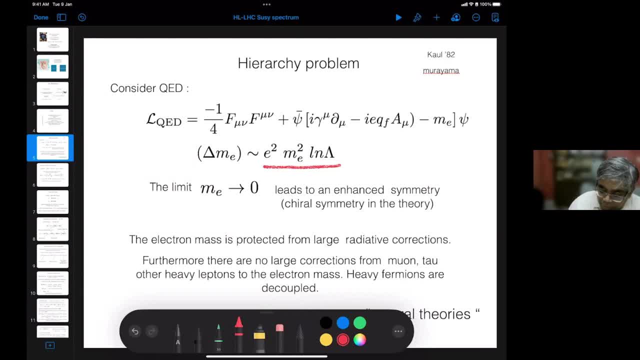 this is something which you already know, Because supersymmetry also has a very nice feature which will come, and when I'm talking about radiative corrections is that remember the point that the mass, the corrections to the mass of the electron, is proportional to itself. 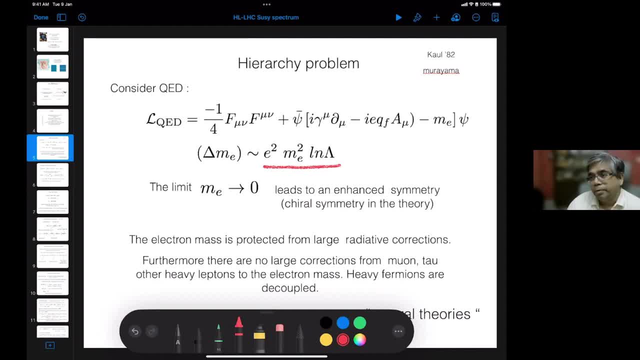 So in the limit, the mass goes to zero, the correction goes to zero. These are important point. So this is what happens also in supersymmetric theories, purely because of something called the non-denounceable theorems, which I'll come to in a minute. So anyway, coming back to the QED, 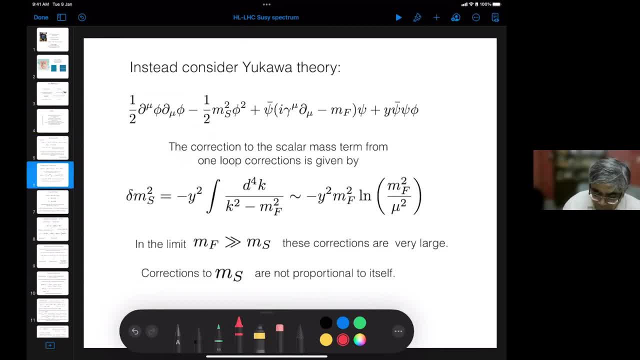 Example now: instead, consider a theory with Yukawa interactions, Instead of QED interactions, just consider a scalar theory with Yukawa interactions, Just nothing but Yukawa interactions. Now, if you do the one loop corrections, the correction to the mass, of the scalar mass is: 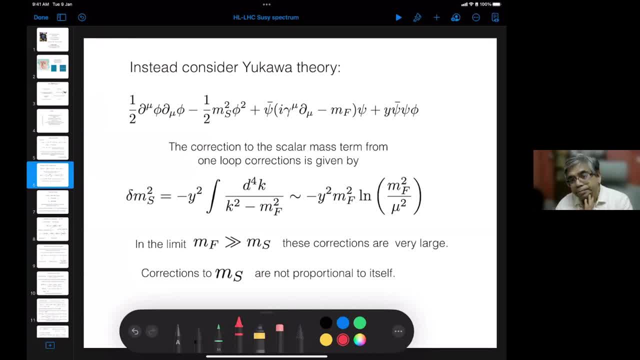 not proportional to the mass of the scalar itself, but it's proportional to the mass of the fermion. So this is your Yukawa theory, This is the kinetic term, the mass of the scalar, and this is your Yukawa coupling. The Yukawa coupling is nothing but psi, bar, psi, times, phi. 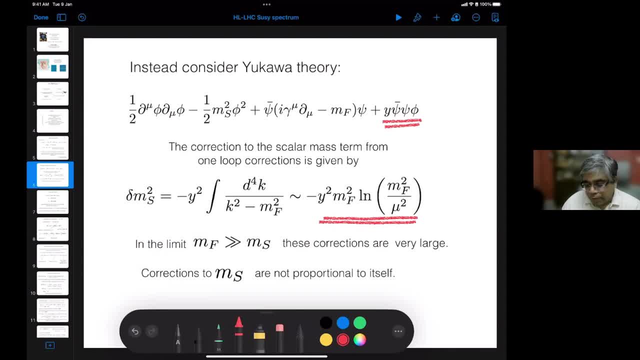 So instead of a gauge boson, if I put a scalar and compute the correction to the scalar mass, scalar mass, So it's proportional not to the mass itself but to the mass of the fermion in the theory. So, for example, you can replace this with the Higgs boson and the top quark. 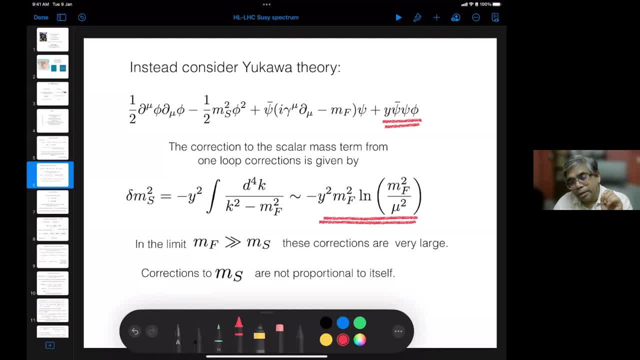 This is the exact formula you have. So the Higgs correction is proportional to the mass of the top quark, not proportional to the mass of itself, Unlike for the fermion, whereas the fermion mass correction is proportional to itself. So in the limit the mass of the fermion becomes very, very. 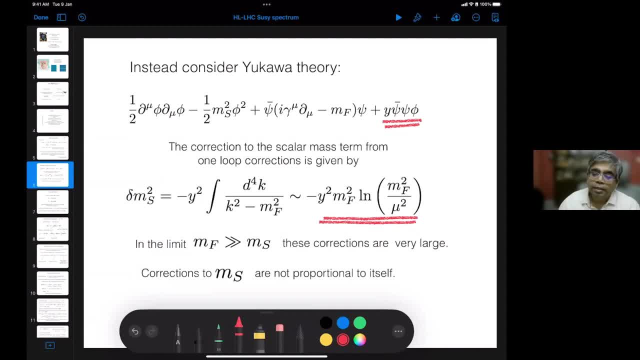 very large, this correction becomes large. So if you take the limit of the decoupling limit, if we say Mf goes to infinity, So in the limit of the decoupling limit, if we say Mf goes to infinity, The mass of the correction also goes to the infinity, or if it goes. okay. so there's a theoretical. 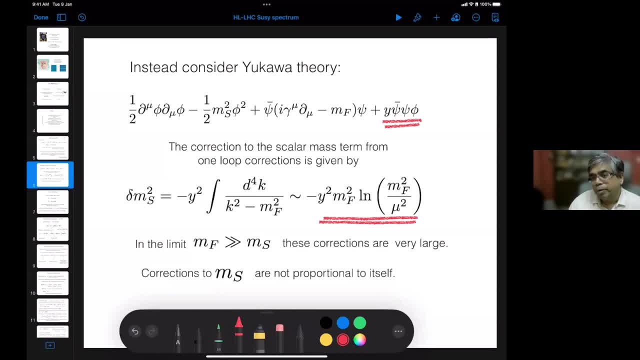 limit. but if you want you can set it to the gut scale or the flag scale or whatever you want and the limit it goes to. So if we have heavy fermions in the theory beyond the standard model, if you have very heavy fermions in the theory beyond the standard model, 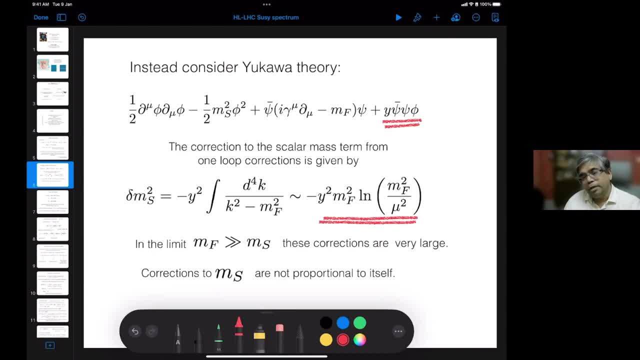 and if these fermions coupled to the Higgs and if they are sitting at gut scale or something. So these corrections are very, very, very large and this is problematic if you, especially systematically, you can show that in a granular theory, this happens because the Higgs comes from. 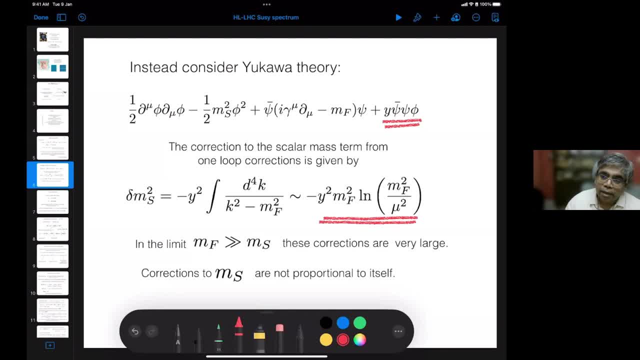 a higher multiplet and so on. so So it comes from a higher multiplet, there is a mixing between doublet and triplet and so on. so you can actually systematically show within a granular theory. this is a very, very large correction and of course you can argue it in various ways. actually, 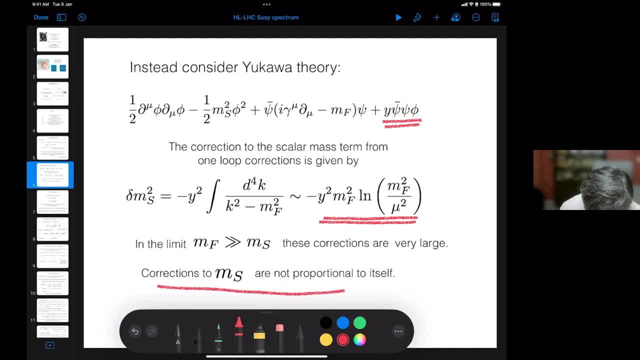 So this is the main point. So now if you, how do you get rid of this correction? You impose a symmetry, and this symmetry is nothing but a supersymmetric theory. So how does it get rid of it? You add a fermion for every fermion. you also add a scalar, so for, uh, so for every fermion. 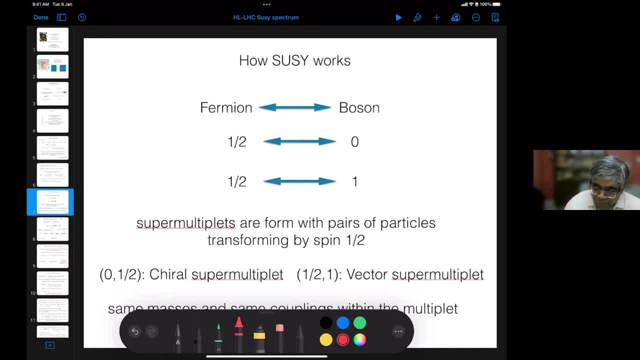 you add a scalar, and for every scalar you add a fermion in a way. okay, So, for example, we will stick to something technically called n is equal to 1 supersymmetry. For all phenomenological purposes, this is more than enough actually. 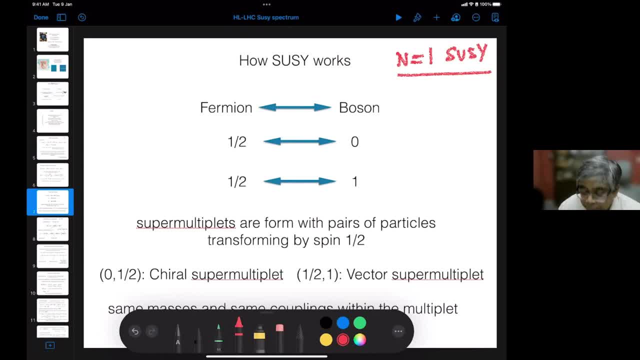 In this theory we consider two kinds of supersymmetric multiplets. Two kinds of supersymmetric multiplets For every fermion. for every fermion in the standard model, say, for example, you add a boson, And for every boson in the standard model you add a fermion. 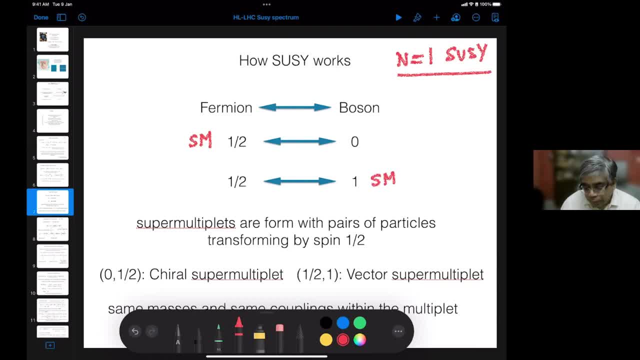 For every boson in the standard model you add a fermion, So supersymmetry is a theory in which it doesn't. So the basic idea is that if you interchange the spin of a particle by half, if you interchange the spin of the particle by half, 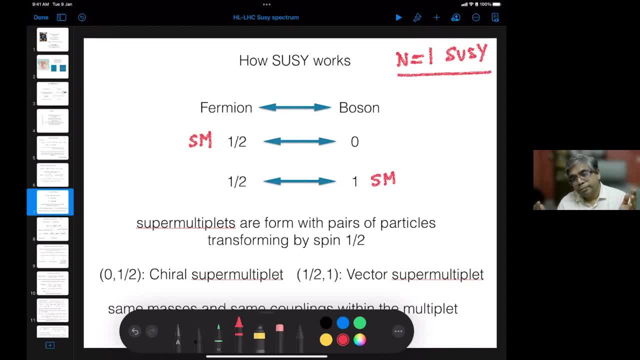 the Hamiltonian doesn't change, or the Lagrangian doesn't change, Okay, The Lagrangian should be equal, So the physics should be equal. That's the symmetry you're imposing. To impose that symmetry, so you take, you create multiplets. 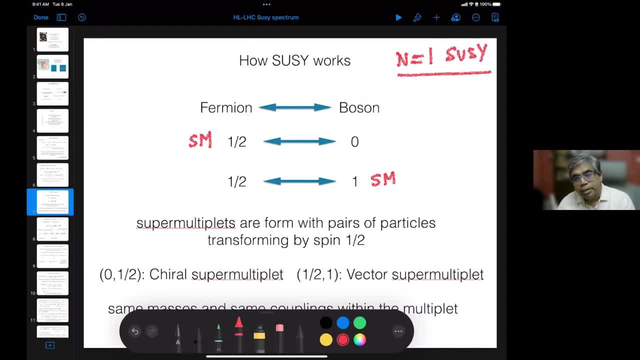 like what we are doing with SU2.. SU2, what we say is that if I change electron or an up-type quark with a down-type quark, if I interchange up-type with a down-type quark, the physics doesn't change. 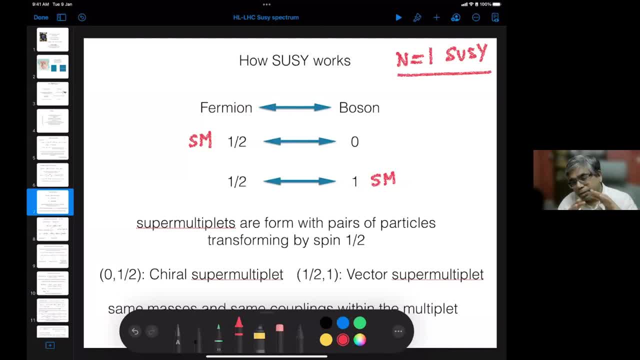 Of course, left-handed and up to certain details. It's not just interchange symmetry, but there are also, But the dominant symmetry is essentially the interchange, the sigma 1 and sigma 2 operators of the SU2.. But in this case what we are doing is the same thing. 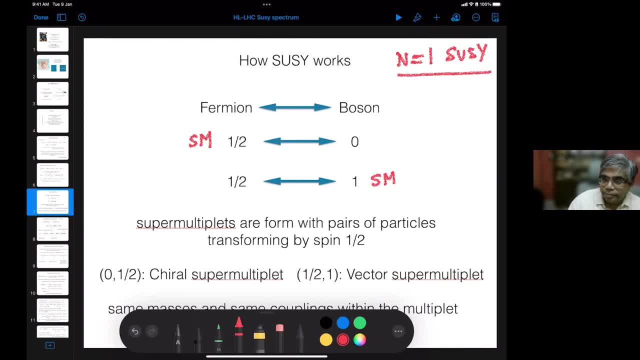 But instead of changing the isospin, what we are changing is the spin itself, the spin of the particle itself. Every spin half particle, if I change it with the equal boson actually, and then you have The symmetry should be invariant. 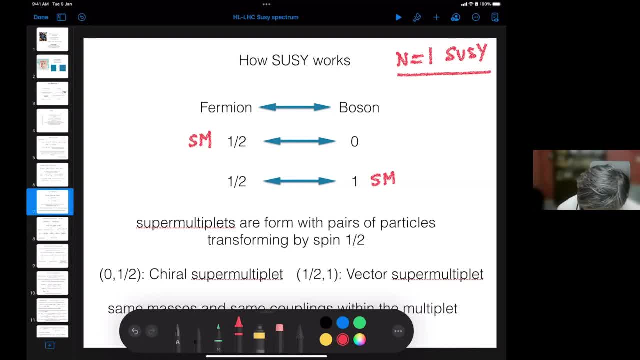 So what you do is you construct something called the multiplets. These multiplets are not, So there are two kinds of multiplets. One is called the chiral supermultiplet and the vector supermultiplet. The chiral supermultiplet is a combination of a spin 0 and a spin half particles. 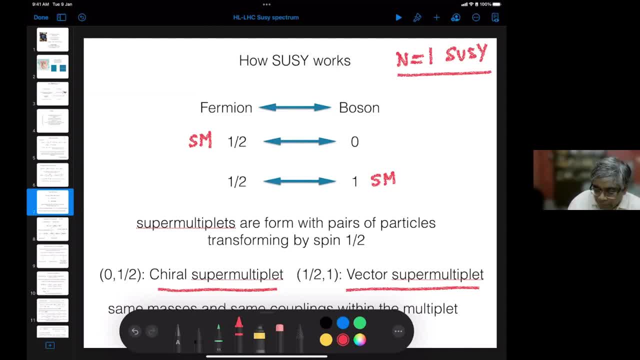 So that means a scalar and a formian, spin half, formian And the vector supermultiplet contains a spin half and a spin 1 matrix. Now what supersymmetry does, as we'll see, it makes sure that the particles within the multiplet. 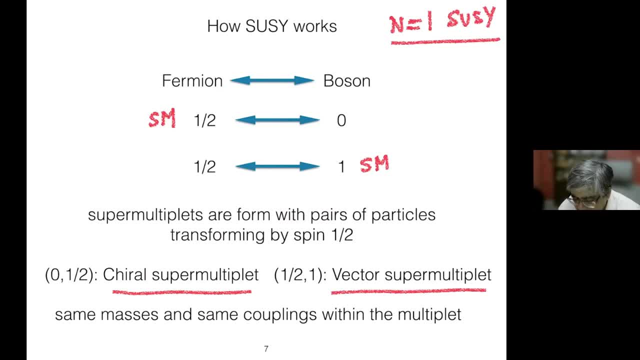 say the chiral multiplet, they have the same masses and the same couplings. So even if you put a gauge theory on something, the particles within that multiplet will also not just have the same masses but also have the same couplings. 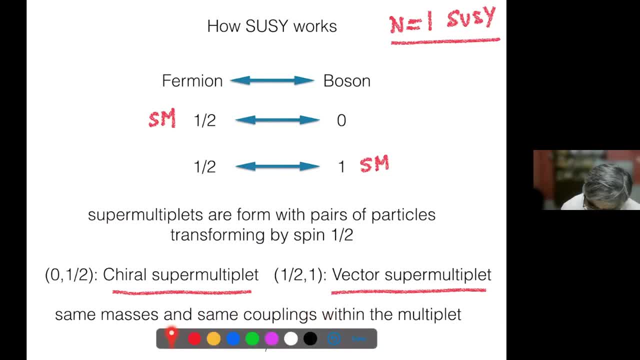 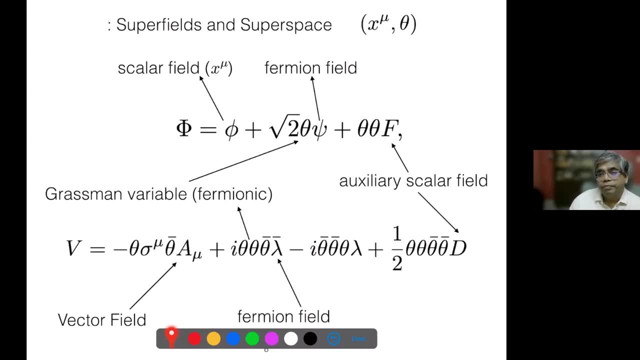 Okay, So they have the same couplings here, So these multiplets can be written in. if you want to connect it with field theory, you write them in terms of some sort of something called a super field. Okay, So these super fields have some space. 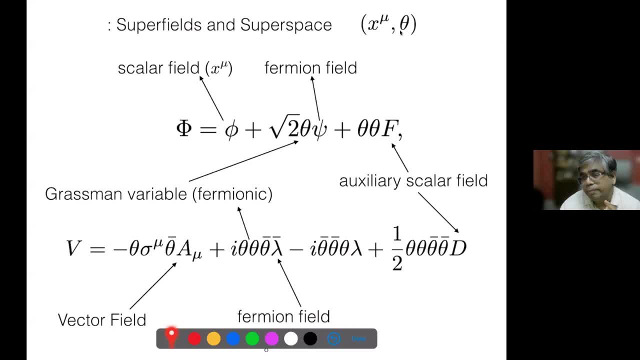 which is called the Grassmannian space, essentially, which is theta. Now, let's not worry about the great details, But anyway I'll just write down how I have written explicitly down What this super space contains, Super field contains. 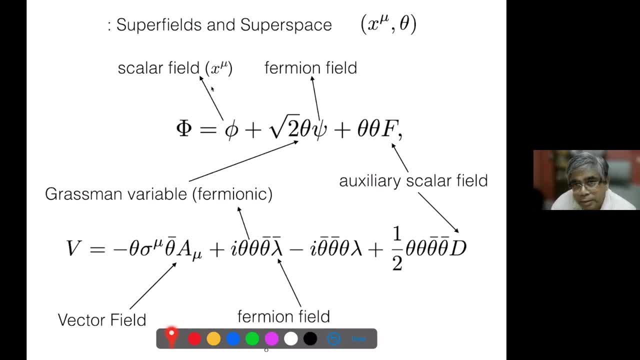 the chiral super field contains a scalar field which is spin 0 particle, a fermion's field, Psi. So this is important, Phi and Psi. And it also contains a spin 0 field called auxiliary scalar field. This is not a physical field. 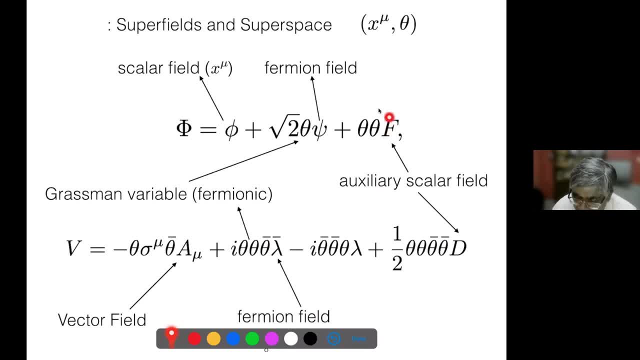 This field is not a physical field. Okay, The F field is not a physical field. So Phi is your scalar spin 0.. Psi is your spin half And F is spin 0, again, But this is not physical. Similarly, if you consider a vector multiplet, 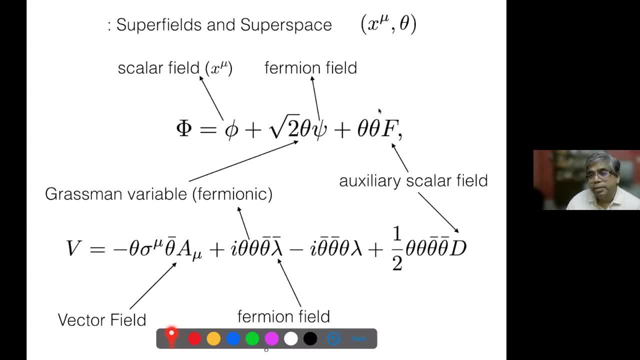 Vector multiplet means it contains the vector boson. Okay, Essentially. So. this is say, for example, a photon field. The photon field comes with a spin half particle- Okay, The spin half particle lambda, And it's conjugate. 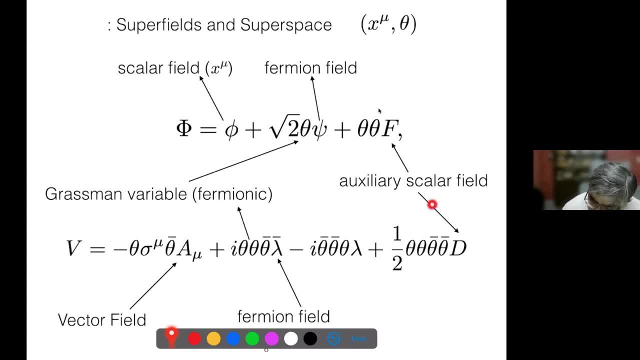 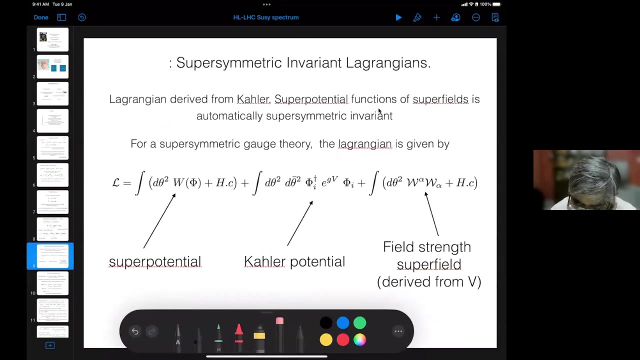 And then there is another auxiliary field, Auxiliary field. Auxiliary means it's non-physical Okay Field, which is called a, D. So these F and D terms play a crucial role in how supersymmetry is broken into two. So now let's 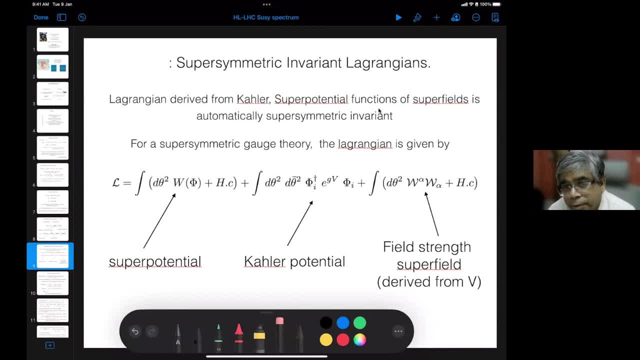 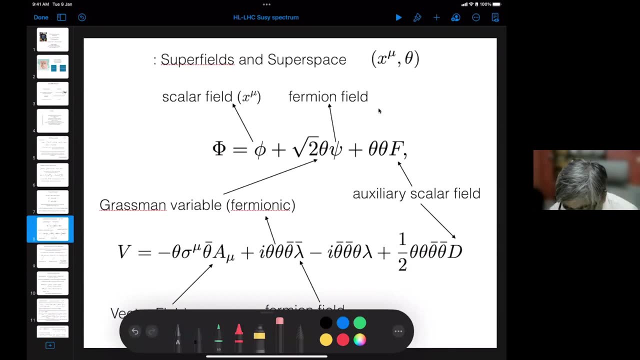 How do you write supersymmetric invariant Lagrangians? Supersymmetric invariant Lagrangians: you can write them very easily by considering three functions of superfields. So suppose you decided what your superfields are. Say, for example: you know what is the particle content of the theory you want to build. 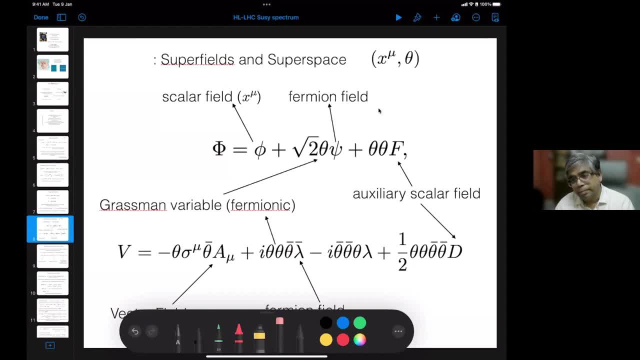 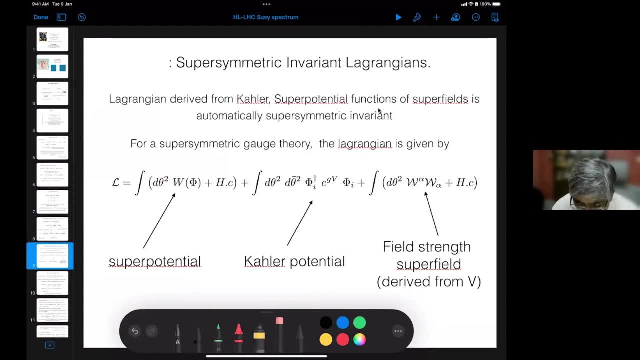 You want to build a theory with an electron and a photon. say for example, For an electron you consider a chiral superfield, For a photon you consider a vector superfield. And then to derive the Lagrangian, you have to write three particular functions. 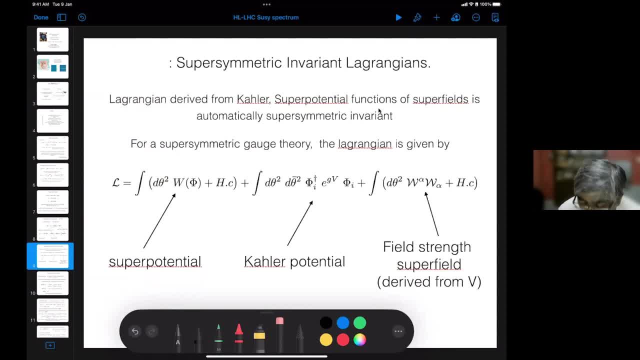 which are invariant and supersymmetric, And the gauge theory of the theory. If it's QD, you only look for U-N interactions. So the gauge interactions are conserved in a part of the potential, which is called the killer potential, Or which is part of the Lagrangian, which is called the killer Lagrangian. 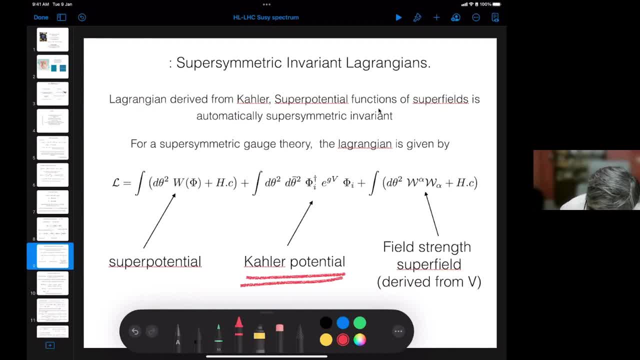 which sits like this: Okay, I'll come to the expansion. what the terms it gives you in a second actually, Then there is. Then there is something called the superpotential. The superpotential is an analytical function of the chiral superfields. 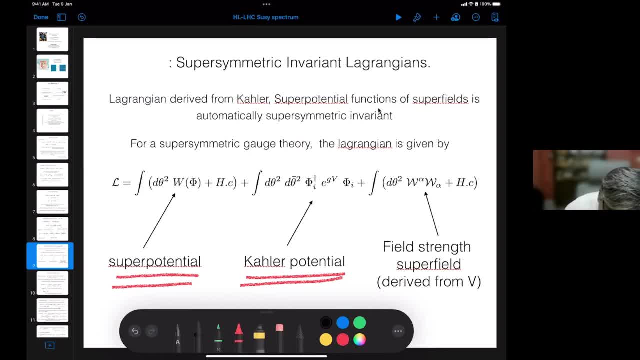 It doesn't contain any vector superfields, So this is just purely a function of phi, Whereas this one is a real function of the chiral superfields and also a vector superfield, So it contains both the chiral superfields, Okay. 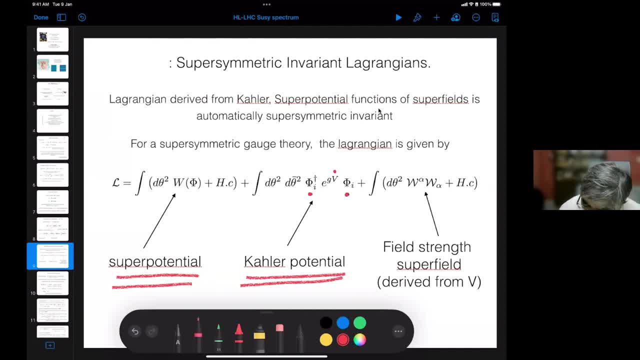 It contains both the chiral superfields and also the vector superfields here. And there is another thing which gives you the kinetic terms for the vectors. Say, for example: this is the F-mini, F-mini term in supersymmetric language. This is your F-mini, F-mini term, which is called the field strength superfield. 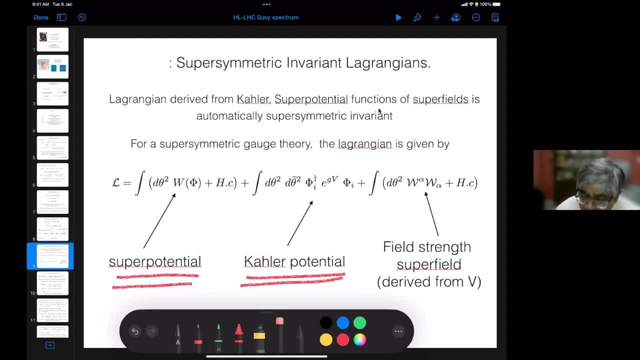 which only contains the vector superfield, meaning V, nothing else. Okay, So now let's go into these three functions. So, given these three functions, your Lagrangian is fixed. Okay, If you're given these three functions. so all you have to worry in supersymmetric theories is essentially okay. 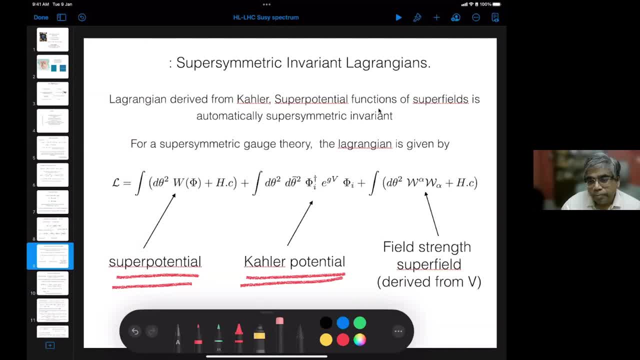 I know what my particle content is. Okay, What's my particle content? I'm going to write supersymmetric theory involving electrons or photons, or I'm going to involve some standard model plus with some extra scalar or extra photon. So you know your particle content. 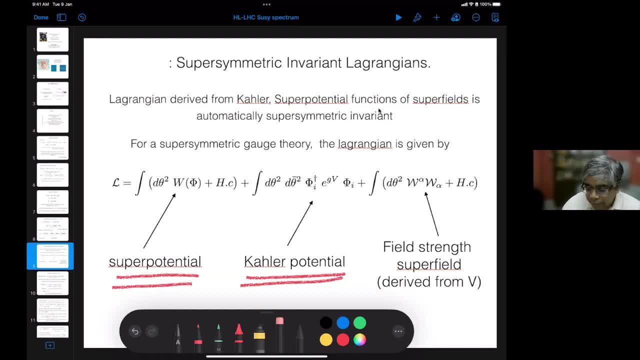 Once you know the particle content, you write down these three particular functions of superfields and derive the terms which you get and that gives you the entire Lagrangian. So your Lagrangian is completely fixed And these superpotentials- scalar potential and field strength- also have definite rules. 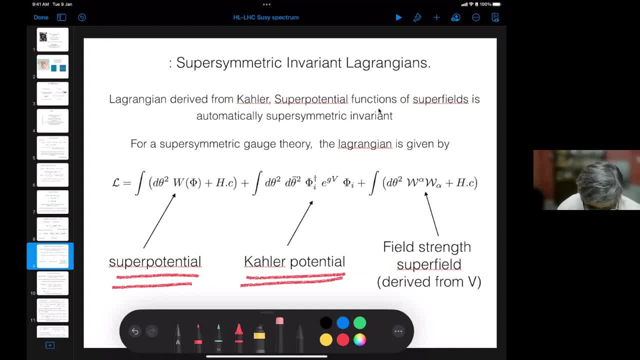 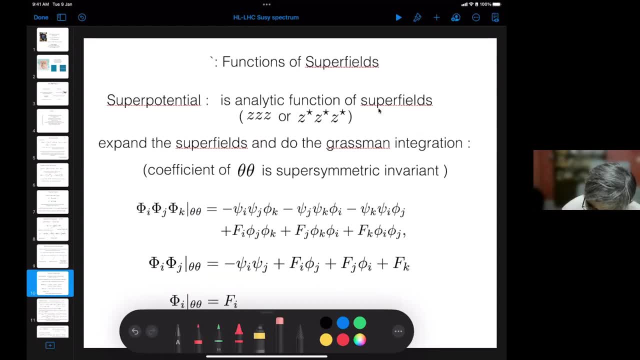 So these rules, if you follow them, you can derive them very easily. Say, for example, the superpotential is an analytical function but it's not a specific function of superfields. That means it just goes as 5,, 5,, 5, or 5 star, 5 star, 5 star, and so on and so forth. 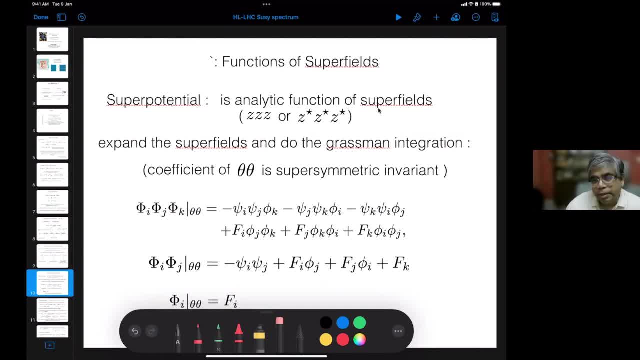 And if you do this full algebra, okay, the Grassmann integration and so on and so forth, you know what you'll get. Okay, So suppose, if there is a term, So you can write down a linear term or a bilinear term in superfields or a trilinear term in superfields. 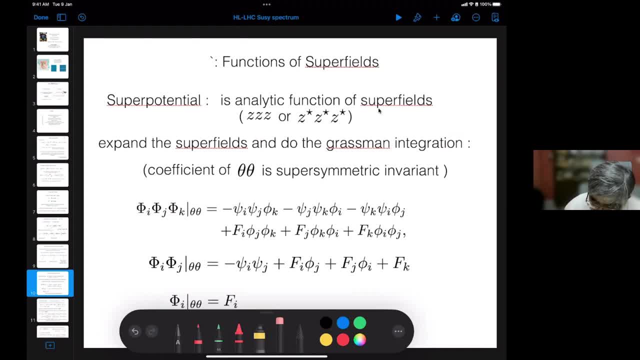 When you write it down, see what it gives you Automatically. you'll get it immediately. So if there is a bilinear term, let's start with a linear term. Linear term is not physical, but it gives you something. F term: 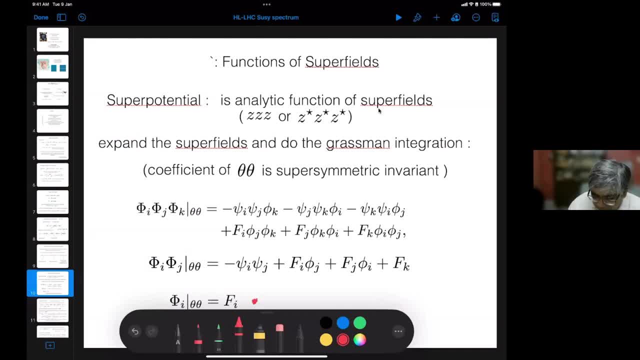 Okay, The linear term is F term. If you just add a single superfield in the superpotential, it just gives you F. If you add two superfields, it gives you just the fermionic coupling. So if you want, this is people familiar with. 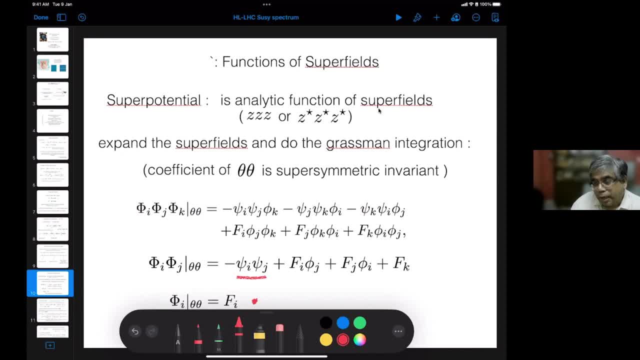 supersymmetric theories. I'm just making the connection. This is how you get the mu-term in supersymmetric theories. The supersymmetric, the mu-term. it contributes in scalar sector, but it essentially the one is the Higgs-Zeno mass term. 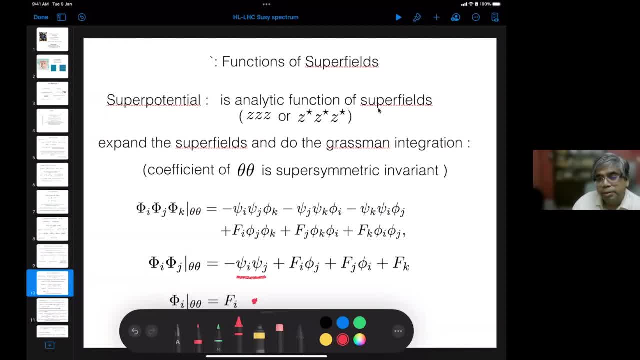 So this is how you get the mu-term in supersymmetric theories. Okay, So so if you have, say, for example, Marana masses for some Newton or any of these things which you, if you write it down, if you have a very linear mass term, 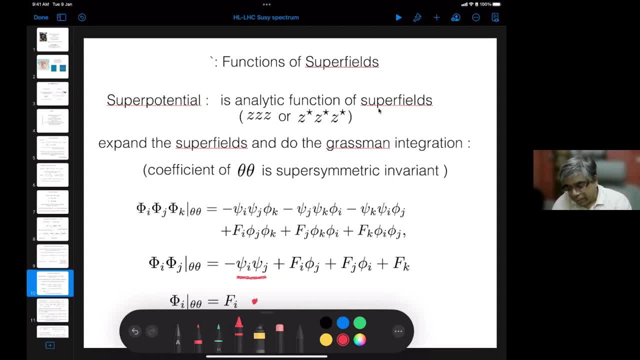 it only gives you fermion mass terms and some combinations of scalars. The most important thing is that a cubic term with three superfields, current superfields. what it gives you is Yukawa couplings. It gives you Yukawa couplings. 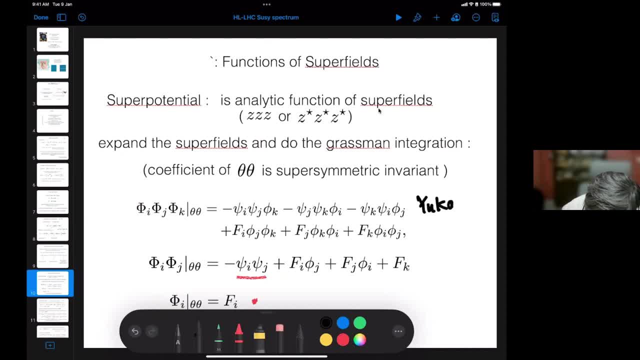 So it gives you Yukawa couplings. So essentially we know if you want to put supersymmetric standard model. the Yukawa couplings are, say for example, all the fermion masses, electron mass, muon mass, tau mass. 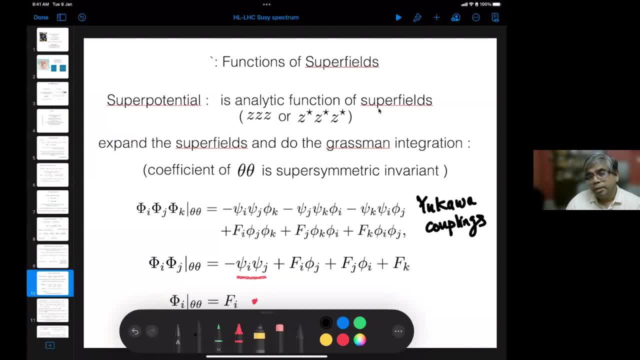 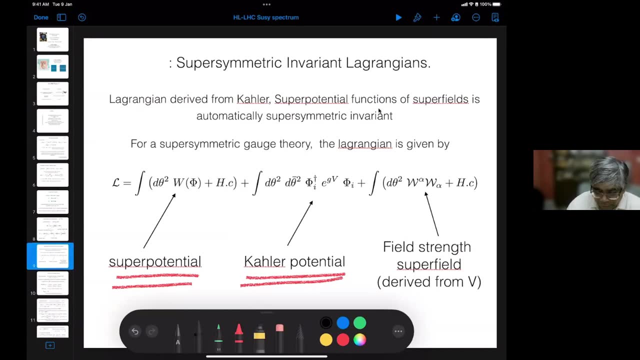 These things should come from the superpotential. So the superpotential should give you this function. The superpotential function will give you essentially the Yukawa couplings, But this is not the only thing, because there is also Hc sitting here. So Yukawa and Yukawa Hermitian formulae will be given from the superpotential terms. 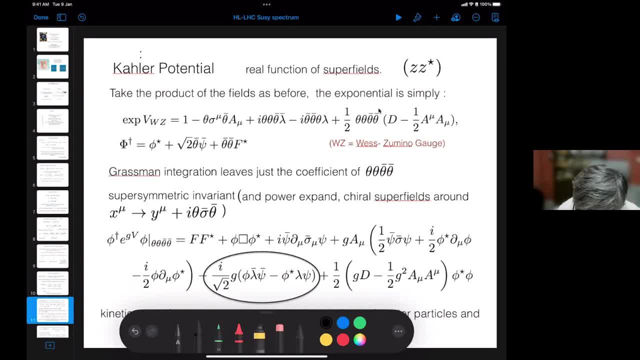 So what about the Keller potential? The Keller potential is a real function of superfields Z and Z star. So if you expand the exponential containing the vector superfield, you can do the full analysis and you can do the Grassmann integration. And the Grassmann integration just leaves the coefficient with theta, theta, theta bar, theta bar. 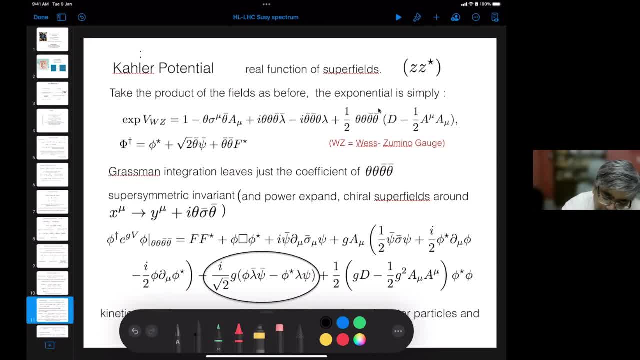 I didn't tell what these thetas are. These are just Grassmann variables. These are Grassmann variables which you have done when you have fermionic curve, If you did path integrals with fermions or if you did quantization of fermionic piece. 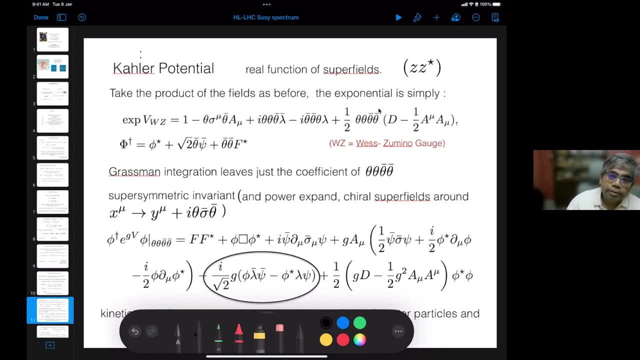 you are familiar with Grassmann variables essentially, So even if you don't know, it doesn't matter. All we need is to know the final formula. Even if you don't know what these Grassmann variables are, they are exactly like fermionic piece. 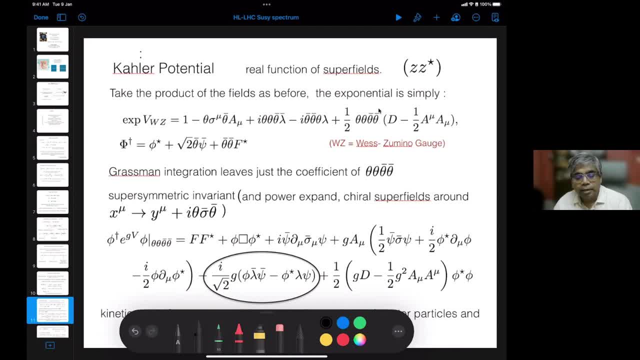 So they have to commute with each other and they act like spin-half particles essentially. So they are not particles, of course, They are just some variables, like h, mu and so on. So you are introducing spin variables- if you want quote, unquote spin variables- along with the spacetime. 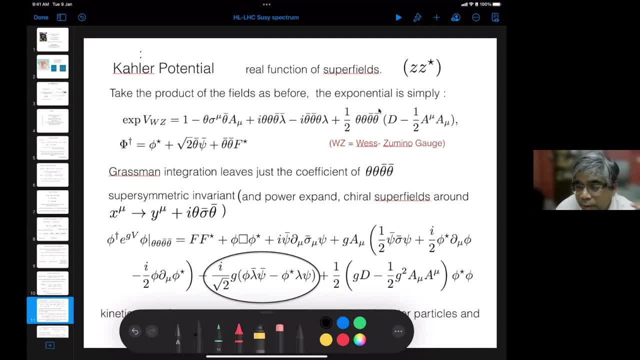 So you want to build it as a super space because, remember, supersymmetry changes the spin of the particle. So what you do is, when you do this expansion of the Keller potential, what you finally get is all the kinetic terms. Let's say, for example, the kinetic terms for the scalar. 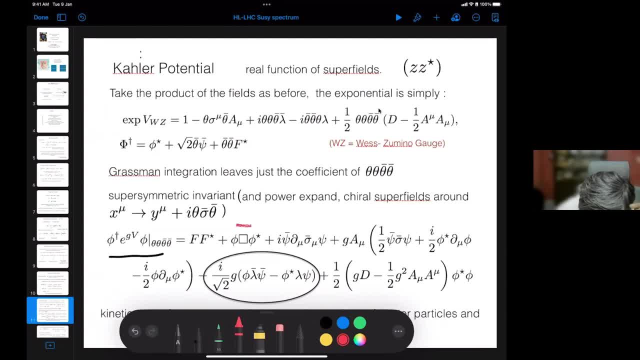 kinetic terms for the scalar, kinetic terms for the fermion, and then, exactly like what happens when we do an ordinary field theory, along with the kinetic terms you also have the gauge interaction terms. This is like your gauge interaction terms with the scalar fermion. 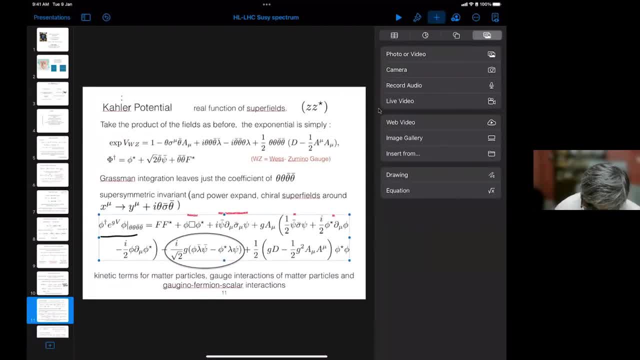 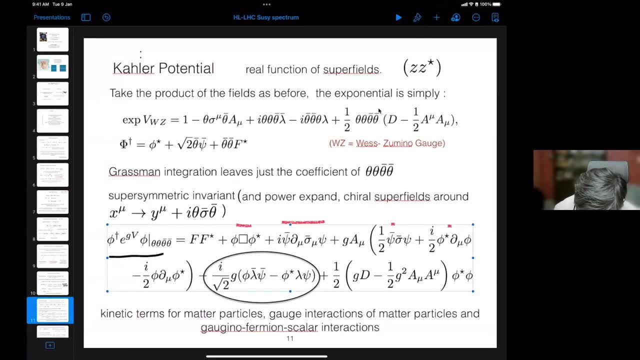 gauge interaction terms with the fermion of the scalar. Okay, how do I go through this? Okay, gauge interaction terms with the, but the self-interactions, whatever meaning? the quote unquote. this is the gauge interactions of the scalar. 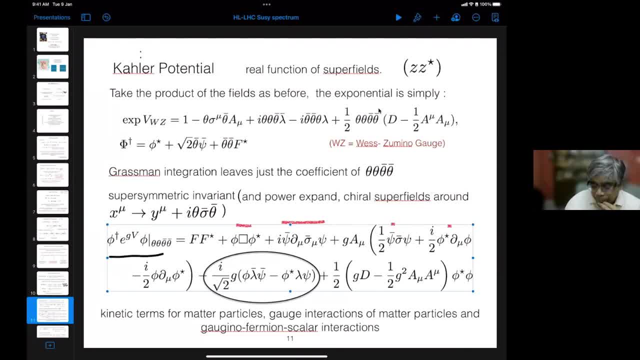 But in addition. in addition, the most important point which distinguishes ordinary field theory with supersymmetric field theory is that you get gauge interactions which are like Yukawa interactions. Okay, So in addition, they come in the kinetic potential, So they come with the kinetic terms. 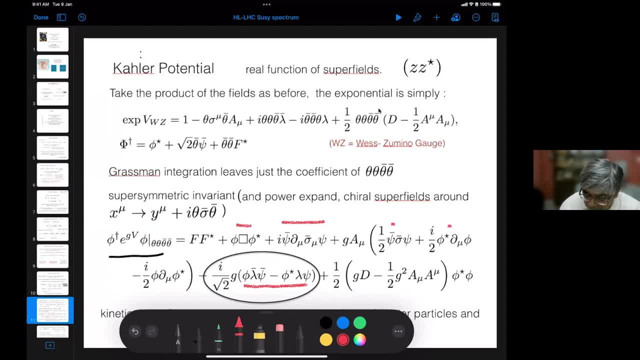 So they come with the Keller potential, So you get Yukawa-like interactions, but they're proportional to gauge, So I'll express this in more detail in a second. actually, So lambda is the spin half partner of a mu. Okay. 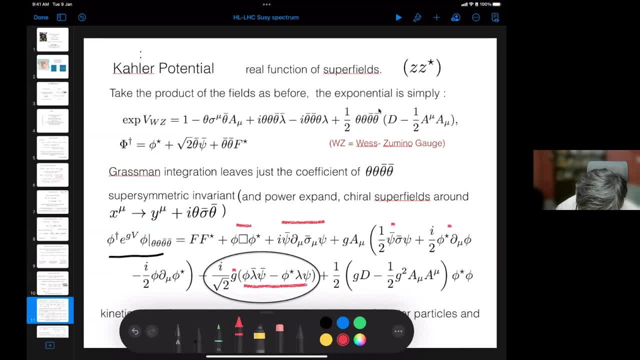 And phi is a supersymmetric partner of psi. Okay, So between the three lower spins, spin zero spin halves, two spin halves- you can write a sort of what do you call a Yukawa-like interaction. But this is a gauge interaction, because the lambda 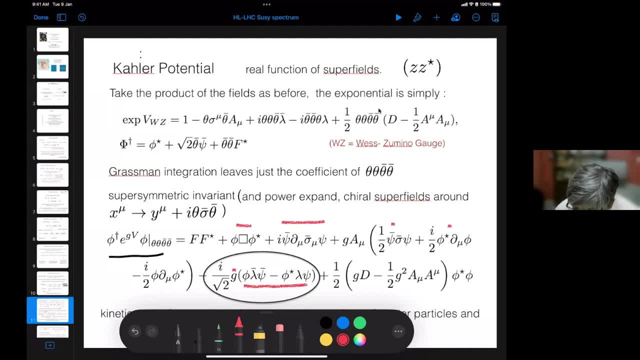 the lambda is a gauge partner, super partner of the a mu field. It's a gauge super partner of the a mu field because a mu and lambda form a super field, vector super field. Okay So, the vector super field and in interaction with current super fields, 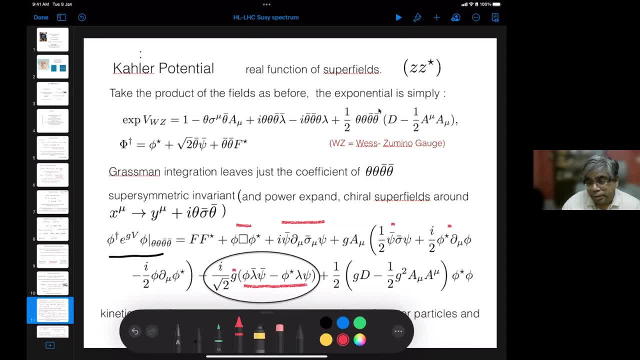 also generates gauge-like Yukawa couplings, gauge-like Yukawa couplings. So there's it: generates Yukawa couplings, but their strength is proportional to the gauge interaction. Their strength is proportional to the gauge interaction. So then, finally, the third function. 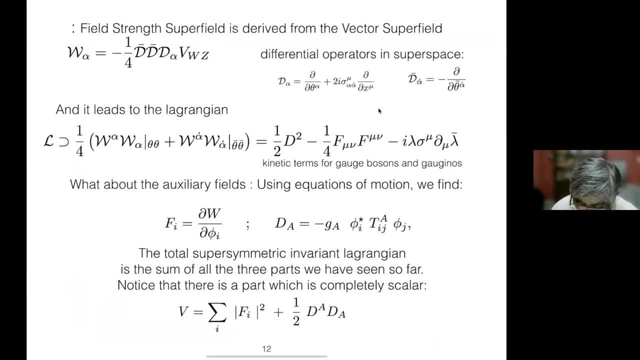 which is the field strength super field. it is derived from the vector super field. Okay, It's derived from the vector super field by some derivative terms. These are supersymmetric differential operators of superspace And this gives you, as I said, 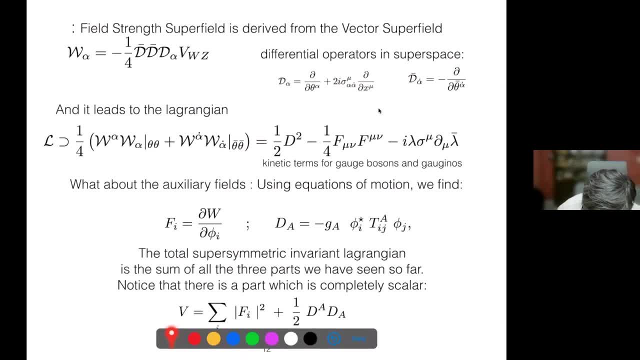 the kinetic terms not only for the a mu field but also for the lambda field. So the lambda is essentially so. this is the only term which doesn't have, didn't have a gauge interaction so far. many kinetic terms so far. 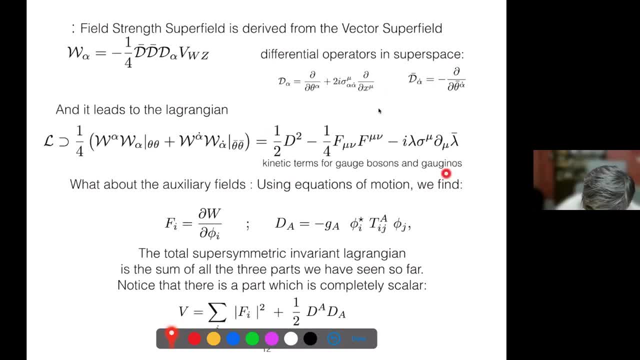 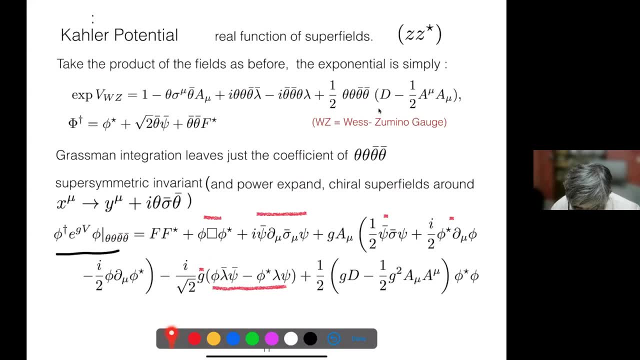 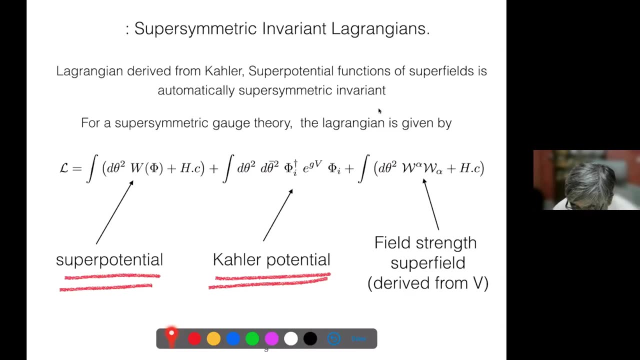 So the kinetic terms for the gauge multiplet and its super partner come from WR. So just to summarize, what we have is essentially the super potential, which gives you Yukawa-like couplings, ordinary Yukawa-like couplings, like doing the matter particles. 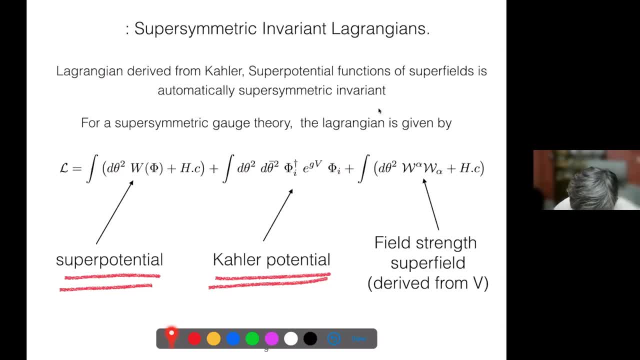 Okay, Without no gauge interactions. if you write Yukawa couplings, you write them in the super potential, You get them from super potential. So okay, And the Kähler potential gives you kinetic terms for all the all the particles in the super multiplets. 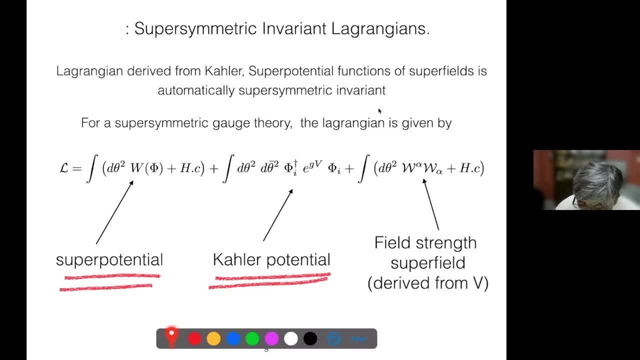 except for the gauge particles, All the matter particles. it gives you the kinetic terms and also the gauge interactions of this of these particles, And the gauge interactions with the gauge genome or the supersymmetric partner of the gauge particle also come from the Kähler potential. 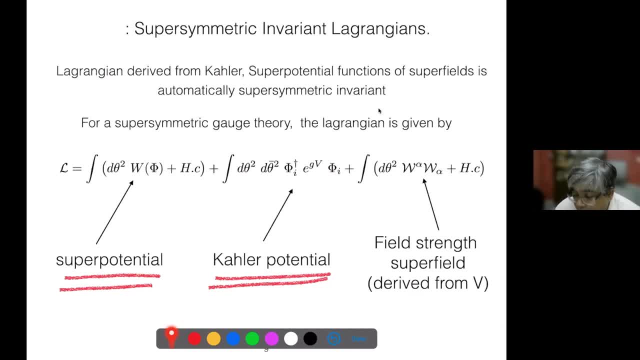 And they look like Yukawa couplings. They look like Yukawa couplings but they are proportional to G. And finally, the last term is essentially the kinetic terms for the gauge sector. Okay, So the kinetic terms for the gauge sector. 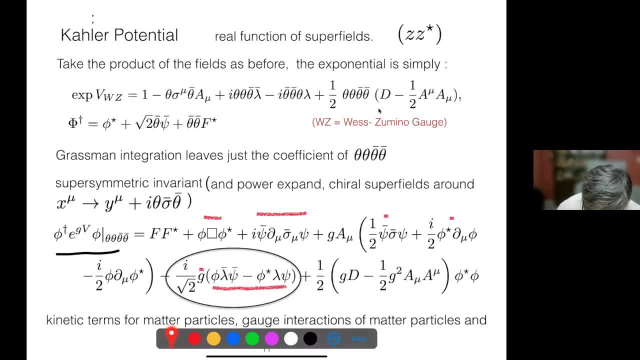 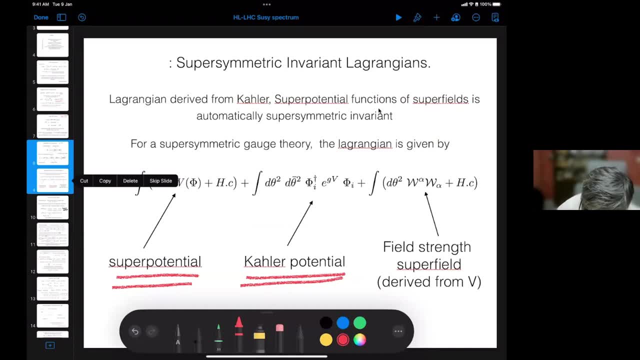 so each function has its own duty. One second, So each function has its own duty. so this is kinetic terms, terms, Oh sorry. This is kinetic terms for EMU vector field lambda. This is kinetic terms for all the matter. multiplet, which is essentially 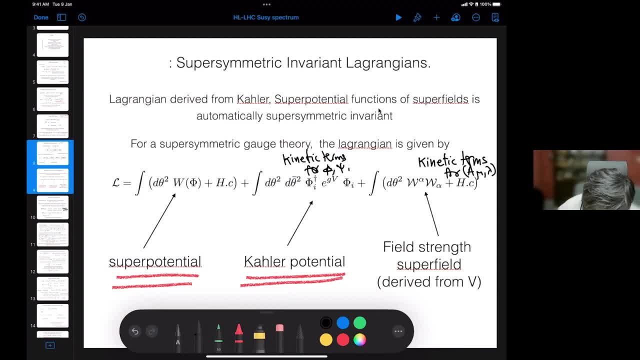 phi and psi and also the gauge interactions And within the gauge interactions we have Yukawa-like interactions with the gauge inner. The gauge inner interactions appear like Yukawa interactions and this just gives you Yukawa couplings, Non-gauge interactions, or this is non-gauge interactions. 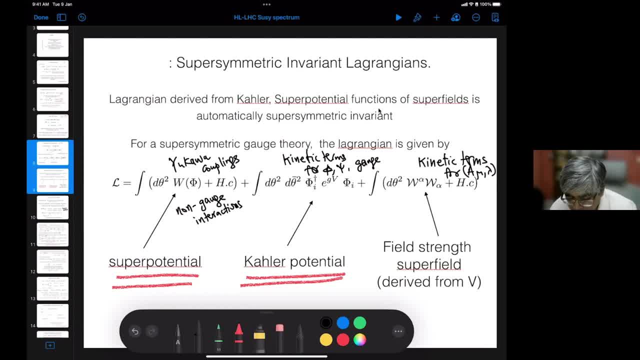 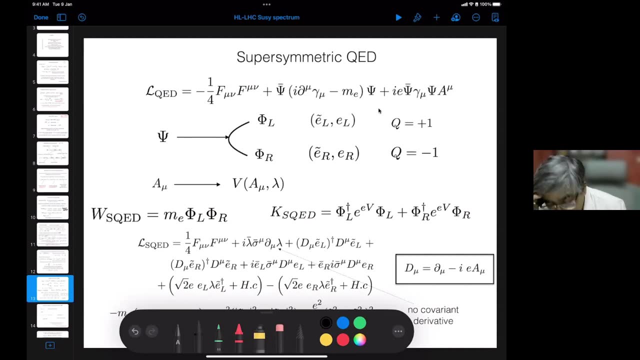 So if you can distinguish what are gauge interactions and non-gauge interactions, you know what each function gives you in the supersimple theory. Okay, so let's just do an example so that we understand this better before moving to MSS. Any questions so far? 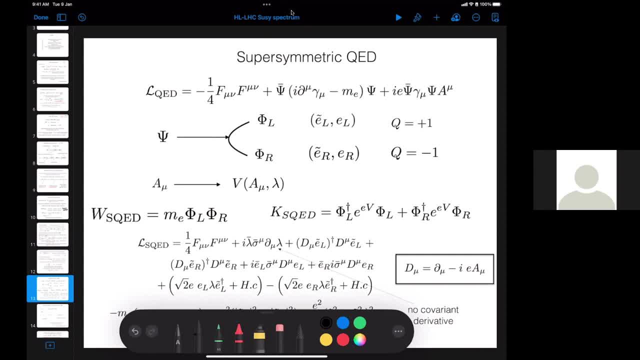 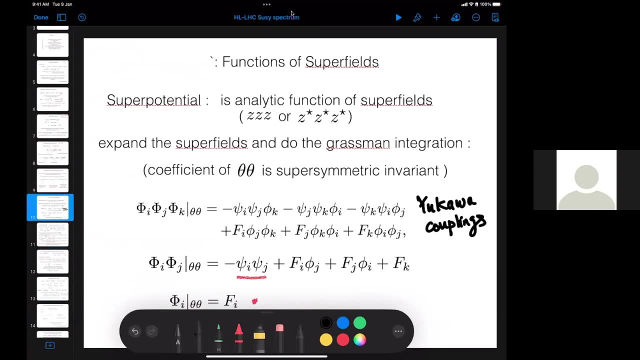 I see one in chat box. Okay, What is g Alpna? you can speak up please. So on this slide, I think the previous question- there is an exponential factor with z in it, So indica potential, yeah, in this one. 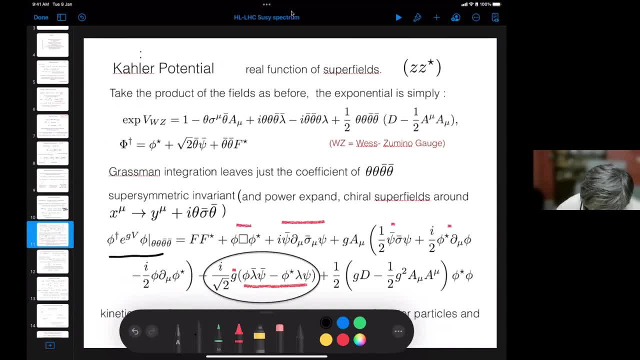 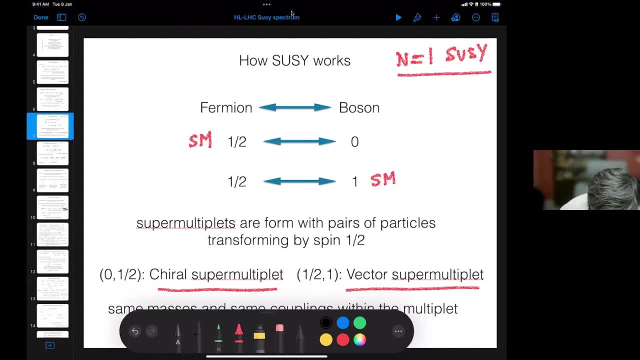 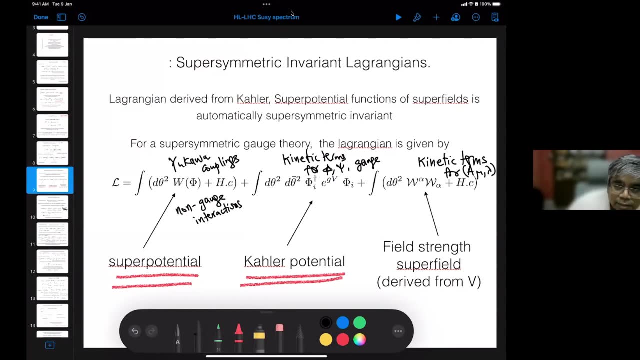 So on slide 11.. Yeah, g is just the gauge coupling. Okay, The small g you're asking right, Pardon, I'm sorry. Yes, yes, This g. Yeah, yes, That g is just the gauge coupling. So if you have more than one gauge, 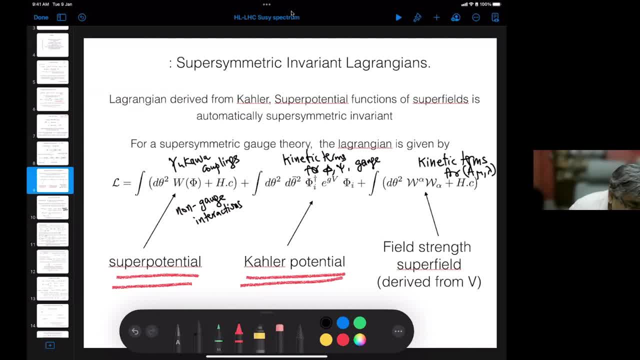 coupling. you just sum over all the g's and their corresponding v terms. Okay, g for, say for example u1, g for su2, g for. So there are three different g's, right, So each one will come with. 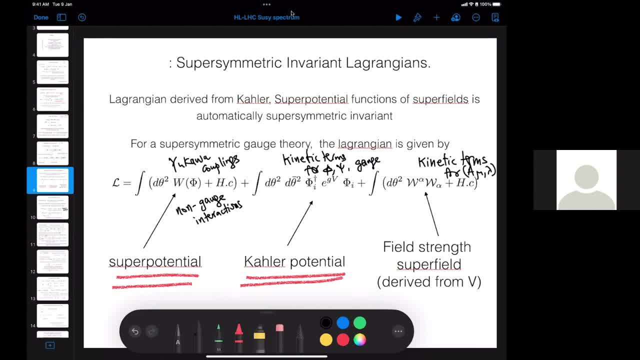 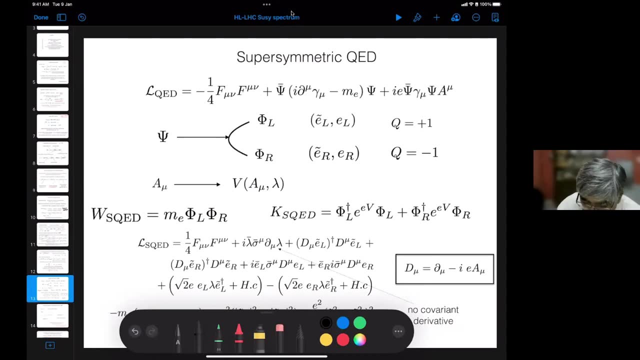 their own v? Okay, so their own gauge vector, super multiplicator: Yeah, Okay, thank you. Okay, so now I have the supersimple theory theory. Sima, you have some questions? No, I had a quick one. Yeah, go ahead. 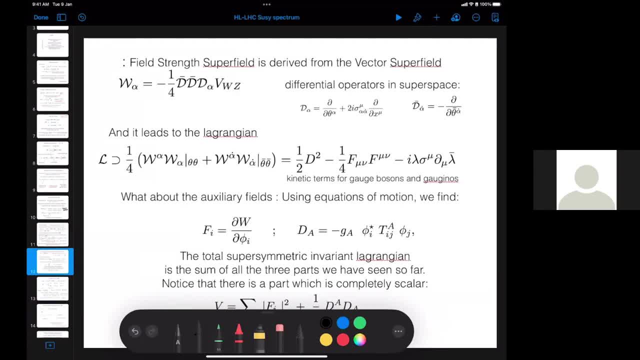 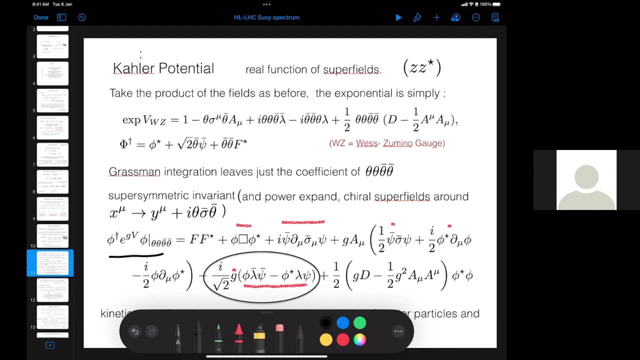 So, on the previous slide, Yeah, Previous to this one, Previous to this one, The one which we're just discussing- Yeah, So you mentioned the no, the one which, yeah, so this one only. So you mentioned that some of these are the gauge interactions also. Yeah, So you mentioned that some of these are the. 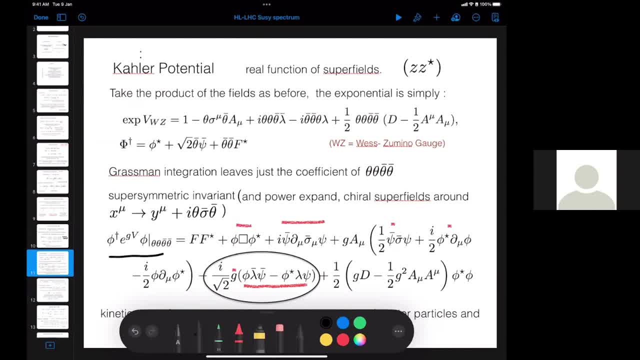 gauge interactions also. Yeah, So you mentioned that some of these are the gauge interactions also, While the others are for the, the terms which you are writing. See, the point is that the Kähler potential gives you only gauge interactions, so their form is like個- expressions, because the gauge, you know. 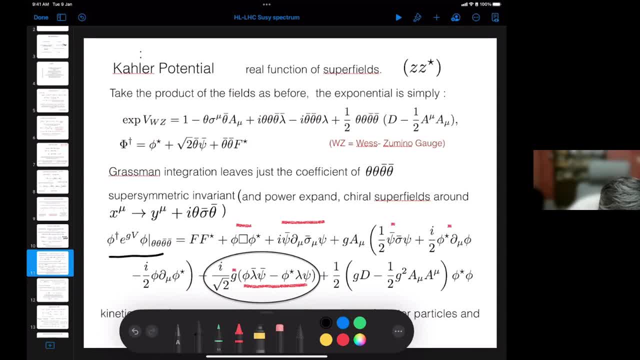 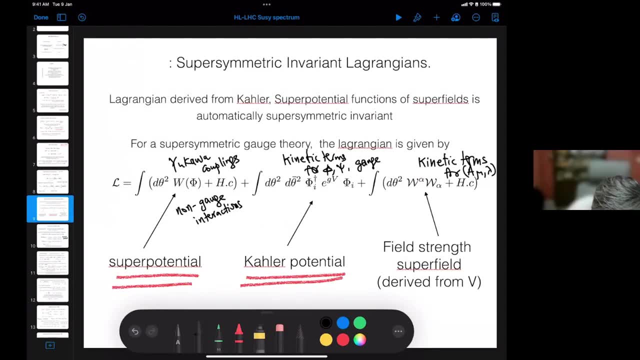 No, no, I think it was the same slide which Awakuna was asking the questions, So it was the same, where you have written the two terms: This one, Oh, okay, So this one you are talking about that the scalar potential is only giving the kinetic. 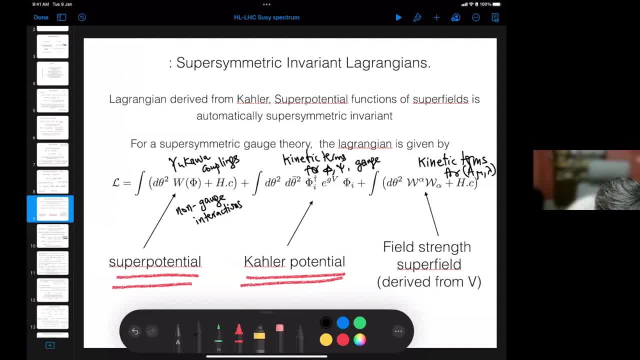 terms for the phi, psi and the gauge inverse or gauge interactions. No, no, no, only at gauge interaction. yes, Okay, and the letter one is for the gauge inverse and all Yeah, the kinetic terms for the gauge inverse and the gauge boson. 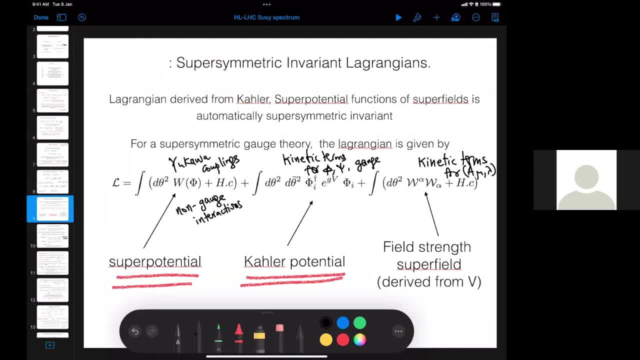 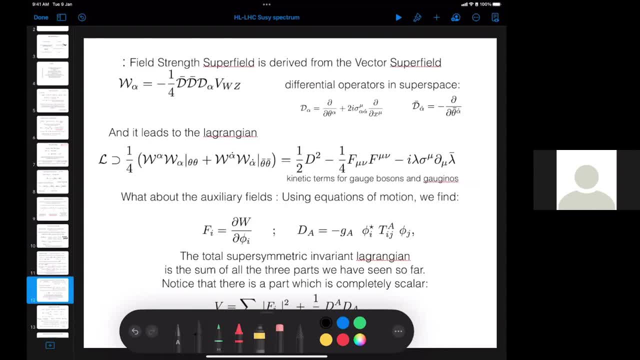 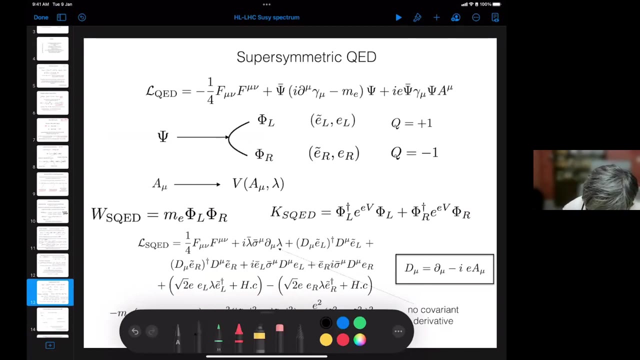 Okay, okay, that's fine. No, I'm confused with the gauge interactions and the gauge inverse, what you said. Thanks, Right, right, yeah, Okay, so, yeah, so, let's, this is your ordinary QED, So let's start with the. let's try to supersymmetrize the QED. 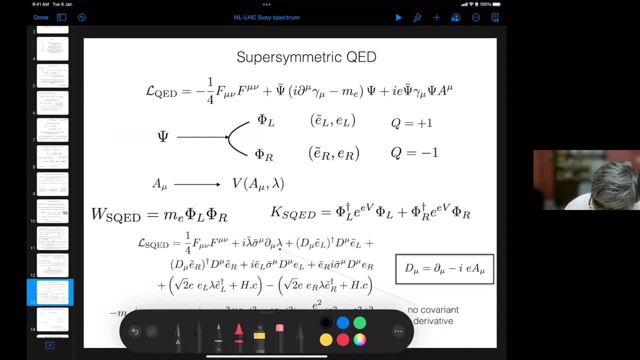 This is the Lagrangian which I think most of us have spent a lot of time on it, more than the standard model, I think. I don't know if you are a student, I think Okay, so if you are a student, you would have spent more time with this. 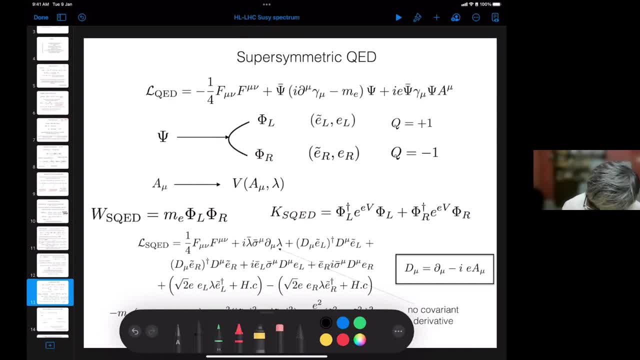 This Lagrangian compared to any other Lagrangian, Say, for example, the QED Lagrangian. So this is your ordinary Dirac Lagrangian. and then you have the Fminu Fminu and this is the interaction term. 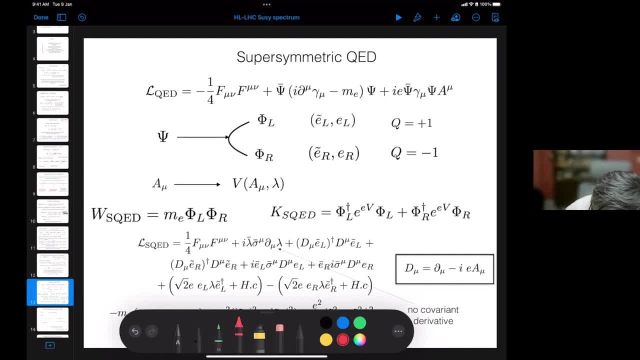 This is the interaction term. So this is your interaction term. So what I have here is a photon field and then a psi field, which is for the electron field. So what I had to do is This is the description. as I mentioned to you that electron has two components. 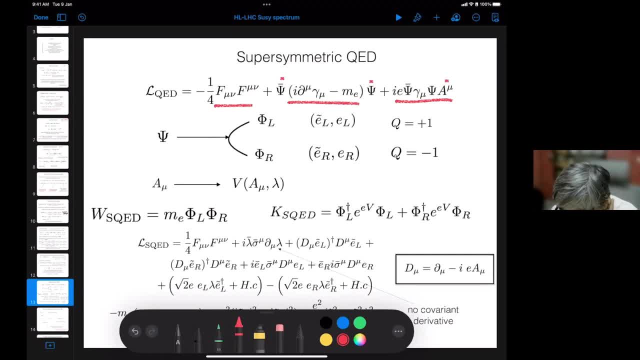 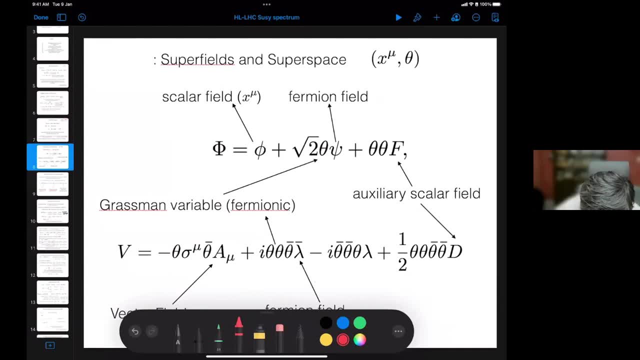 Okay. by the way, I should mention that, whatever I have done so far, chiral- the term chiral here- this is a two-component field. That means it is either psi L or psi R. This is a two-component field only. 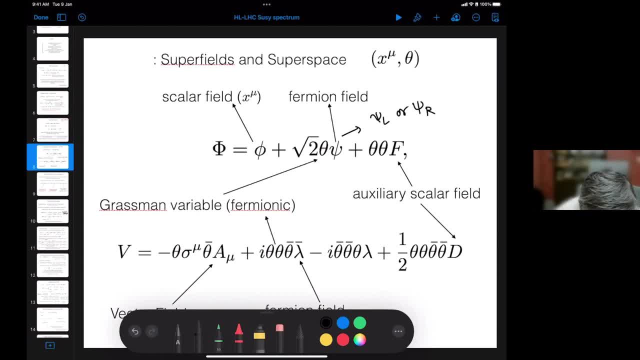 So every two-component field you have to add one super field. So for every left-handed projection or right-handed projection, you have to add one super field. Okay, so the super field is a chiral super field, so it at least has two components. 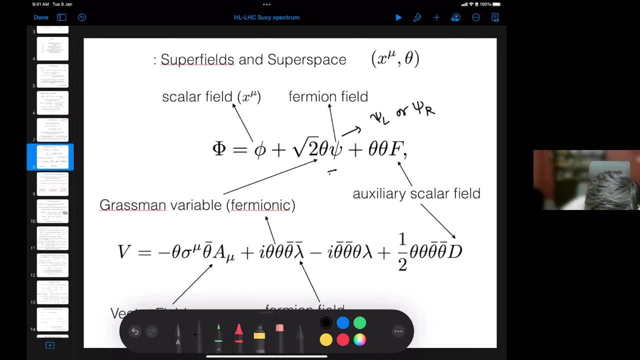 This is not a four-component Dirac spinor. This is not a Dirac spinor, This is just a two-component spinor, whether it could be in the chiral representation this could be just psi L or psi R. So remember your gamma matrices for the chiral representation and then you are the Dirac. 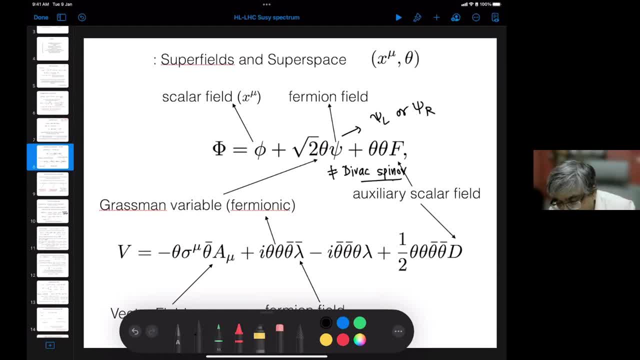 spinor And then do the projection for 1 plus gamma 5,, 1 minus gamma 5, and take the chiral projections And for each chiral projection you have to write a separate Dirac spinor. The reason is the degrees of freedom are really two. 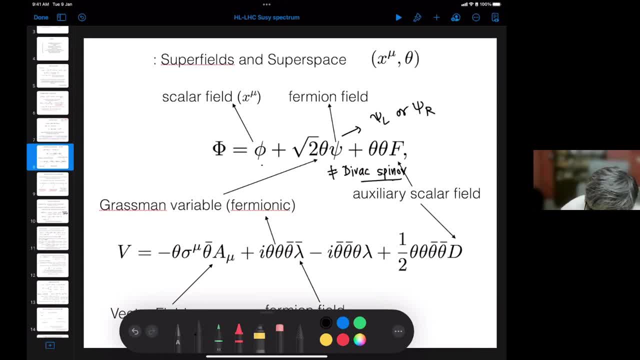 So this has really complex. So phi is a complex scalar field. It has two degrees of freedom. So psi has only two degrees of freedom. You can only add two degrees of freedom here If you add a full Dirac spinor. If you add a full Dirac spinor here, you end up having four degrees of freedom. 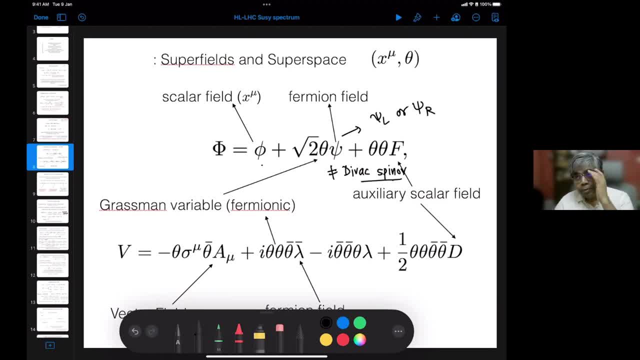 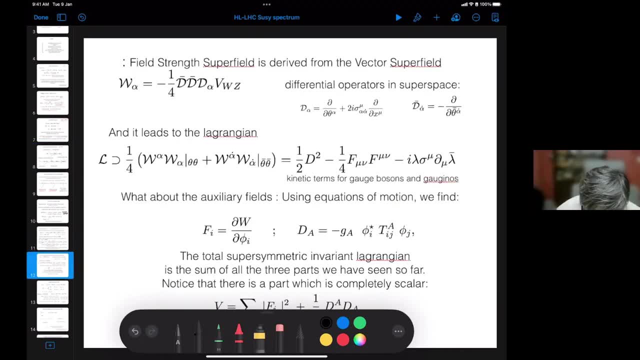 So this is not allowed. So you lose two degrees of freedom. So that's the reason why you only add chiral projections. Professor Rimpati, there is a question? Yeah, I think the two browns should. Can you go ahead and ask the question? 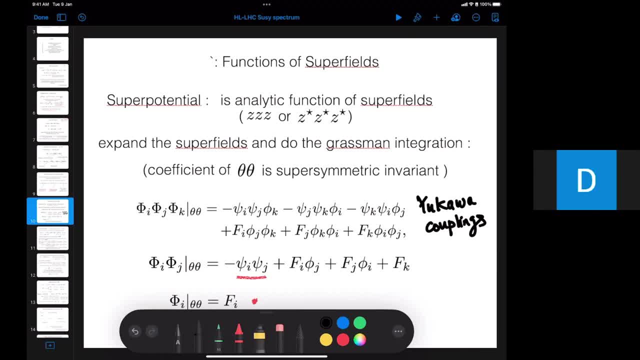 So it's not a question. So the thing is that, because of the colored palette which Sadi is using, the bottom portion of the slide is getting hidden. So I'm not, So, I'm not, So. I'm not able to see the content which is written there. 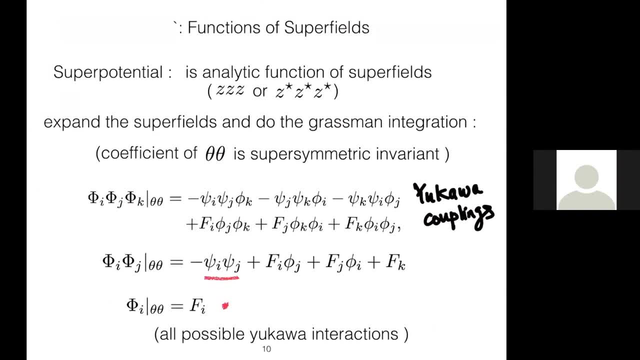 Yeah, So you just remove that. Yeah, Yeah, Now it's better. Thanks, But the point is, if I do that, I cannot write. Also, there is a question from Lekhika Malhotra Psi, as well as spinor. can you consider? 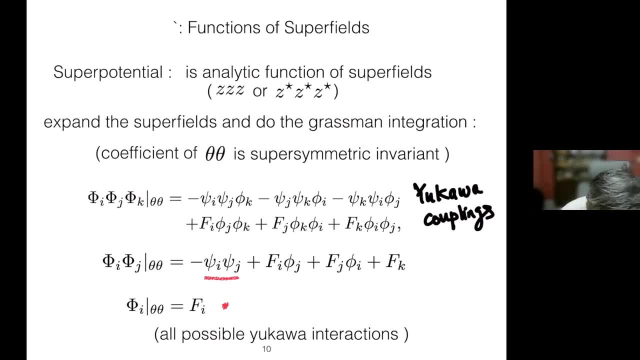 That's the question. Yeah, Yeah, In the mass. Okay, You can. You should consider it as a wild spinner. Hello, Who has asked this question? That's actually a correct question, actually. Yeah, So, Lekhika, do you want to go ahead? 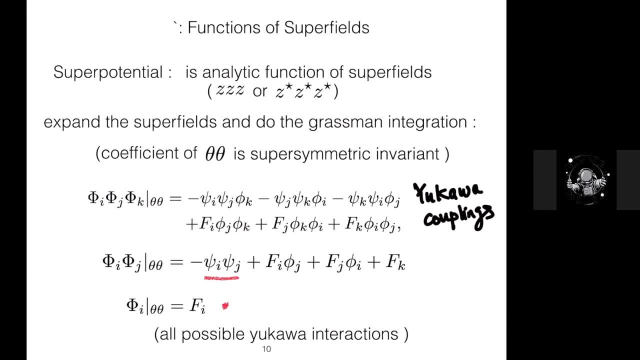 Yeah, I was just wanting to confirm that. Can we consider it as a wild spinner, Because you have just mentioned that it is not a Dirac spinner? It is not a Dirac spinner. Yeah, So it is a wild spinner. It is a wild spinner. 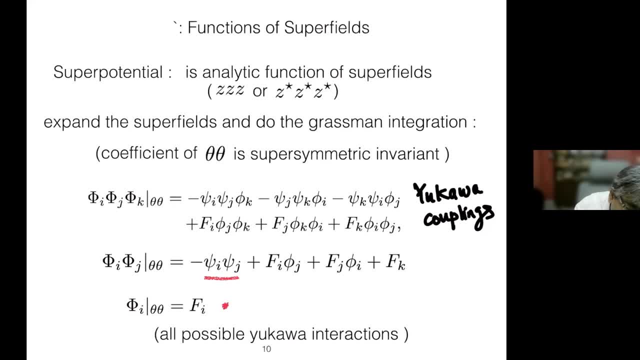 Because in the massless limit- Okay, In the massless limit, you cannot distinguish a chiral spinner with a wild spinner. Okay, Thank you. Yeah, So wild spinners are In the massless limit. they are exactly the same. 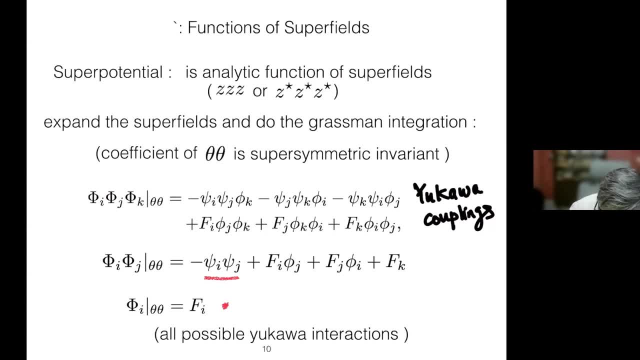 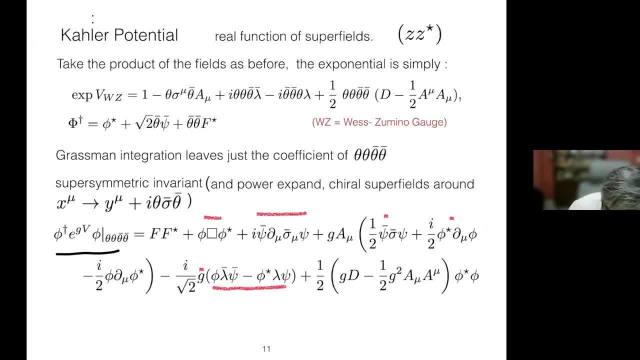 So you consider them as wild spinners essentially. So if you write in the massless limit, you end up having wild spinners and all these things. Why it's not a Dirac spinner? as I mentioned? because Dirac spinner has four degrees of freedom. 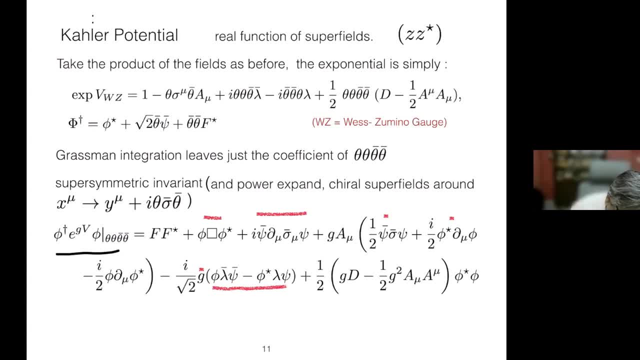 Whereas the wild spinner or any chiral. I wanted to explain why the word chiral. That's the reason why I said chiral spinner, But anyway, we should strictly considering wild spinners. They only have two degrees of freedom, Okay. 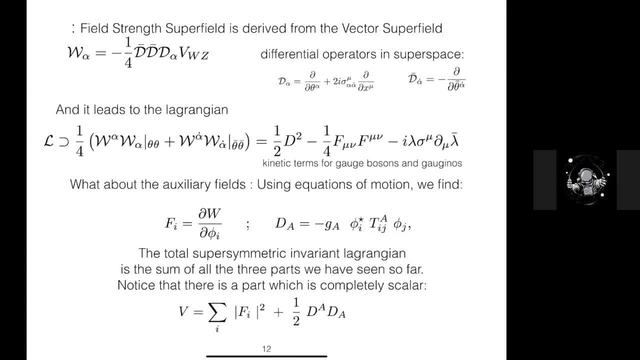 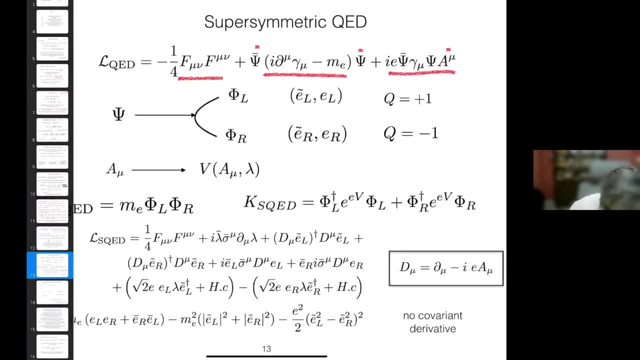 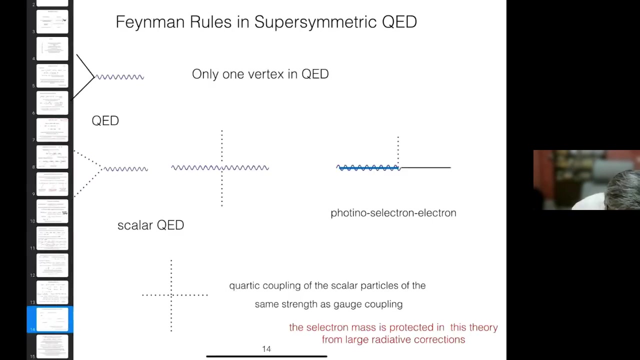 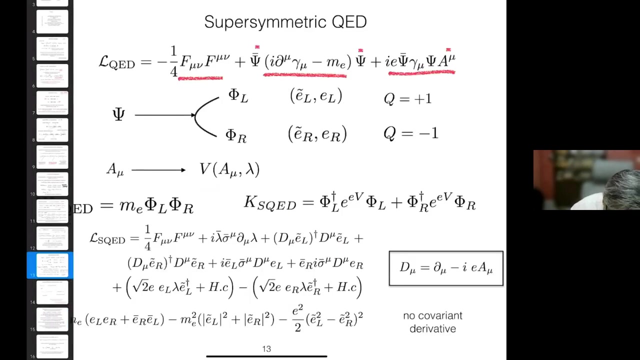 Yeah, Okay, Now I'm here, Sorry, Sorry. So let's Now, in this case, in the QD, psi is a Dirac spinner. I'm sorry, This is the problem with this one If I don't full write the full thing. 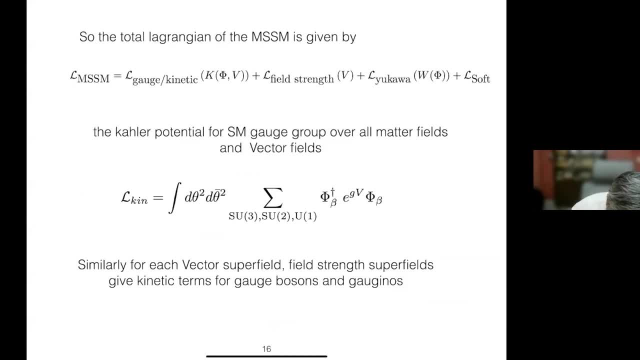 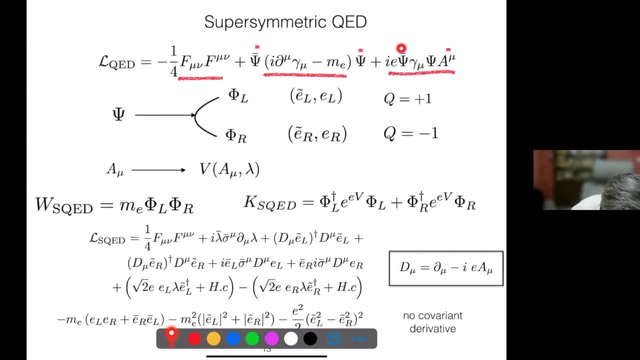 Oh God, I I'm unable to get, I'm sorry. Yes, Okay, Psi is a Dirac spinner, It comes. So psi is a Dirac spinner, So it has four degrees of freedom in QED And mu has two degrees of freedom. 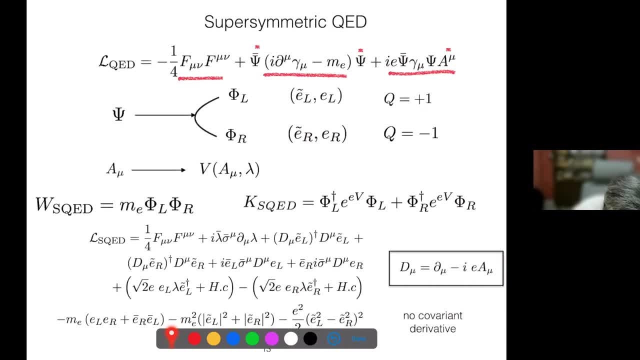 It's a photon, This is a photon field. So, psi, I can recompose it into two parts as phi L and phi R, One for the left-handed projection, one for the right-handed projection. And I chose, I chose, I chose different spin, different signs for that. 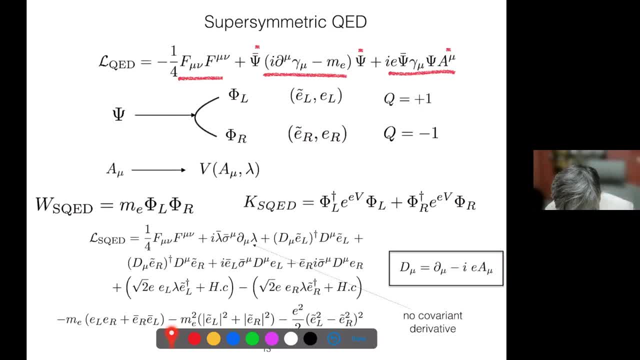 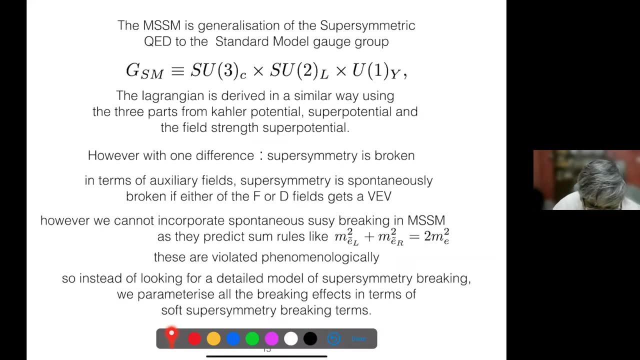 The reason is, there is a reason for this. It's not exactly. This is not exactly ER. It's something called the charge conjugate of the ER. Okay, There is. Okay, I'm having issues. It's jumping faster than what I can. 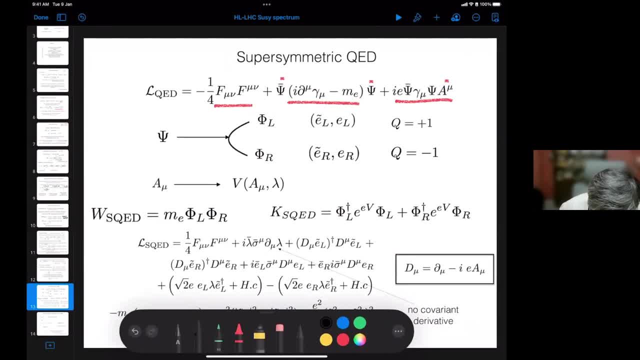 See, remember I told you that W is always By supersymmetry. it's supposed to be, It's supposed to be Meaning, it's supposed to be something analytic. Analytic means it is a function of complex numbers, but it's only a real function of. 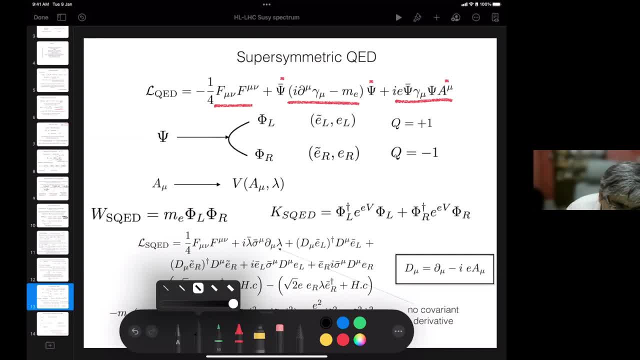 Meaning complex. It is analytic, means it's something like 5, 5, 5.. It doesn't contain any real part. Essentially, it doesn't contain some 5, 5 star. So, for this reason, what you do is you construct a chiral supersymmetric. 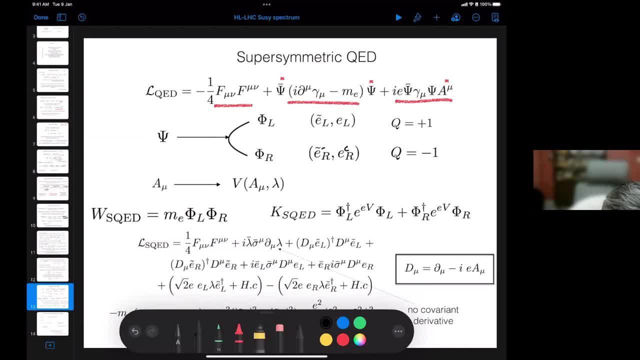 Chiral superfield with the conjugate. The conjugate, This is C ERC. So that means you do a charge conjugation of the right-handed field. Okay, You do a charge conjugation of the right-handed field. and take ER, star 5.. 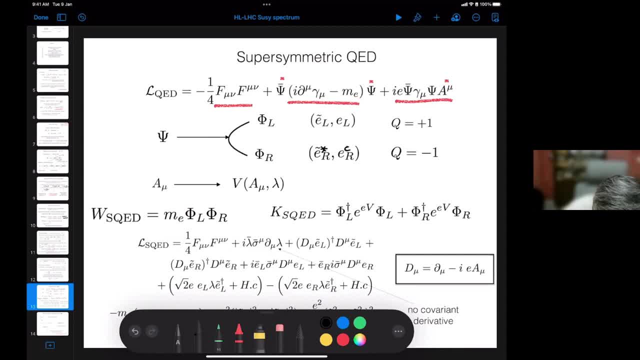 Okay, ER star And say that ER star is equal to. I wrote it as ER because this is ER star is equivalent to The scalar of phi, Phi R as the scalar of the phi. So I do such a thing so that I can work with. 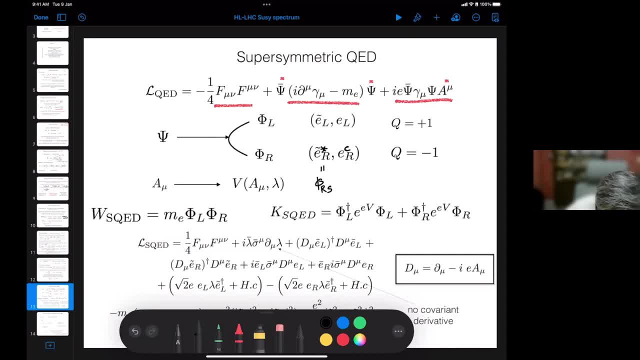 I can work with just phi L and phi R in my superpotential, If you want. Meaning, if you're. The basic idea is that I cannot write Terms like phi dagger or something in my mass term. Okay, Let me just explain it to you in a second. 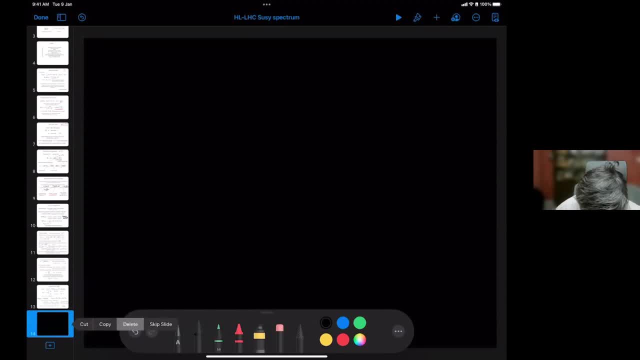 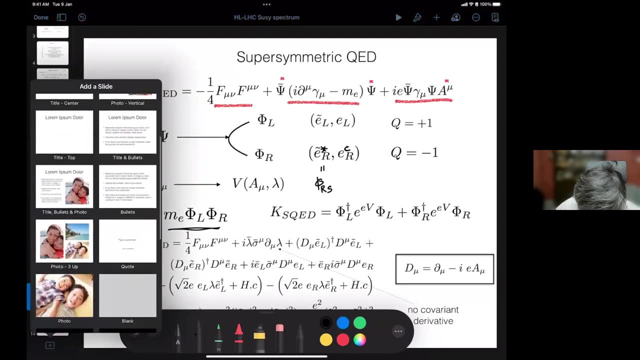 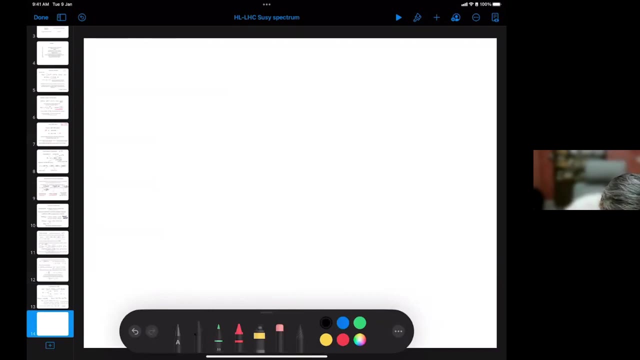 Oh no, What is this? I'll just write it down here. See, the basic idea is that in your Dirac theory, if you write a mass term, you write it as Dirac QED. Okay, You write a mass term as psi, L, bar, psi, R plus hc. 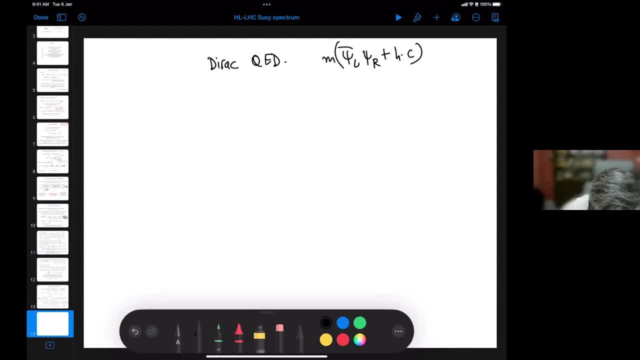 Okay, Or you just write it as m, psi, bar psi. Now bars are not allowed because in the superpotential I cannot write any bar term. So the way I write it down is: I take psi, R, is c or charge, conjugation of that. 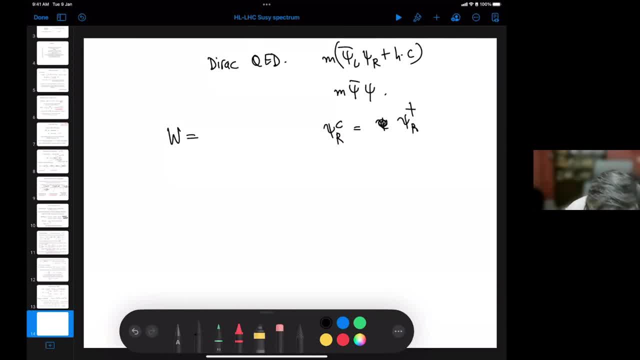 So that means psi R dagger. Okay, Some gamma two and everything will be there. Okay, So I gamma two or something. Okay, I sigma two, psi R star to be more accurate. This I call it as some other super field. Okay. 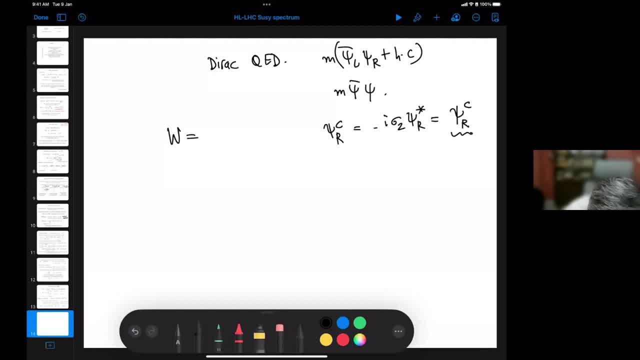 Psi, C, R. Okay, This I can take it to be real, I can call it as real. So the star of something is real. of another wave function. Okay, Another complex number. It's like calling Z: star is equivalent to some Z prime. 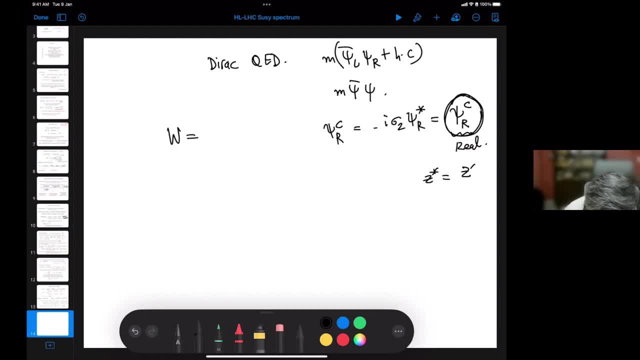 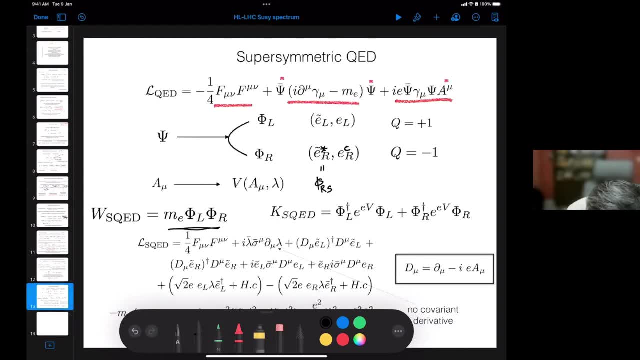 Okay, I can complex conjugate it and call it some other complex number. That's precisely what I'm doing here. Okay, So I take Er, Er, C and then I write down. I add two chiral super fields: phi, L and phi. 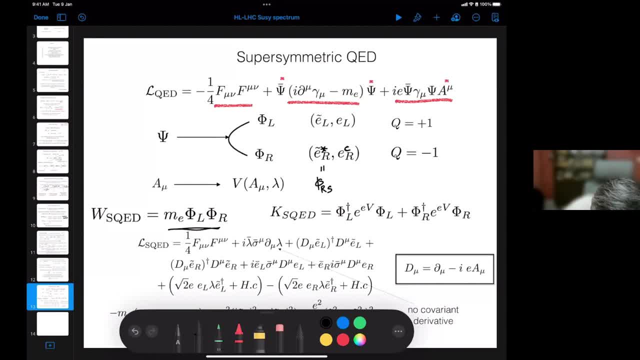 R And for the amu, the photon field. This is the photon field, This is the electron field. For the photon field, I just write down amu and lambda, which is essentially the spin one particle, And along with the spin one I add something called a fortino. 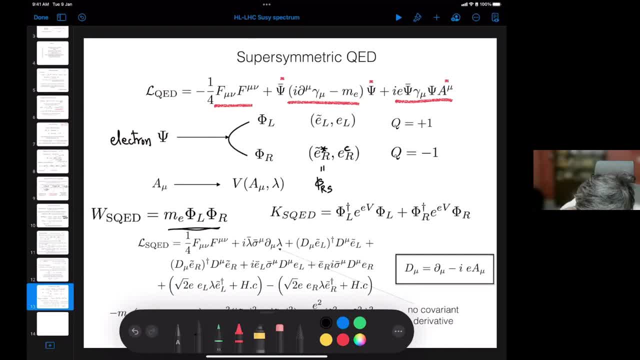 The gauge, you know, is called a fortino. Now, with this I have to write down my three functions. The theory is even invariant. The theory is even invariant. So the three functions, I can write it down. The first function is W, the supersymmetric QD, W, which contains just five, the only term. 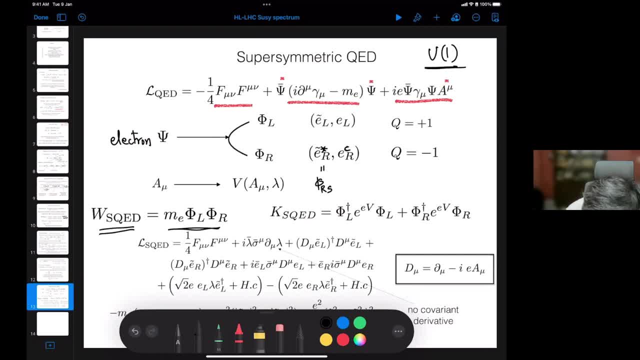 which is allowed, because this has a plus one charge. this has a minus one charge, minus one purely because I have complex conjugated them. Okay, Because I have complex conjugated them, they carry an opposite charge, And so this is the only thing which is allowed by the U-N symmetry: phi L, phi R. 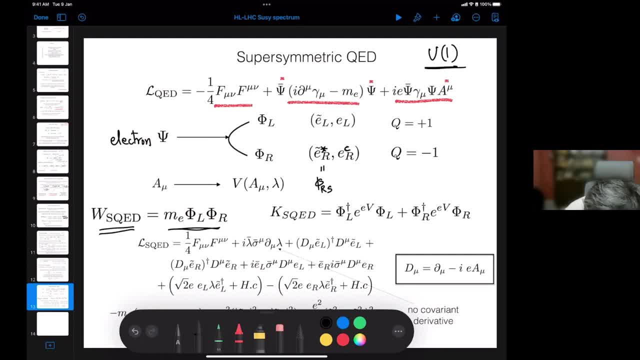 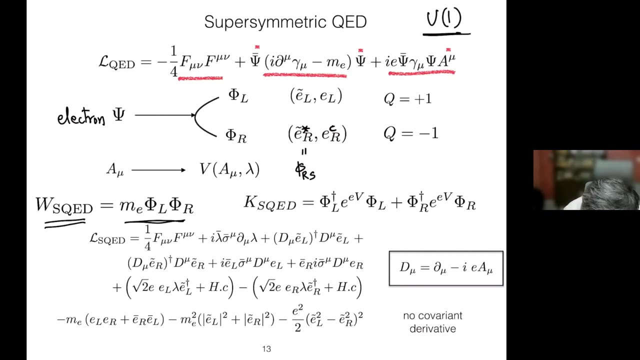 Okay, Okay, This gives you the mass term of the electron, And so that is gives me me, Then, the kinetic terms for each of these super fields: phi L dagger E V, phi R dagger E V. Okay, Phi L dagger E V and phi R dagger E V, plus the W, plus the W. The third function is the. 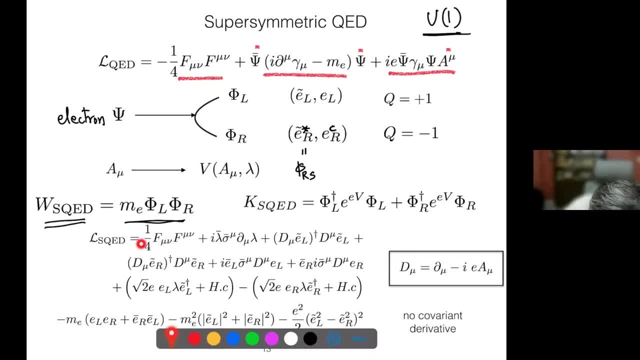 W. So the W gives me this function, the kinetic terms of the fortino and the kinetic function of the photon. This is the kinetic function of the fortino and this is the kinetic function of the photon. So this is given to me by the W And the K. the K gives me the covariant derivatives. 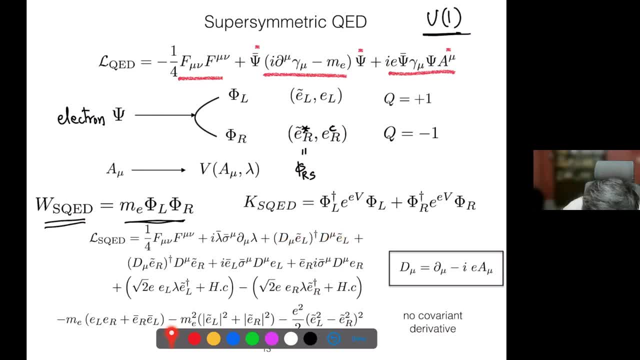 of El fields, Er fields, Okay, And the gauge interactions of the El fields, Er fields. And then another thing, Okay, Then another set of gauge interactions which look like Yukawa interactions here, which I told you, which are essentially electron selectron and the 14 ohm. 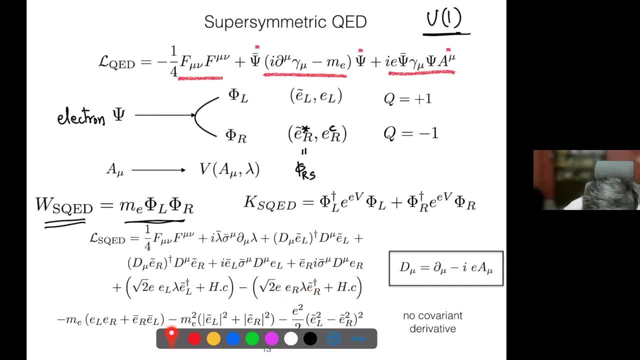 And right-handed electron selectron and the 14 ohm. They look like Yukawa interactions, but they have the same charge as a photon. I mean same coupling as the QED coupling, Same coupling as a QED coupling. And then I have terms from the W, which is M e l bar e r. 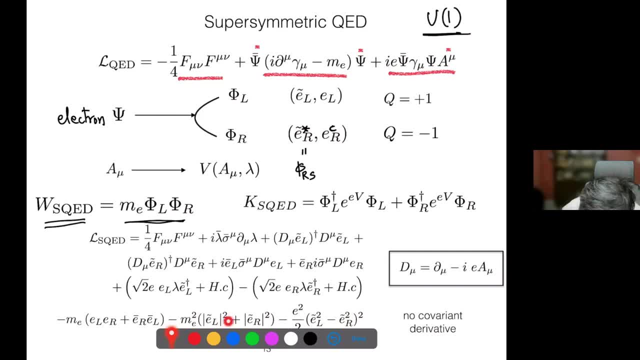 And here I have additional purely scalar type terms which come from. I'll tell you the source of this one in a second. actually, Let's, for the present, just take these terms as granted. These are purely scalar terms, meaning these are essentially selectron terms. 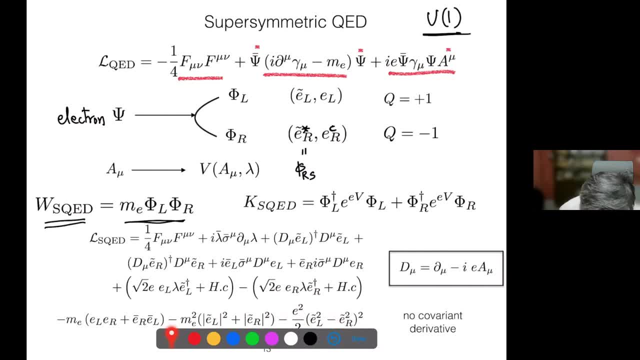 How do these selectron terms come? I'll tell you in a second. So far we have counted for all the terms. So the Yukawa coupling, which is essentially M e, M e, doesn't have Yukawa coupling because I didn't give any Higgs mediation or Higgs-Yukawa couplings. 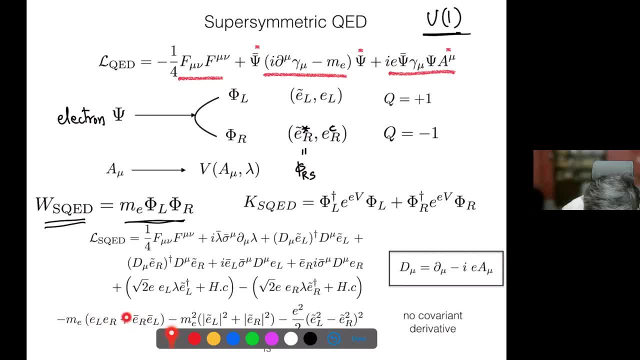 So I just have the term, which is essentially M, e, l, bar e r, e, r, bar e r, the mass term coming from W, the kinetic terms of the e, l and e? rs coming from this thing, and the gauge interactions And finally the other gauge interactions which are with the 14-ohm. 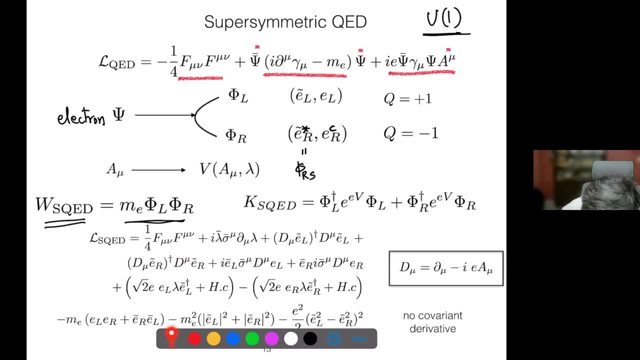 So the gauge interactions with the photon are given here And the gauge interactions with the 14-ohm are given here. They look like Yukawa interactions and so on. And then this is the kinetic terms for the gauge-in-ohm and the 14-ohm. 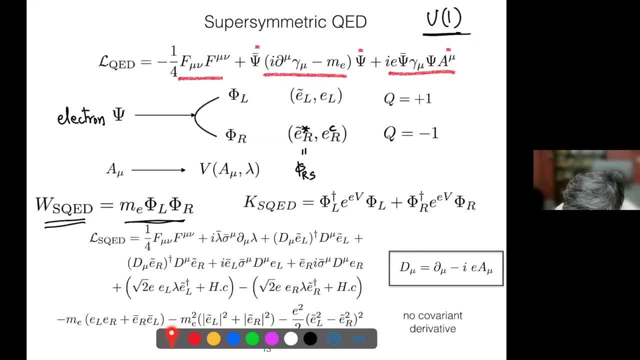 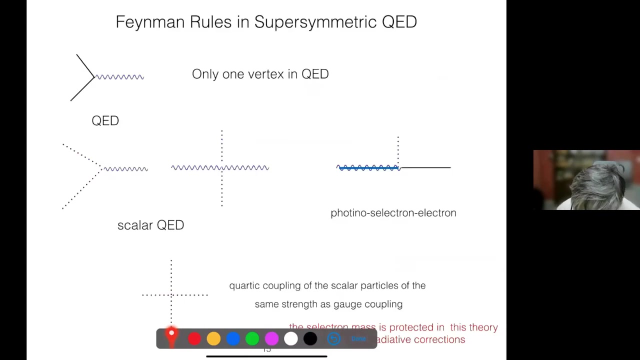 Now I'll come to these two terms which come. So this is your full QED theory. Now you started with just Particle spectrum. the particle spectrum is electron-photon and with that you derived your full QED Lagrangian Simply by following the three functions: the W, K and another W. 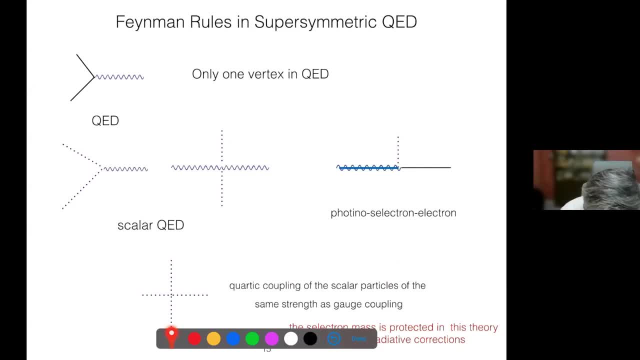 So normally in QED you only have one vertex, So we study with one vertex. essentially the first gauge theory we study is essentially this theory. There is only one vertex, which essentially photon with an electron electron-photon- There's only one vertex- is IE, gamma mu. 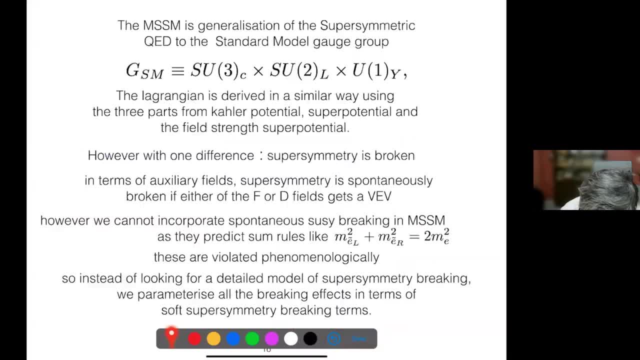 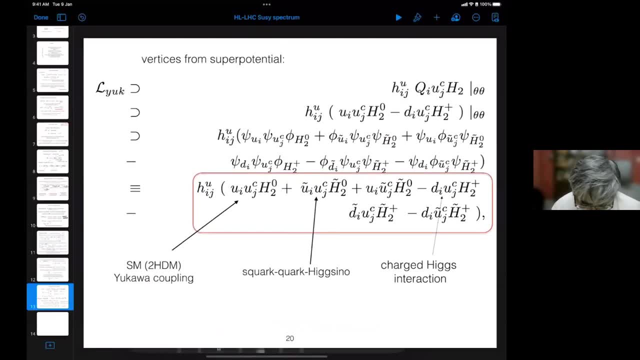 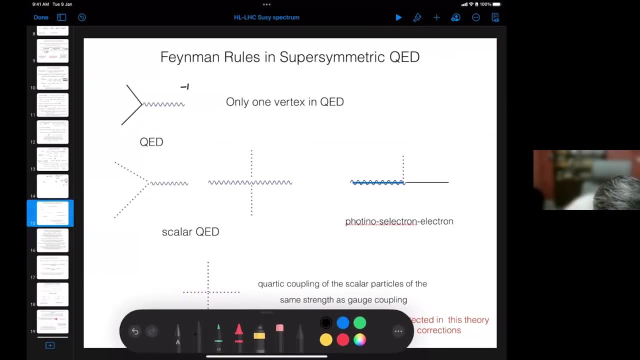 It gives me by IE gamma mu. let me just- it's fun to- oh God, this keynote just goes away. Let's just write down this: couplings: Essentially, this is IE gamma mu. Okay, Now, this is the only thing in QED. 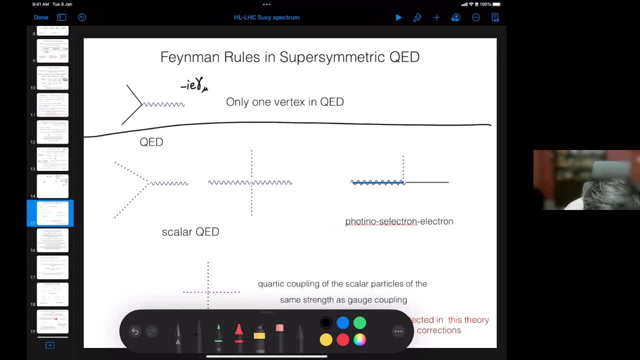 Now what we have is QED in supersymmetric QED you have first, for QED, vertex is there, which we have seen, because it comes from this one, this terms. Then you also scalar QED, because the supersymmetric partner of QED. okay, that is coming from. 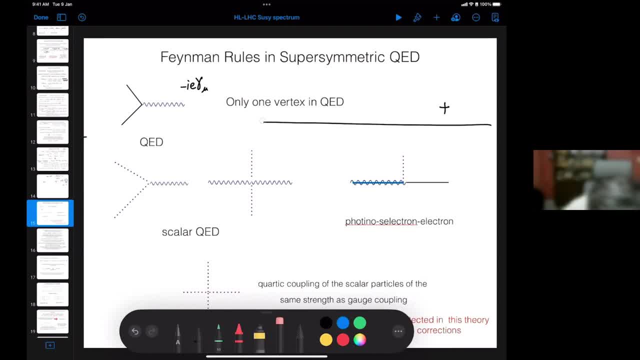 the scalar QED. Okay, Okay, So this last QED plus scalar QED, so this terms. so the scalar QED contains two terms: one vertex with the scalar, which goes as IE p mu plus p mu prime. So okay, 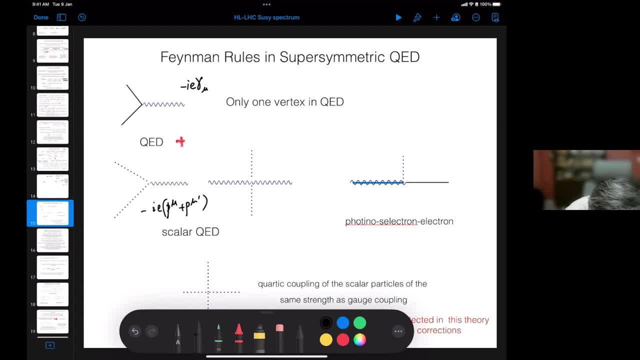 So this is the vertex, because instead of a gamma mu you get a p mu. here you have a del mu, So you have this and then IE square. The second is two photons and two scalars, which has squares of the coupling constant. 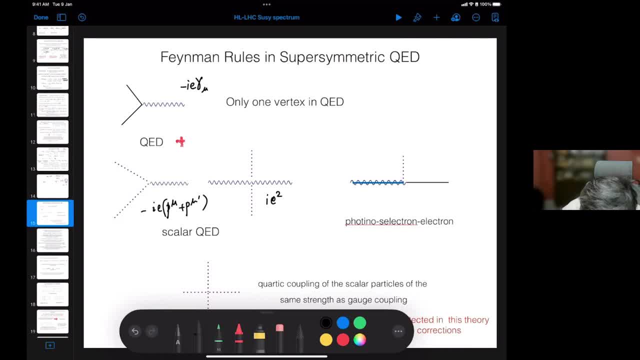 which is IE square. So you have scalar QED plus QED plus. okay, plus this new kind of a gauge coupling, this new kind of a gauge coupling which I am mentioning. this looks like a Yukawa coupling, like a Yukawa coupling which contains the KG node lambda, the electron or the selectron. 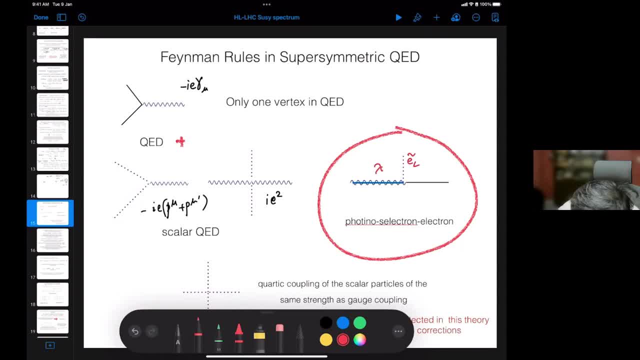 at the selectron El tilde and the electron El. So instead of two photons, what you put is you replace, So you start with this. So the easiest simplest way is that you start with the QED vertex and then replace this by superpartner. So replace this, You keep. 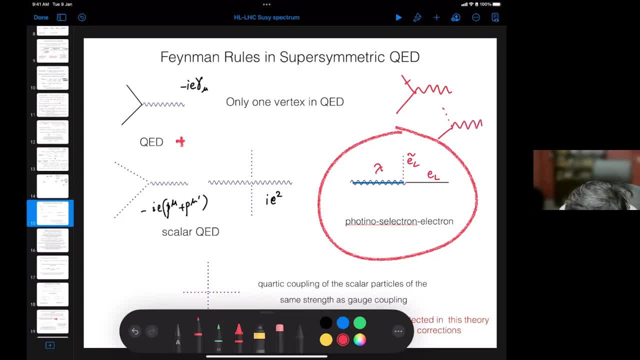 this one as this, So any two partners, So any two particles. you replace them by the superpartners For a given vertex. if you replace any two particles by the superpartner vertices, So lambda is essentially the superpartner, Superpartner of photon. So this has a photon line given by a fermion line, Both of them. 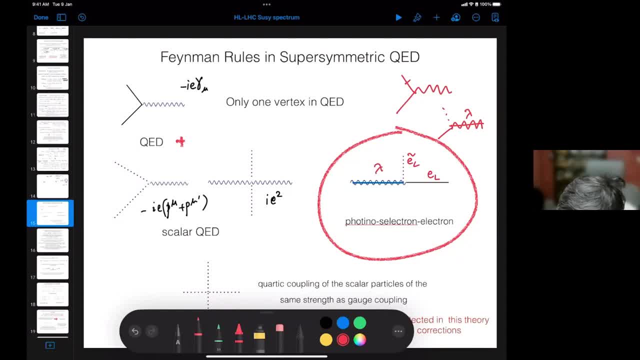 sit together. So it tells you that it is a gauge interaction, but mediated by a spin half particle. Okay, So take any vertex, replace each of them, any two lines with the corresponding superpartner lines and you get the fresh vertex. Okay, This is new, So you 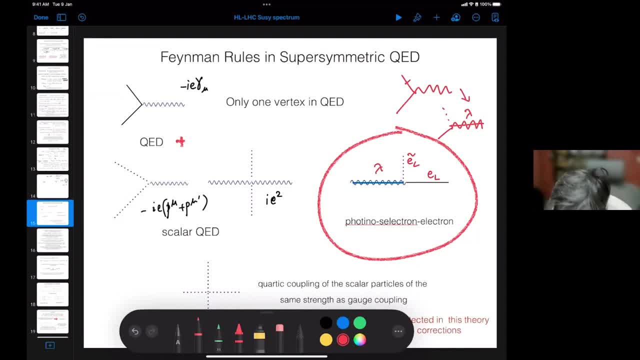 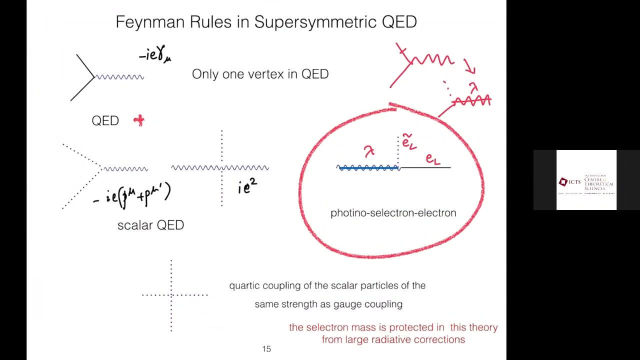 can see. this is new. This is the 14 ohm selectron electron vertex. This is a 14 ohm selectron electron vertex. And then you have. I do not know how to. okay, this goes away. Hello, sir. Can you hear me? Sir, the camera is slightly above. It is just light, Can you? 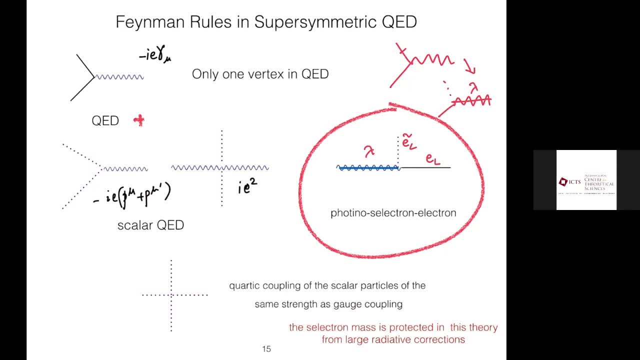 is it possible to bend, Because we can see only your head while you teach. Okay, Sorry, Actually, okay, let me reduce my monitor once again. Is this better? Okay, So then you have quartic. coupling of the scalar particles has the same strength of the. 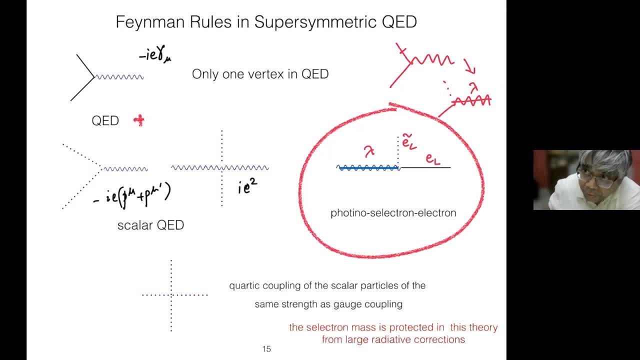 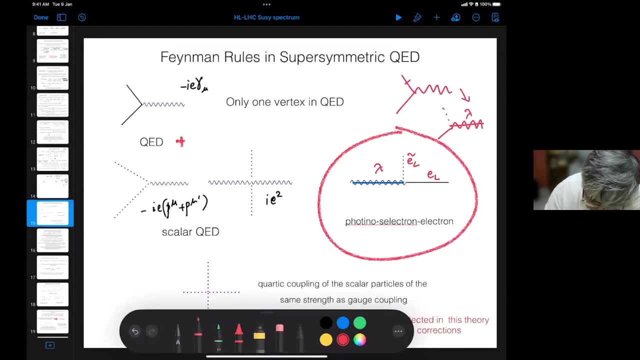 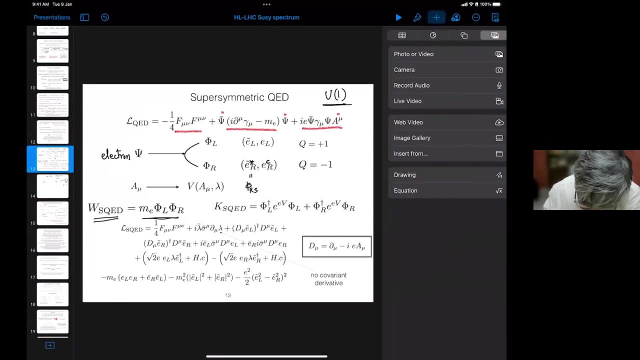 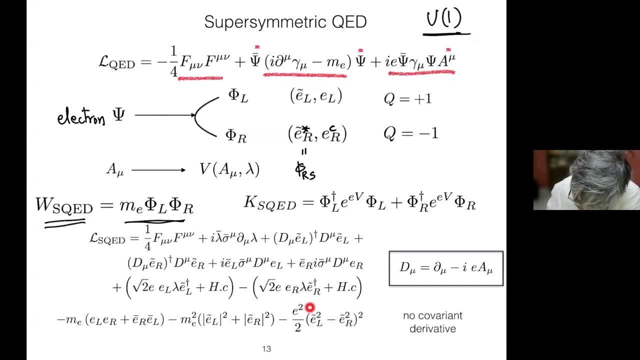 gauge coupling, So you also have one Particular coupling. This is coming from, this is coming from this theory. So this is coming from this term, this term- I will come how you get these two terms in a second. 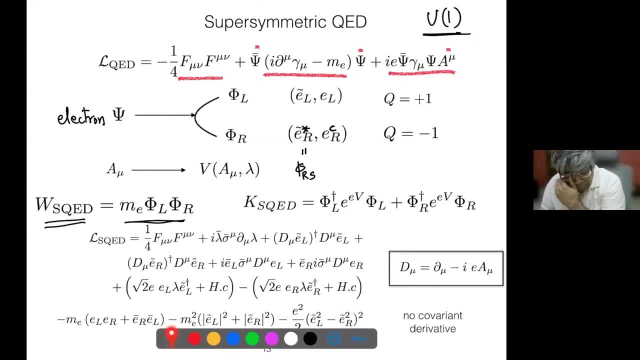 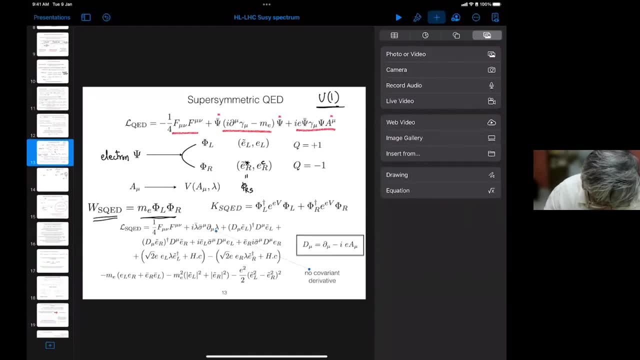 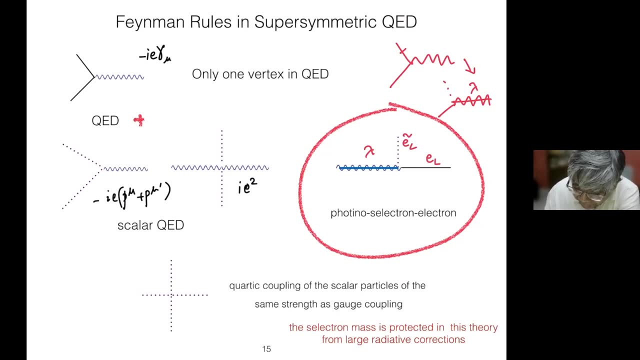 actually. So this is coming from this term. So what you have, you have a, you have a, you have derived. you have derived all possible couplings, okay, all possible couplings- of a supersymmetric QE, okay, and you have derived its spectrum. The spectrum is nothing but. 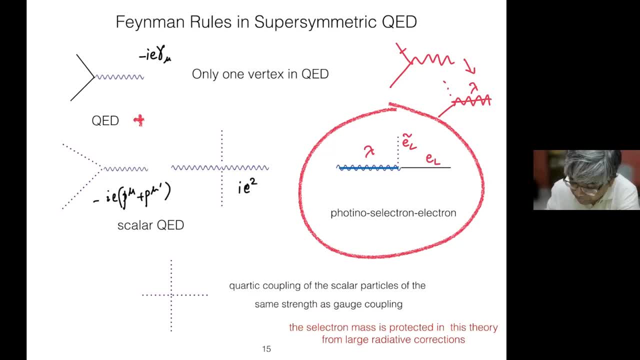 so the particles are electrons, selectron, photon, 14 ohm There are. so you double this particle spectrum, okay, and the masses of the photon and 14 ohm are the same. So 14 ohm is massless. 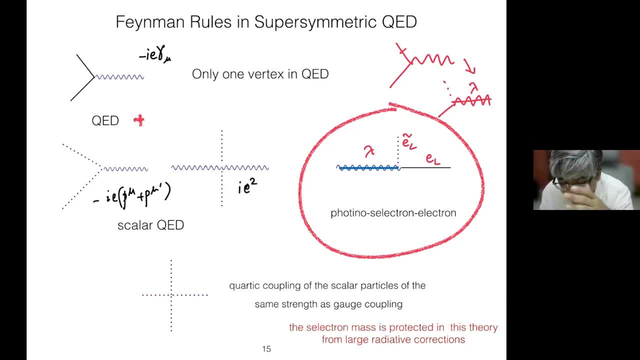 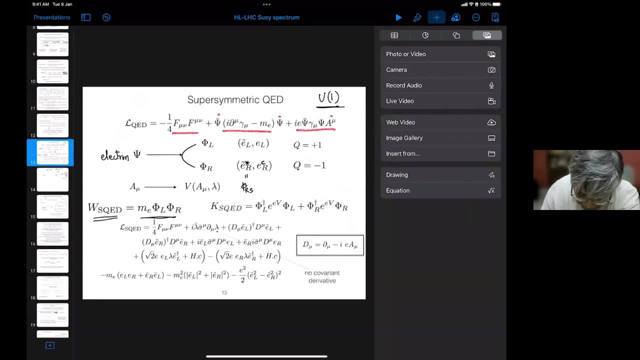 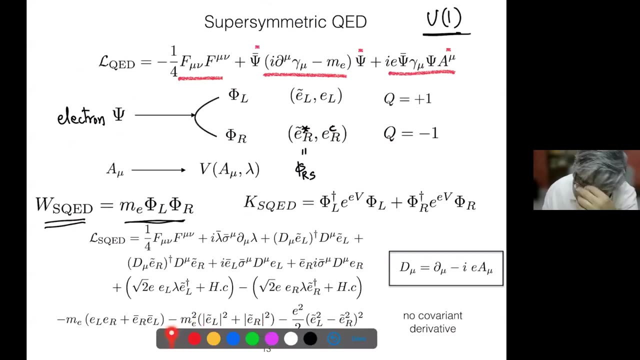 And the electron and selectron has the same mass. Electron and selectron have the same mass, as you can see from this term. Okay, So from this term, as you can see, the electron and selectron have the same same mass. Okay, So the spectrum of the supersymmetric QED. 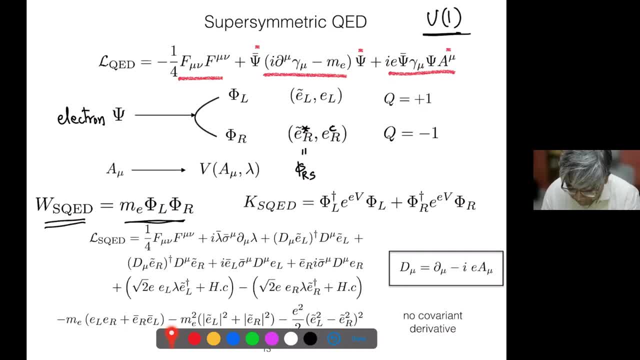 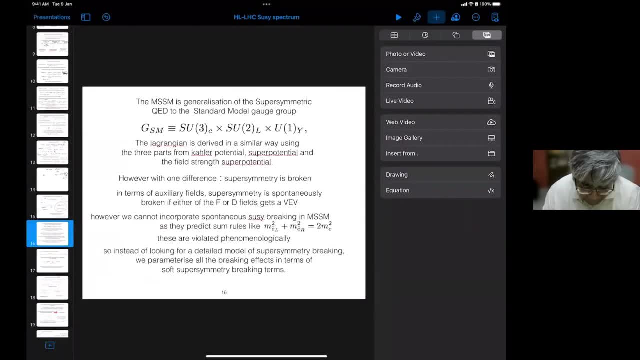 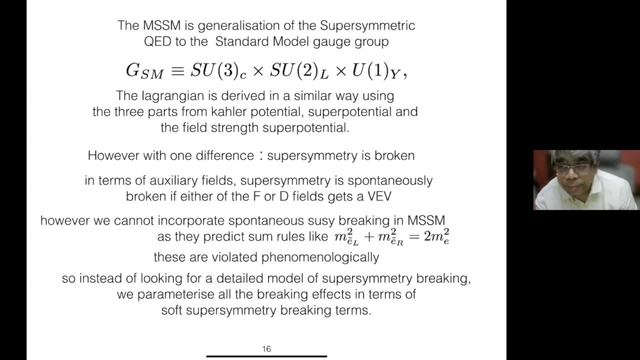 is now fixed. You know how to you have computed the spectrum. You have not broken the supersymmetric QED, But anyway, we'll do that in a second. actually, Any questions on this part before I move to MSSL? So okay, if you don't have questions, so I will come to how to get yeah. 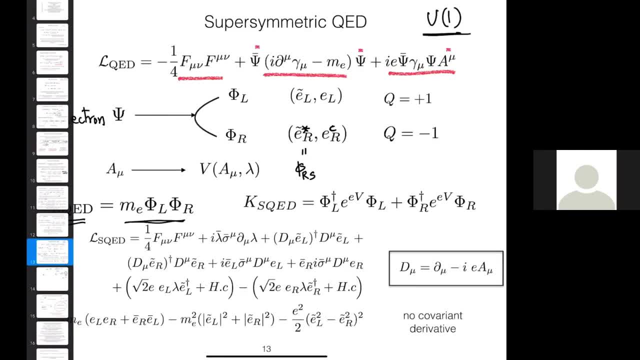 I have a question. So when you talk about these auxiliary fields, yeah, they are needed for the formula, So you can talk about the particleism, But practically, what is the implication in terms of the particles? Practically, in the sense, 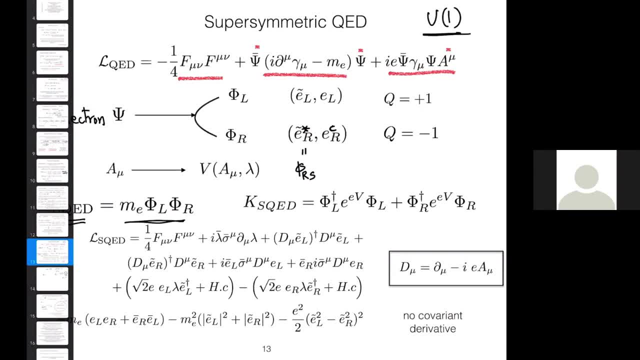 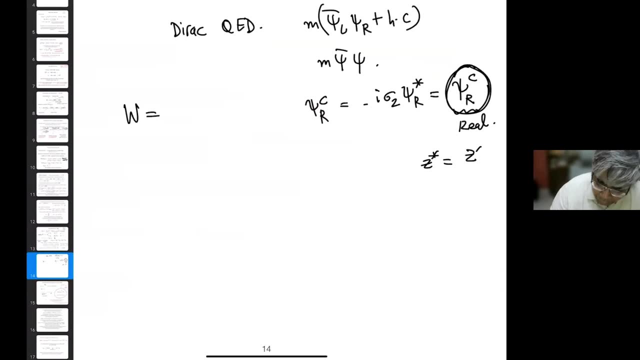 In the physical masses, states or something. They are not physical but formalism-wise, they're extremely important. They're the. they make life easier. You can do the entire thing without actually. so the auxiliary fields play two roles, Okay, because? okay, let me answer this question in a. I'll tell you how you get these two terms. 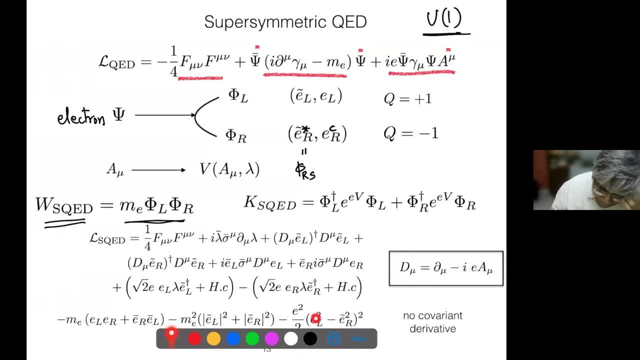 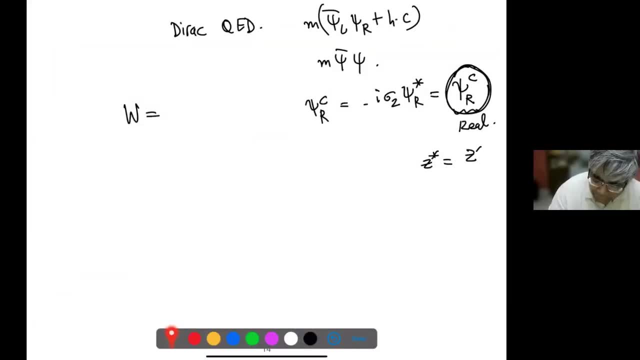 Okay, because, okay, let me answer this question in a. I'll tell you how you get these two terms okay, and then you will understand why they, they play a role. okay, I think that slide, I haven't stressed it, or it's broken or closed or something. oh one. 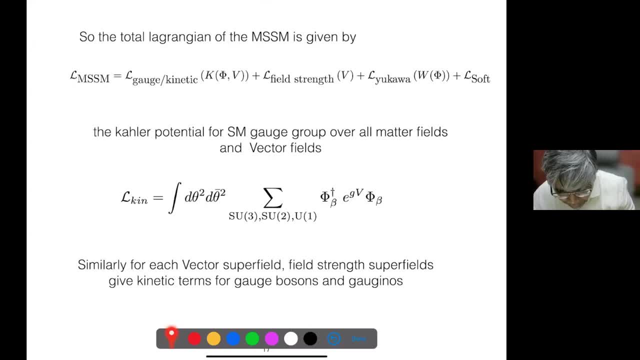 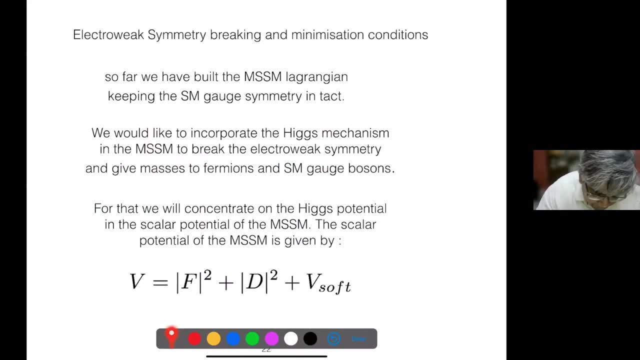 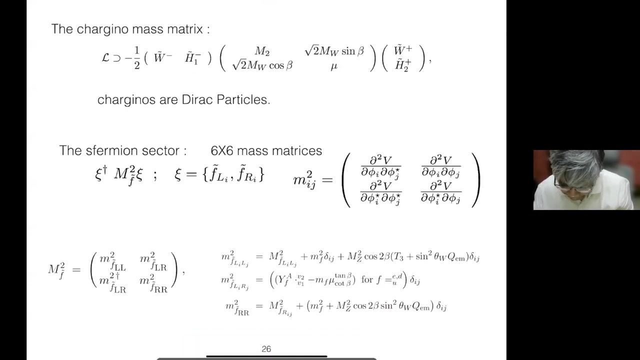 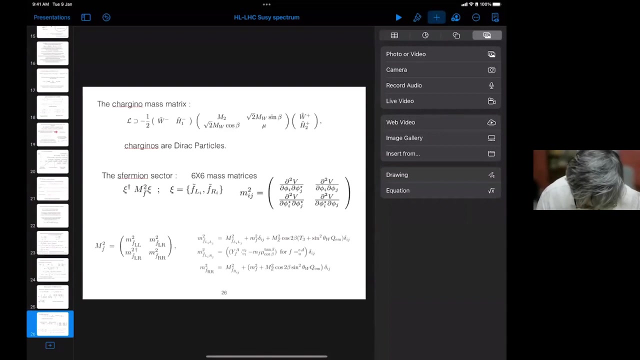 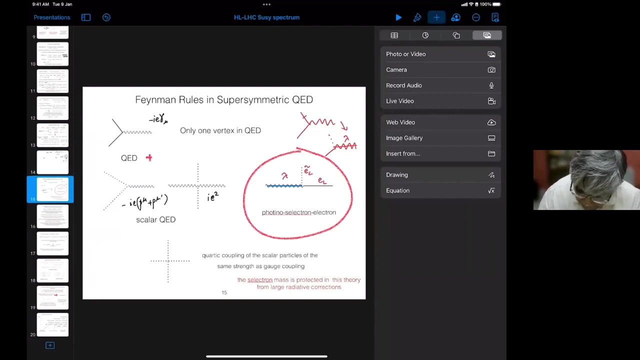 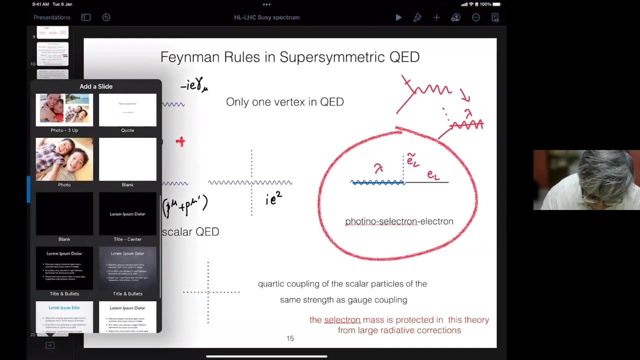 second. oh god, on an iPad, if you want to run, you know it's very complicated. oh god, give me one second, so I'm going always ahead, okay, so let me just add one line, one thing here about the auxiliary fields. I'll just add a slide and mention this. so the auxiliary fields. 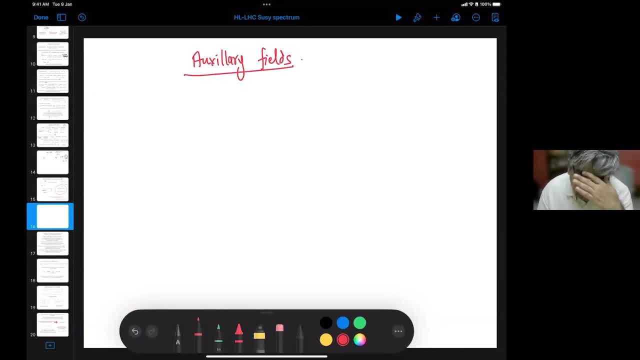 please play two important roles. so they're unphysical, but they keep track of things like the scalar potential. the scalar potential of the theory is given by mod f square plus mod d square. okay, this I have not. I have a slide, but but I, okay, I'll write it down. so so f. 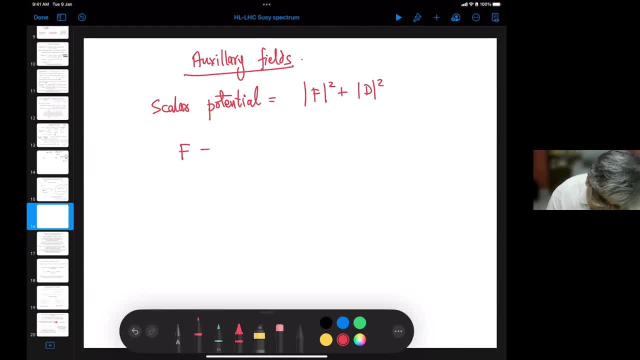 if you use the equation of motion of the f, it comes out to be del w by del phi i. so this term is nothing but f f star d. if you do the entire analysis, it'll just come out to be phi star tau a, phi. so d a is g square, phi star tau a is the generators. if it is u1 it is just one. okay, tau a are the generators. 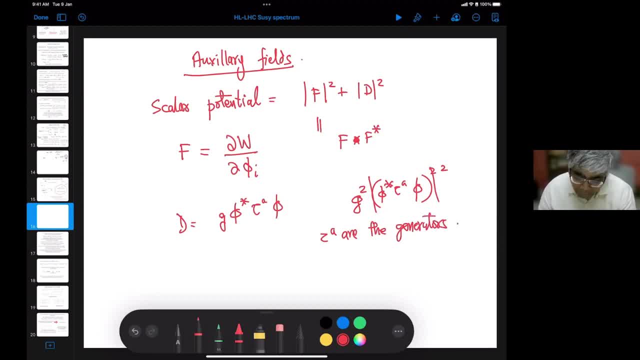 so. so f gives you the scalar potential and it also gives you the self-couplings of the scalars plus masses of the scalars. so the mass of the selectron comes from the f term. the mass of the selectron comes from the f term. 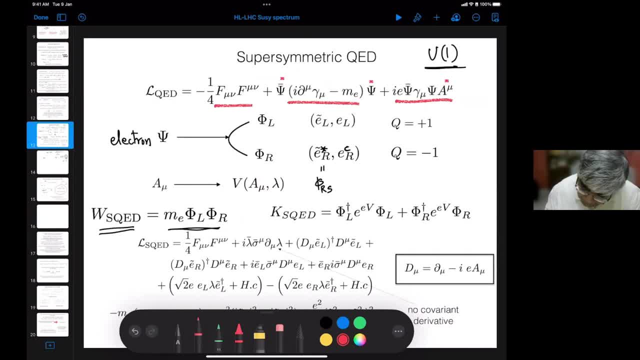 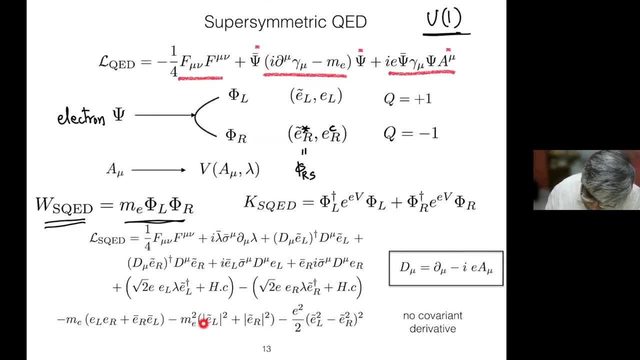 so this terms, these two terms which I wrote on here at the end, this is an f term, this is an f term and this is a d term which comes with the gauge coupling constant. this is an f term. the full super potential, the full supersymmetric Lagrangian contains not only all these terms. 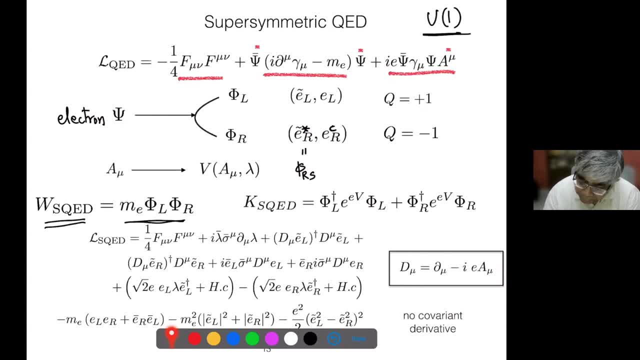 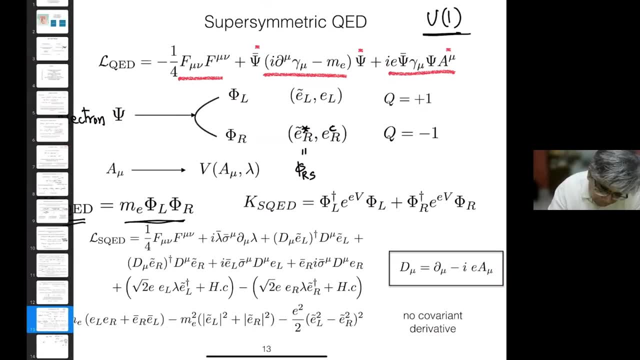 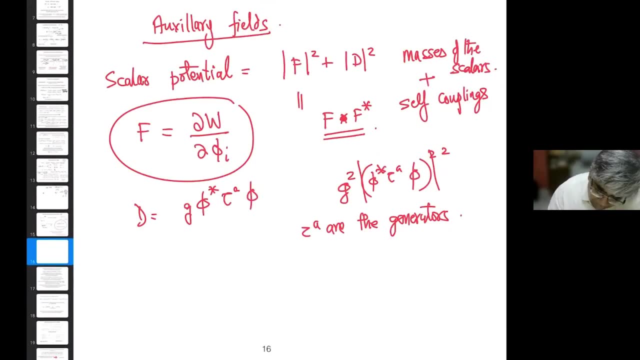 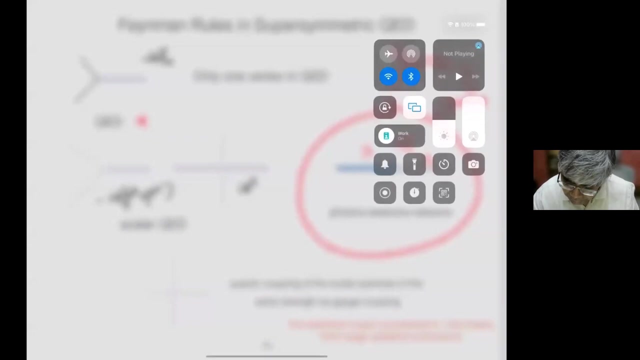 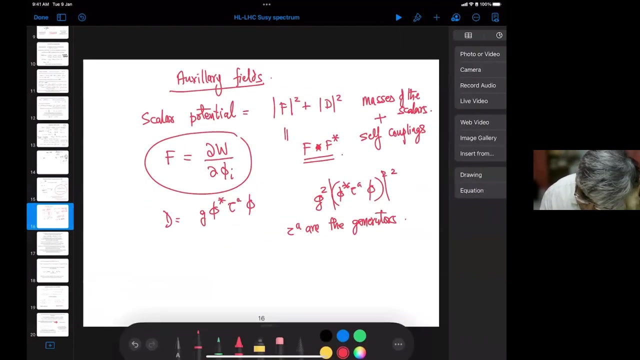 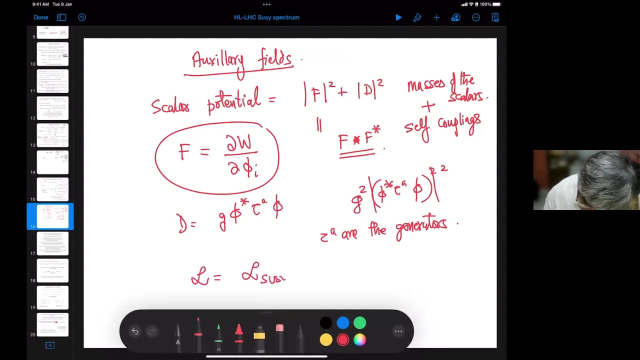 coming from w, k and curly w, but also the v, and the v is defined in this particular fashion. okay, the v is defined in this particular fashion, so the v is the scalar potential. sorry, this touch id is playing the role. ah, two pinch, okay. so the v, v. so l total l is equal to l suzy plus v. 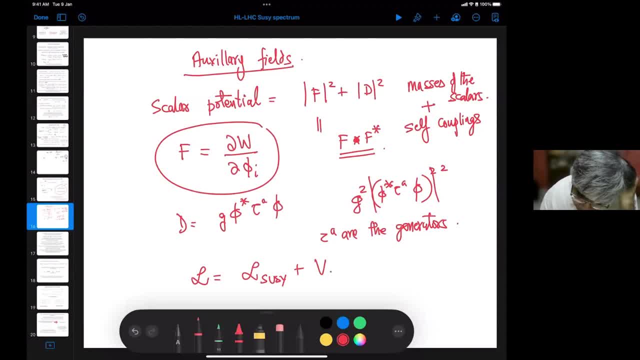 now f terms are the scalar potential. now, because they contain terms, just because they are unphysical, their equation of motion is like this: that means you set them. so you say that equation. how do you get this term? you get this term coming from if you write an equation of motion for them. 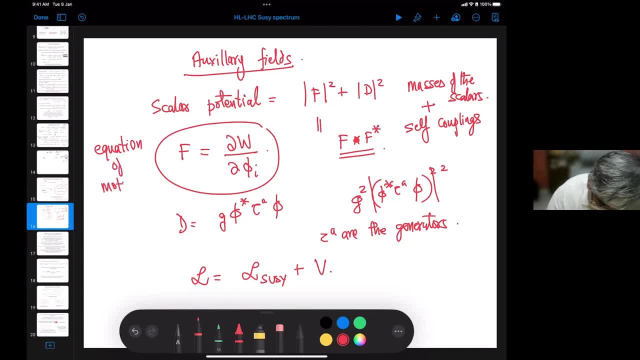 it gives you f plus del phi i is equal to zero. okay, so this is an algebraic equation, it's not a dynamical equation. so this you can set it to be so, because there is no other way where the f terms will come. there is no other place in the entire Lagrangian the f terms will come. 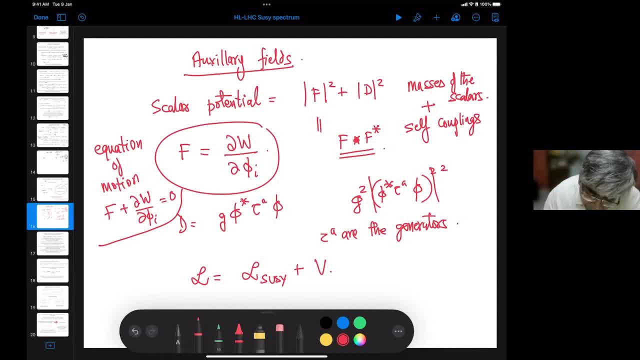 so this is the equation of motion and then you solve for that the f term. now, the f term because it's purely scalar, and the entire supersymmetric scalar theory, purely scalar part, comes just from the f terms. okay, and the d terms. so, if you want to break, 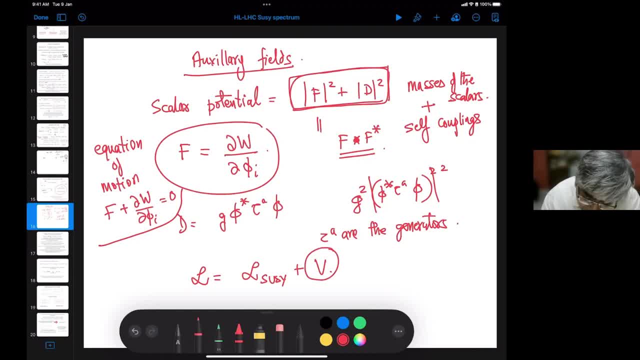 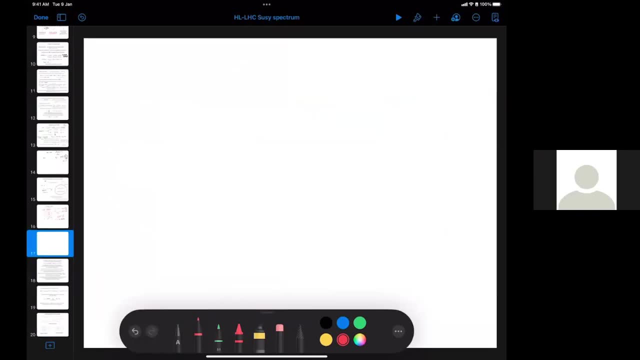 supersymmetry. if you want to break supersymmetry, you have to break. give a vacuum expectation value to either f or d. okay, so they play. so for example, let's just take w is equal to phi i, phi j, phi k times d, theta. so these are your chiral superfields, and each chiral superfield contains one scalar phi i. 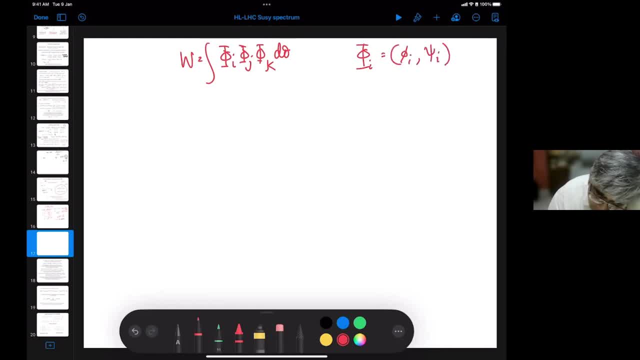 and one fermion psi i. now, if you derive del f, phi is equal to it. gives me a sum: phi i, phi j, okay, whole square. or let me write it down explicitly. so this will give me: say, let's just write three terms. simplest thing is let's write one, two, three. there are three chiral superfields. i write it on phi 1. 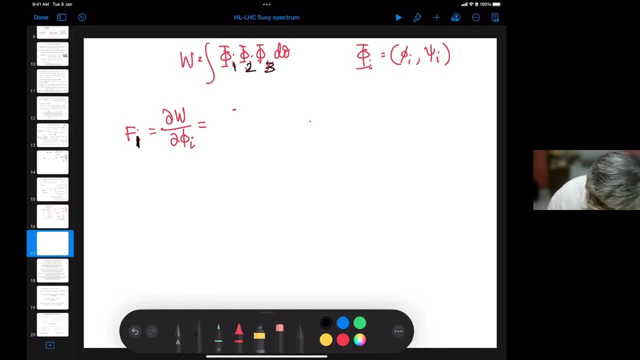 phi 2, phi 3. then i derive f1. f1 would be phi 2, phi 3, f2 would be del w, phi 2. so that gives me phi 1, phi 3, f3 would be phi, phi 1, phi 2. so my scalar potential would be the scalar parts. these are just the scalar parts. 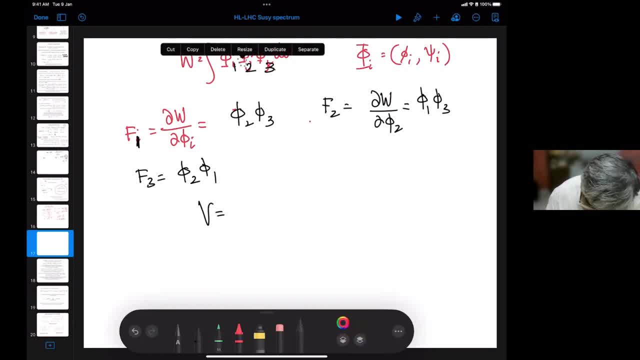 so these are the capitals, okay. scalar parts would be: phi 1- phi 2 square plus phi 1- phi 2 square plus phi 1. phi 2, phi 3 square plus phi 1, phi 2- phi 3 square plus the gauge thing which is coming. 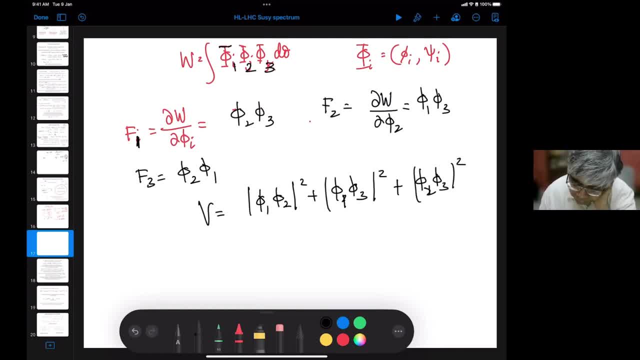 from the d term. so now, if you want to break supersymmetry spontaneously- spontaneously means by giving a vacuum expectation value for any of the scalar fields. for any of the scalar fields, okay, i have to make sure that some of the f- because we is equal to f square- sum over i f square. okay, some f has a non-zero expectation value. 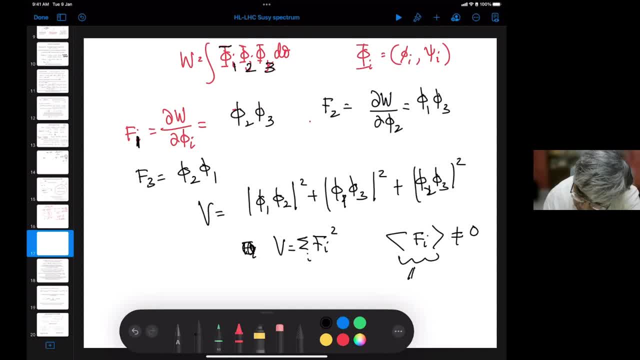 physically, this f could be some combination of scalar fields, okay, uh, okay, so physically this f could be something. so this combination should get a expectation value, okay, non-zero vacuum expectation value, such that the f becomes a non-zero vacuum expectation value. so there are some physical fields, some physical combinations of. 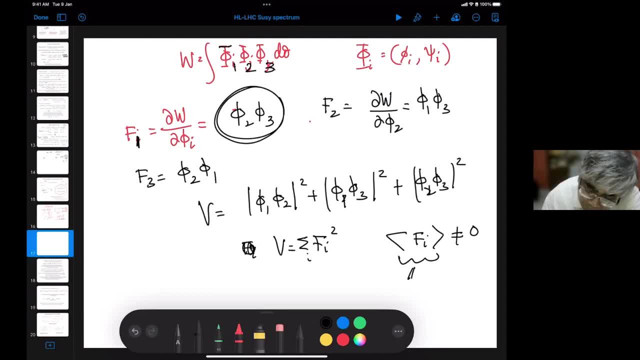 fields which should get a vacuum expectation value such that supersymmetry is broken spontaneously, because the only way you can give vacuum expectation values to the scalar fields. did i answer your question, sima? yes, thank you for explaining it so nicely. okay, so, uh, physical, uh, so physically it could mean something else. phi 2, phi 3 could be a some. 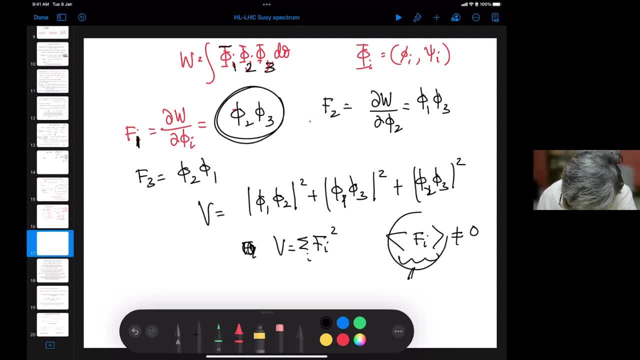 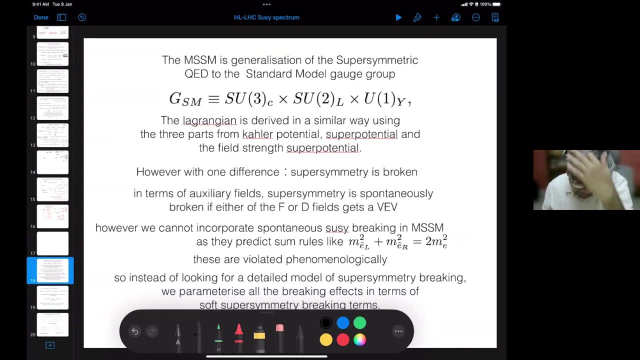 combination. but, uh, keeping track is very easy, uh, by using the auxiliary fields. okay, if you do it in a component formalism of supersymmetry, this becomes quite complicated. actually, you may not be able to keep track of this, okay. uh, so, coming back now, what let's? what we do is, since we understood, 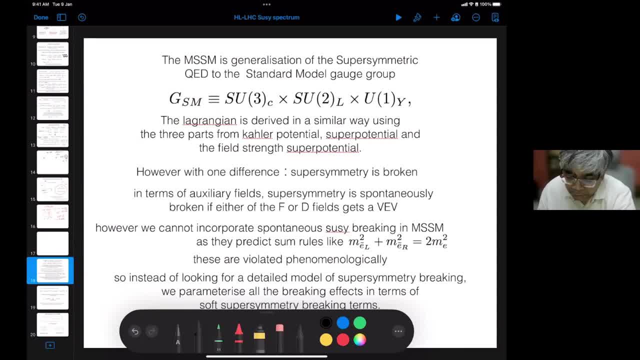 uh, so the supersymmetric qd, uh, before going for the any further questions, actually, yeah, no, i don't see any raised hands, or okay. so, yeah, go ahead. okay now. uh, the mssl is a generalization of supersymmetric qed to the standard model gauge group. now i just change the gauge group and modify the particles spectrum, i add: 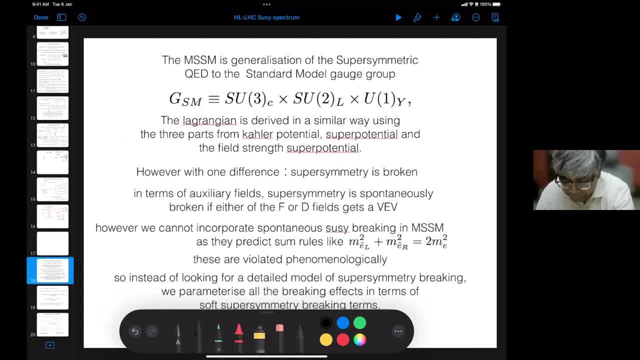 all the rest of the fermions: electrons, quarks, nuanced towers, everything, all the quarks and electrons, and for each of them i add two chiral super fields. but if this helps, qd is not a current theory, but standard model is the chiral theory. so you work with the chiral multiplates anyway. 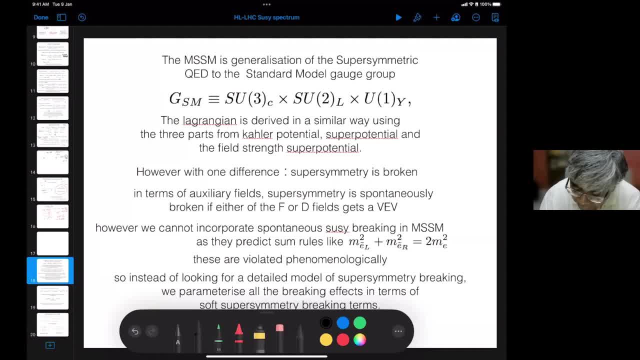 because chiral standard model is the character we. so you have left-handed particles and right-handed particles separately. So the left-hand particles you add chiral super fields, right-hand particles you add chiral super fields again, and then your gauge group is a large gauge group actually. 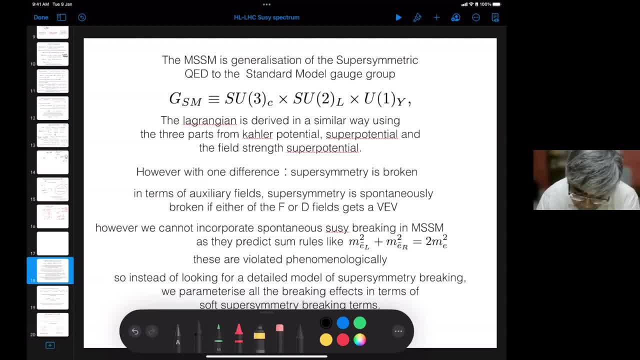 You have SU3C, color SU2L and so on, And so the Lagrangian is derived in a very similar way. three parts: scalar potential, super potential, field strength potential. But one important thing is in the supersymmetric QED we didn't break supersymmetry, But in nature we have 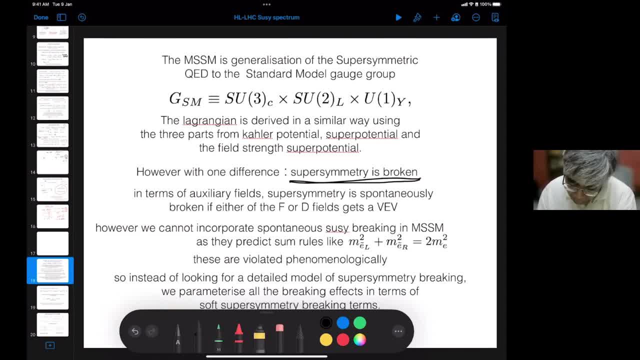 to break supersymmetry, okay. So supersymmetry should be broken. So if it is broken spontaneously, okay, I will come to supersymmetry breaking in a minute because I had to do something about the Hiral situation okay. 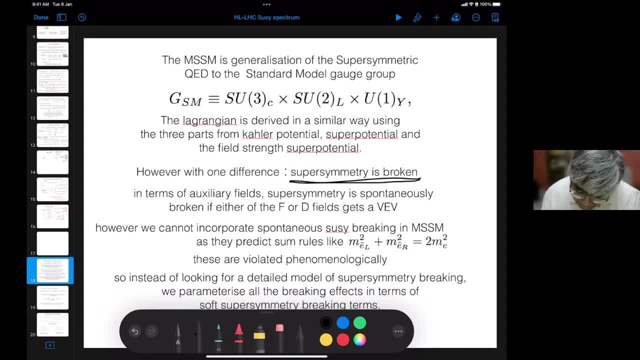 Like I just talking to. we just talking essentially. that F and D terms gets well In any of the some F or D terms, some fields, these auxiliary fields, get well. However, we cannot incorporate spontaneous supersymmetry breaking within the MSSM fields. Within the MSSM fields means 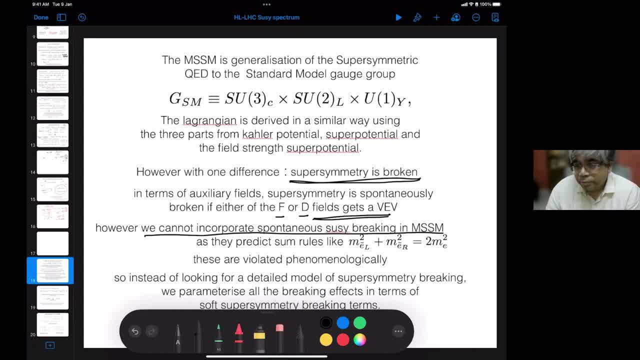 within the standard model super fields, none of the chiral super fields. if you write there F terms and D terms And then give the vacuum expectation value, It leads to problems. Actually leads to some rules, because a supersymmetry is a very, very constrained theory, because you know what the 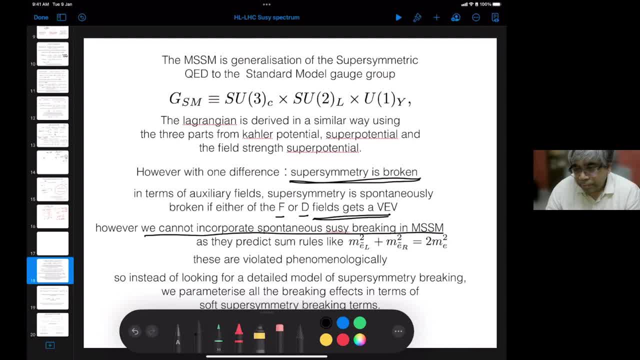 combination of F terms is Okay. the combination of F terms is like quartic terms, like E, square, and the mass terms are same. So if you believe in spontaneous supersymmetry breaking, it cannot be done within the standard model MSSM super fields because it predicts masses like 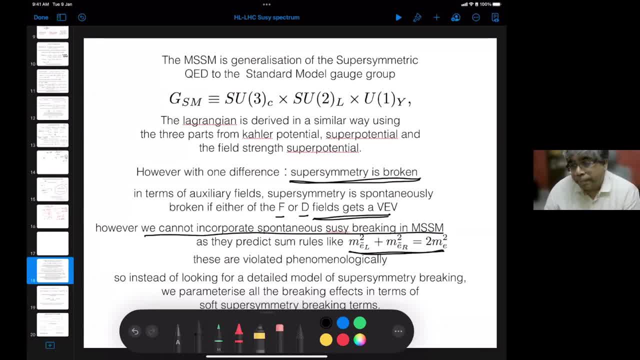 this: For example, if you break in supersymmetric QED, okay, if you break within the supersymmetric QED, you will have relations like the masses of the two selectrons or the electron mass should be equivalent to the electron mass. Okay, if you give by. this is what I am saying. 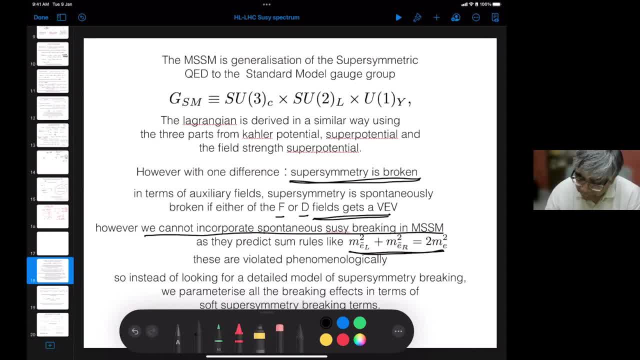 if you give a combination of the selectron fields, giving a vacuum expectation value, it predicts that the mass of the selectron field should be equivalent to the mass of the electron field. which is not done. which is not done, okay. So instead of looking, 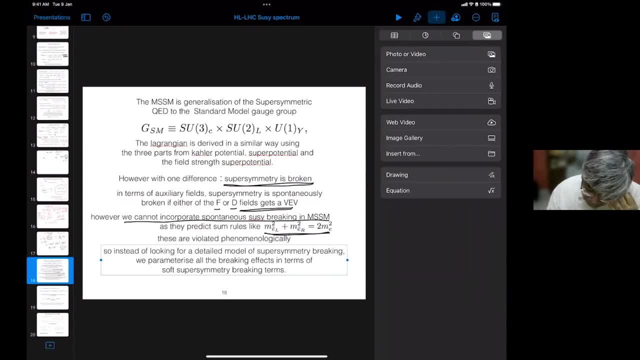 for a detailed model of supersymmetric breaking. what we do is we parameterize all the breaking effects. Now, when I say here breaking effects, here, the idea is like this: You know what is the resultant of a spontaneous symmetry breaking theory? Okay, 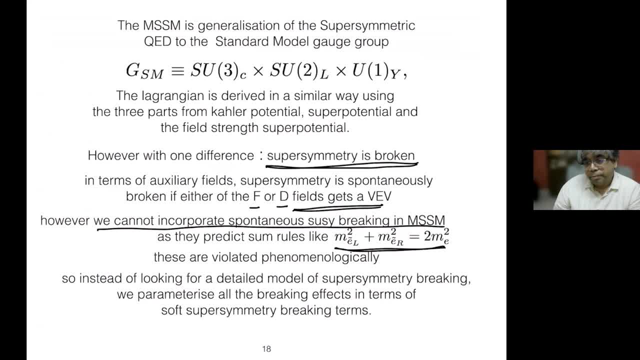 In a spontaneous symmetry breaking theory. you know what is the resultant of a spontaneous, spontaneously breaking theory? you only get soft terms. If supersymmetry is broken spontaneously, it will only lead to soft terms. okay, meaning soft terms means dimension, full terms, Okay. soft terms are terms in which they are just like masses, which do not depend. 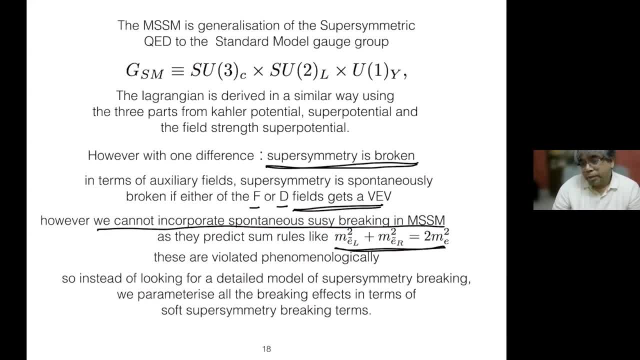 upon momentum, meaning there is no del mu, okay, there is no p mu, or there is no lambda meaning forward. So all the couplings are dimension. there are no dimensionless couplings. Let me put it this way: easiest simpler thing is: there are. 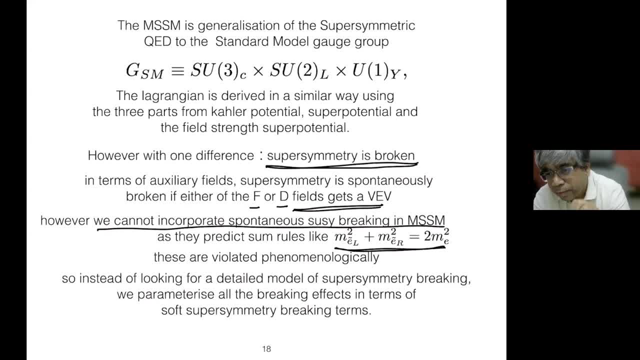 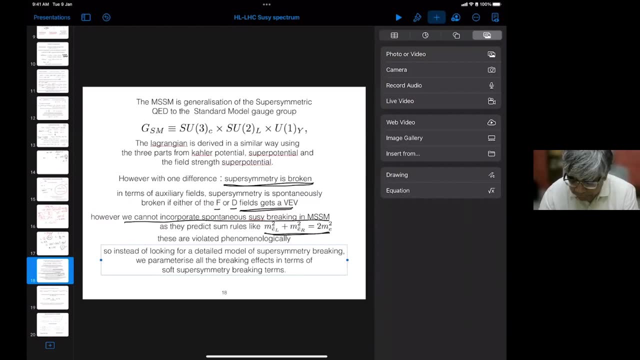 no dimensional couplings. All the breaking effects would be proportional to dimension. full couplings. So they are all super renounceable terms. okay, So you know what are all the possible soft terms which are generated by spontaneously broken supersymmetry. So you: 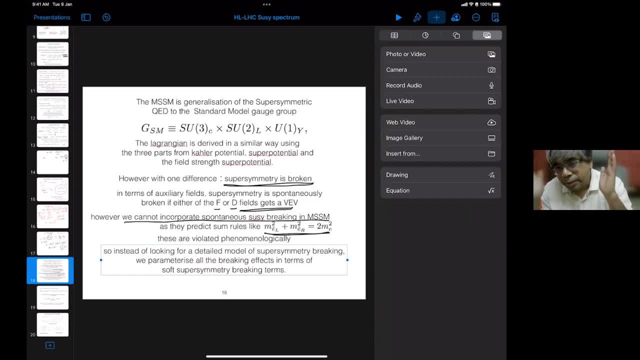 just add them. you do not know how they come. you just add all these possible spontaneously broken soft terms. So you just add them. you do not know how they come. you just add all these possible soft terms. okay, That's what we are going to do in the in building. 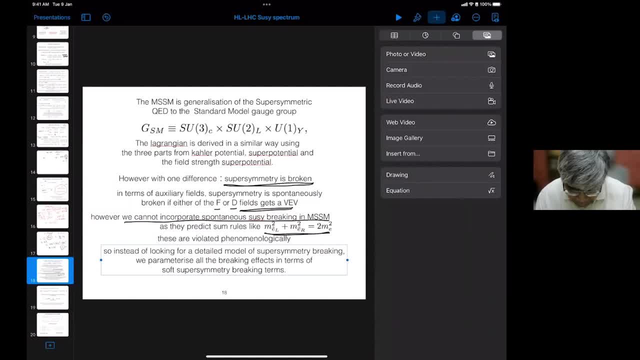 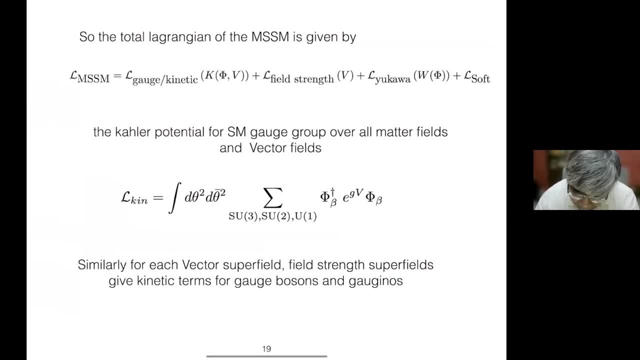 this MSSM actually. So let's start with building the MSSM. Okay, so the total Lagrangian again is given in the format as follows: you have the gauge kinetic part, which is k, essentially the killer potential, the field strength, and the Yukawa part, which is the flat root of 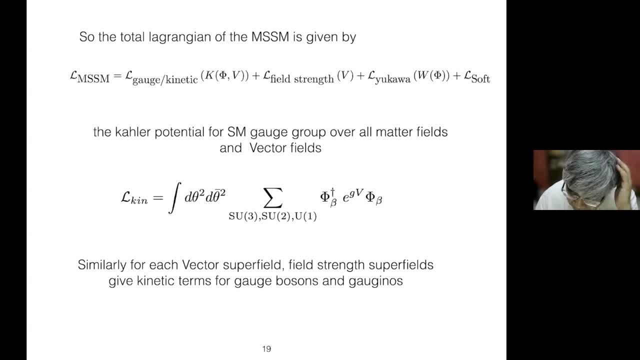 the mass, the, the super potential, and then you have this else soft, which i am talking about, which is, i just add, all possible supersymmetric breaking terms, okay, which i believe. these terms are somehow generated. they are somehow generated in some other sector, but they are present somehow. i don't know how they are come, but i'll write them, all of them, by hand. 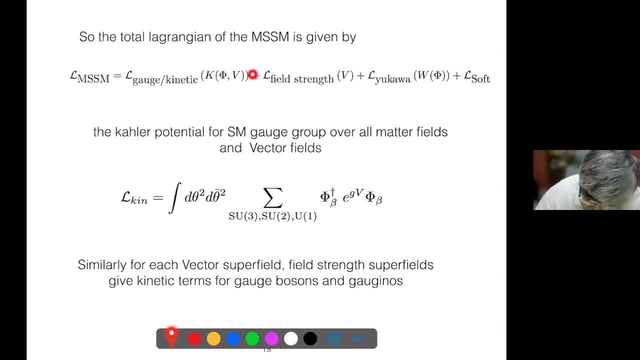 i don't break supersymmetry in any of this sector, okay, in any of these chiral super fields. i don't break supersymmetry spontaneously, but i say somehow this spontaneously, or the resultant soft terms which come from spontaneous symmetry breaking, supersymmetric breaking, are added into the lagrangian by some reason. 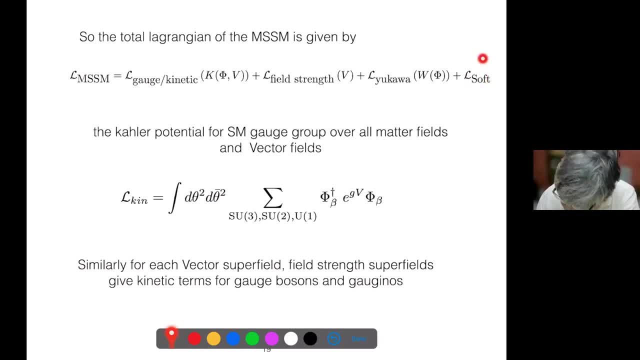 but there are models which give you this kind of soft term. there are explicit models which give you, you, you, this kind of soft term. there are explicit models which give you this kind of soft term. and this is possible. one shouldn't take it that it's some hand waving argument or something. 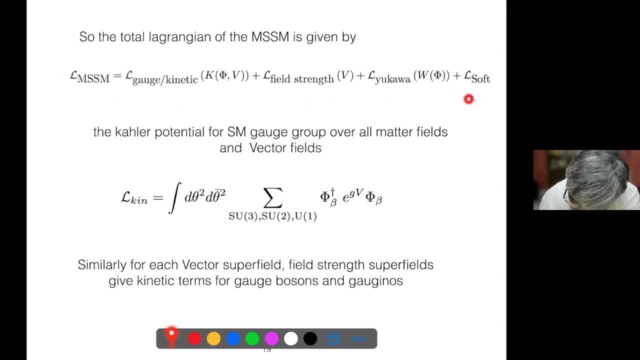 um, if i have time, i'll tell you more in detail, but this part of this sort of a lagrangian l soft is clearly completely possible. okay, it's completely possible and there are. so the simplest models are minimal: super gravity, cmssm, uh, gauge, mediator, supersymmetry, breaking all these things will predict what these soft terms are. 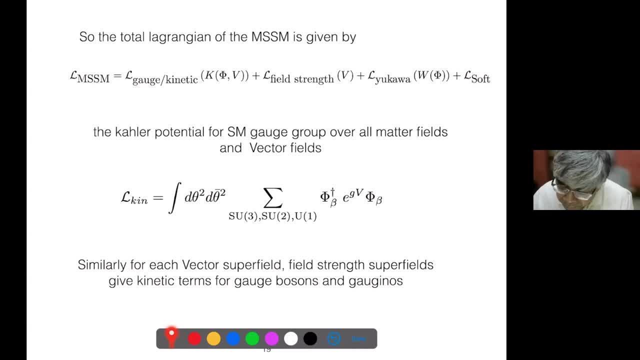 and they give explicit forms for the soft terms. they believe in something called the hidden, uh, hidden sector, which doesn't contain standard model interactions. so in that sector, supersymmetry is broken spontaneously. there is a question: yeah, can you go ahead? yes, sir, uh. so i was asking, like, for a spontaneous breaking of any internal symmetry. 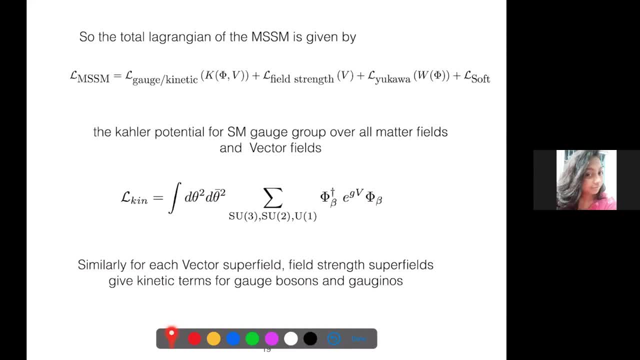 we uh get a gold stone, we have a goldstone theorem and uh. so for uh suzy breaking, is there any analogous mechanism or yeah? yeah, it's a very good question, actually, it's very good. so there is gold stones and there are also gold steinones means supersymmetry is broken spontaneously. 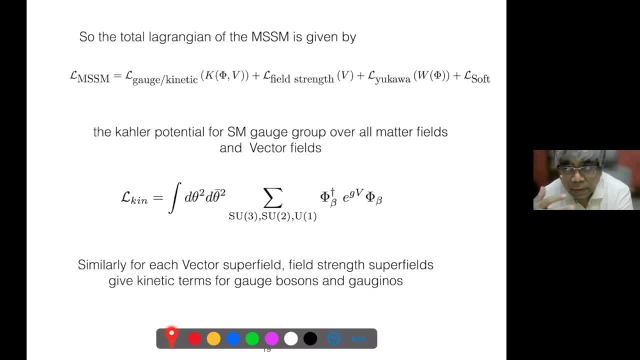 okay, there are spin half fermions, which are also massless, okay, which are called gold steinous, which happen, uh, appear, when supersymmetry is broken spontaneously. uh, but what happens? uh, he. so you have to be very, very careful when you break supersymmetry. these goals, you know if they are. 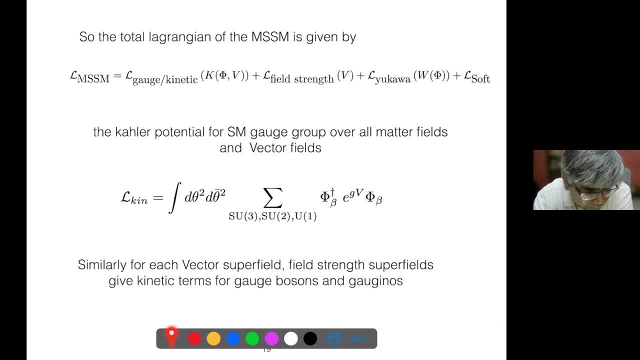 massless and, uh, if you want to make some massless fermions or any massless particles, extra massless particles, so their coupling strength will be proportional to the breaking strength of super symmetry. okay, so if their coupling strength will be, say, if you are um and the scent of submittive breaking and something called the mediation scale, so if it, 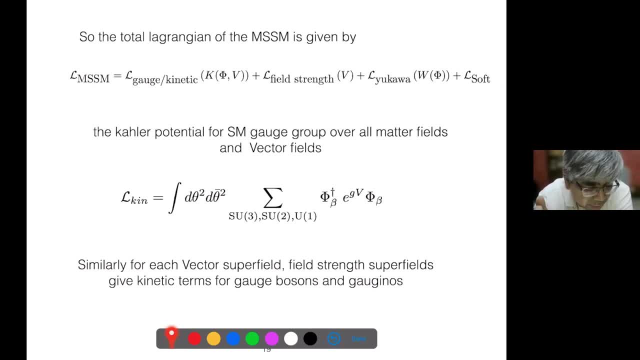 is gauge mediation, it will be the mediation scale of the gauge mediation or if it is a gravity mediation, it will be one by a plank. so this coupling, so these are light particles, meaning massless particles. with very light uh couplings they could be dangerous but in a 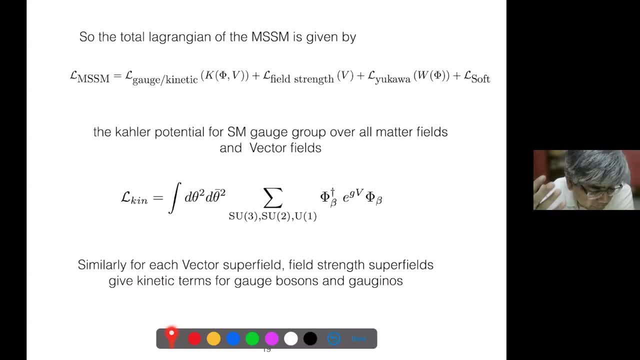 super gravity mediation this goldstein is actually. there is something called a super higgs mechanism which happens: the goldsteiner is eaten by the gravity, you know the gravity, so the super partner of gravity, graviton, and that becomes massive. so this is called the super higgs mechanism. so yes, it's a good question. yes, gold steiners do happen, they are there and 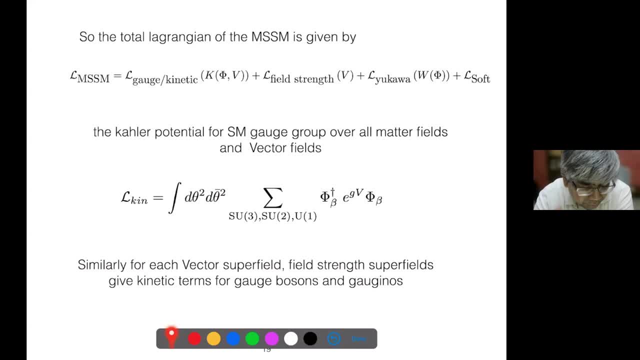 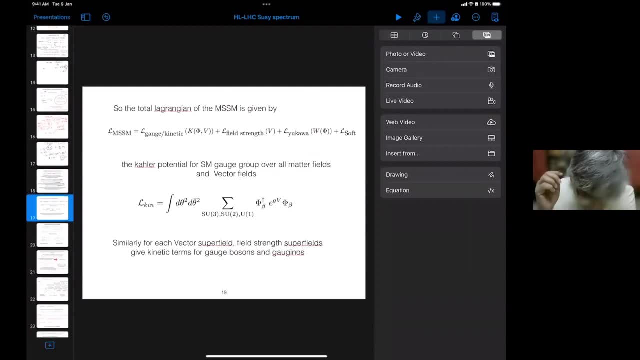 they have very strong phenomenological constraints. okay, gold streams have strong phenomenological constraints coming from cosmology and various effects, essentially so for goldstone. they are different from our goldstone. bosons like ghost and boson are not physical particles and they get absorbed in the longitude. ghost and bosons are absorbed only in um local gauge theories. 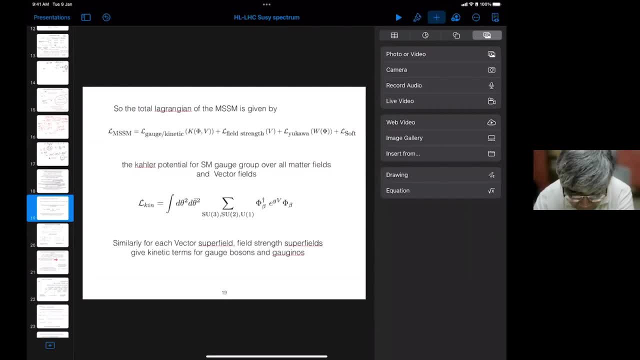 so ghost stones can, uh, goldstone bosons can happen also in. uh, if a symmetry is there, it is broken spontaneously. you can still have goldstone bosons, okay, okay, and they have severe constraints. you cannot have free ghost from bosons. the supersymmetry which we are talking about is a global supersymmetry, sometimes also called 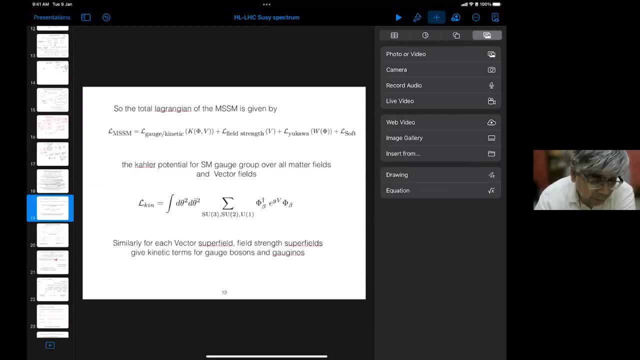 rigid supersymmetry. so in such a case you can have both goldstone bosons and also ghostinos. but if you go to a local supersymmetry which is called super gravity, they get eaten up. they are absent in the physical theory. and what in the? in that case, what happens? 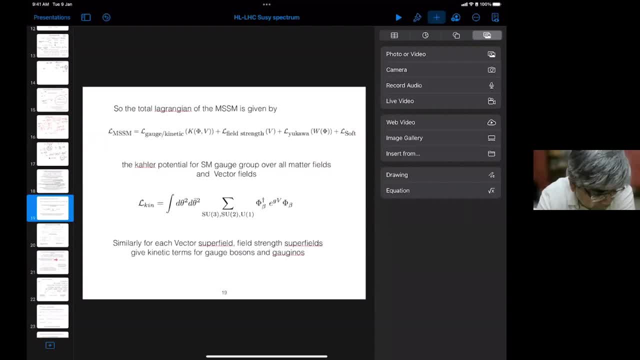 is exactly like the gauge bosons get masses, the gravity nodes get masses. gravity nodes get, become massive in a super gravity theory. so that is the case of a local supersymmetric theory. thank you, yeah, uh, any further questions? uh, any further questions? okay, so, um, uh, okay, i'm here, so 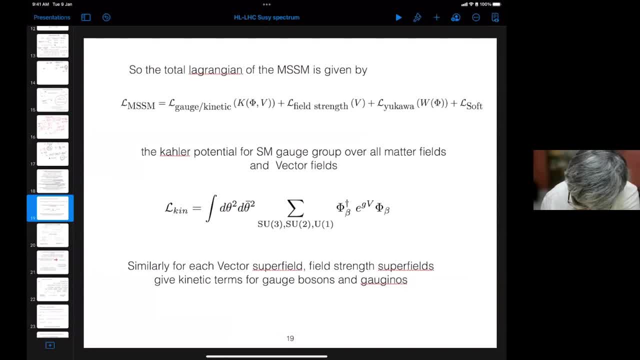 so, uh, now what we'll go by each term, essentially. so here, uh, the important main difference is: uh, echo couplings come from the standard, aquesta couplings come from a w, which is fine. what we have to fix is the more more complication is this one, because now we have some more, all possible gauge groups. 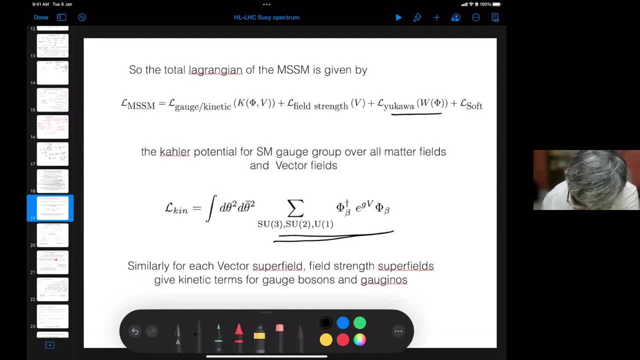 okay, so essentially you have s3, s2, u1. all of these kind of terms will appear in the exponential. so you call all the groups on the right hand side: okay. on the left hand side there are some gauges exponential. so when i do the sum, it doesn't mean it's an individual sum, but it's sum over the g. 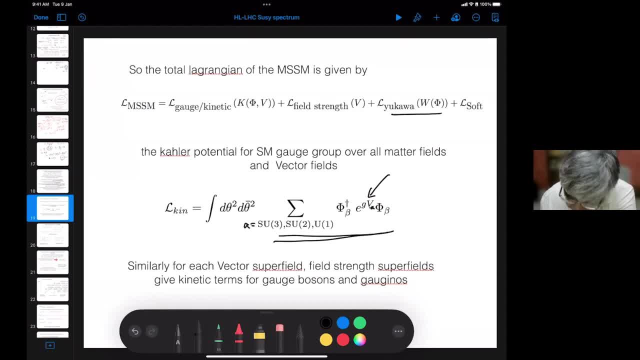 okay, it's only sum over a. okay, so g a. so i didn't write this equation properly. okay, so this is g a v a sum over g a v a. so you're summing over all possible. a is equal to su3, su2 or u1- all the three gauge interactions of the standard model. 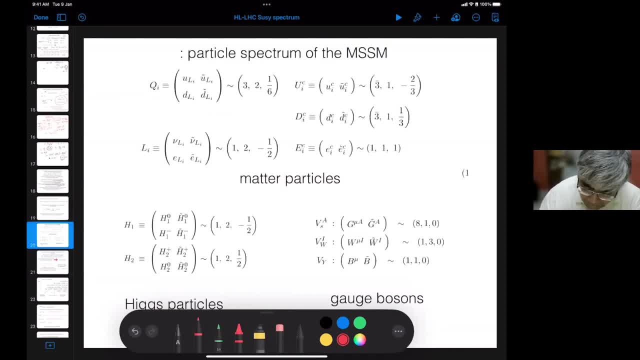 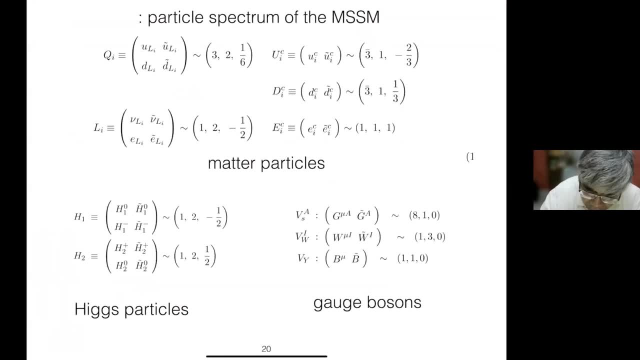 okay, so the particle spectrum, the particle spectrum of the mssm, the matter particles. the matter particles are essentially for every, uh, like i said, for every, because standard model is a chiral 3, anyway, you have this su2, uh uh, chiral theory. so the 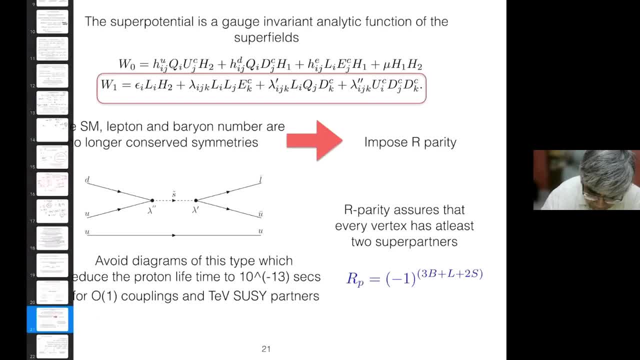 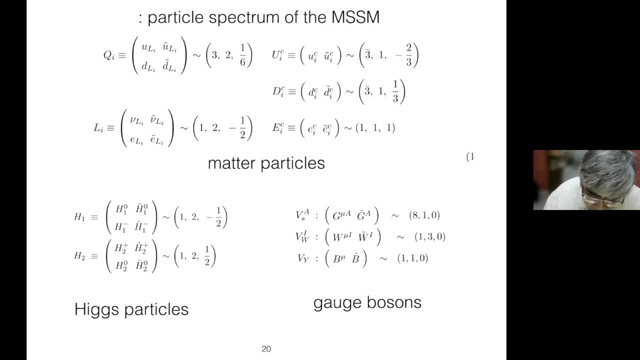 acitu. doublets are essentially divided already already into this part. essentially you have ul and dl and correspondingly you add ul, tilde, dl, tilde, ul, tilde, dl, tilde, and and the right-handed part, c. the c notation has come automatically here, the c is just the conjugate, is just the conjugate here. 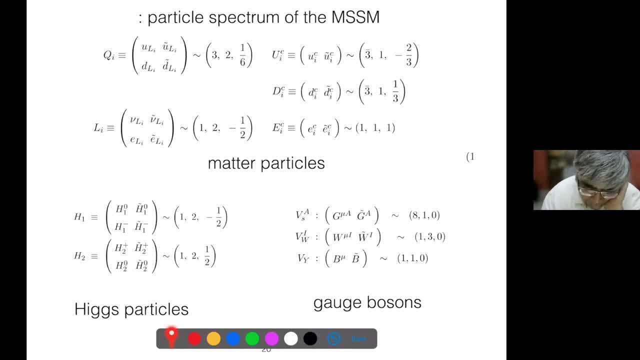 okay, so, and so for the leptons also. you do, and you add it over all the three generations. this is all multiplied by three. i is equal to one, two, three. so you have all the three generations with these representations. so the nomenclature is: these are called squarks, these are called 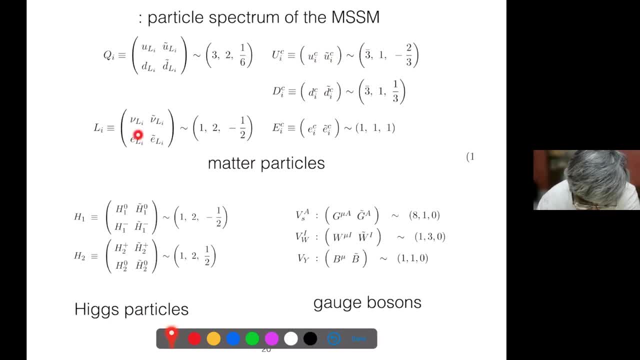 also squarks, right-handed squarks, left-handed squarks, left-handed leptons, right-handed leptons, and the super partners are called squarks here, and these are called slept ons, sleep tons, quarks and leptons, quarks and leptons. okay, s is there in front, essentially. now for the higgs particle. it interchanges, so for. 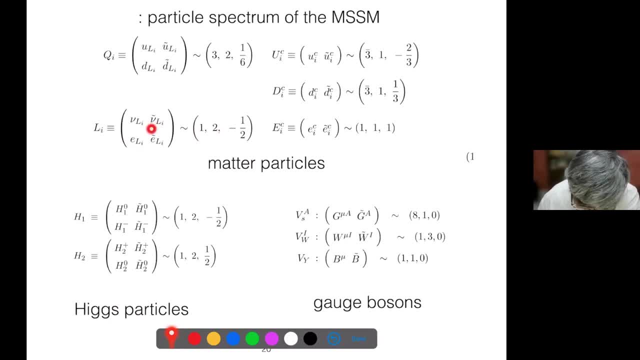 every standard model form. you added a spin half, spin zero particle for the higgs, because it's a spin zero particle. the higgs is the actually the scalar particle, whereas the tilde tilde is a spin half particle, as a superpartner is a spin half particle. so these are called enos. so these are called higgs enos. 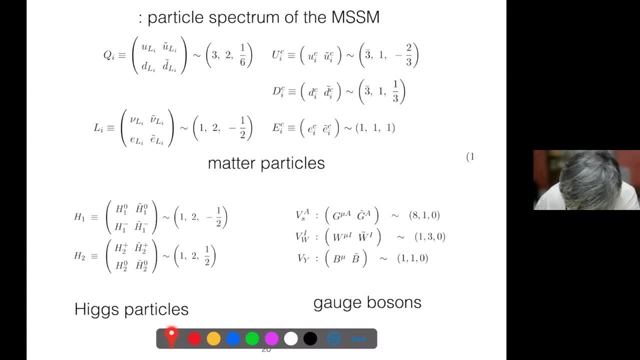 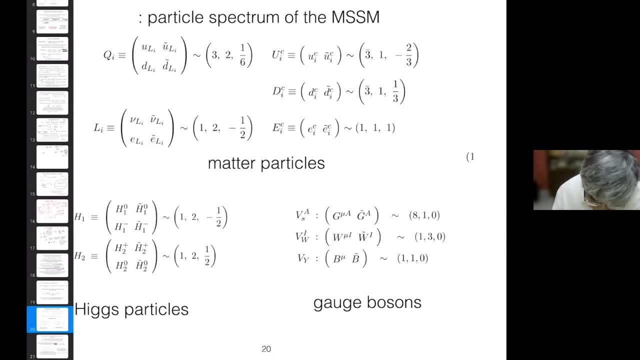 you need it. you need two higgs to give masses for both up and down type particles. the reason is again simply you cannot write five star. you cannot write five star within stand model, so for the uptake particles you need to add a separate higgs. so you add a separate. 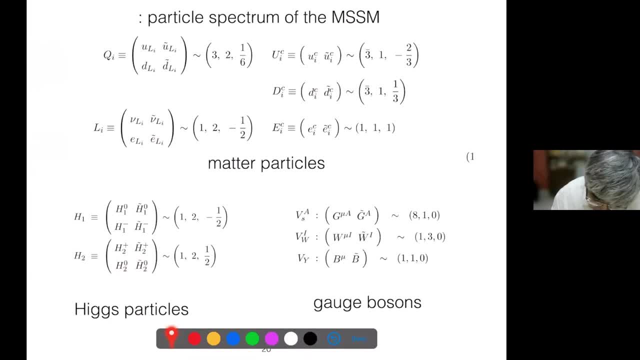 higgs here. for the up type, particle recall couplings okay, and for the down type you add a separate because you cannot write i sigma 2, 5 star, like we do in standard model to give masses to the top quark, so you have to give the same mass. i mean you cannot use the same higgs. this 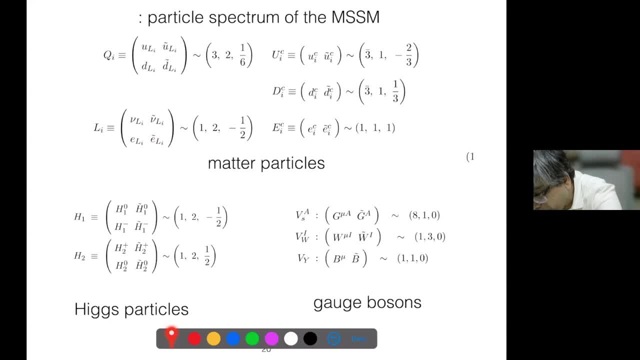 is the problem with supersymmetry, not with su2, because within su2 you know that two and two star are the same. okay, but within supersymmetry, two is allowed but two star is not allowed. or two star is allowed or two is not allowed. so you take two, uh, the doublet and the. 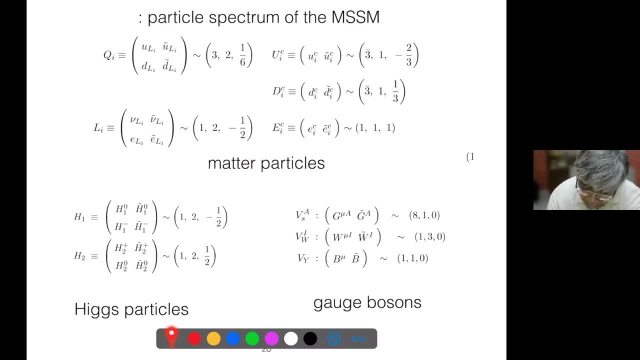 doublet star. you use it as, uh, as a separate field. actually, the doublet star, you use it as a separate field. then you have the three gauge bosons, gluons and the gauginos. we know vino, vinos are two of them, uh, three of them, and gluinos are eight of them, eight kinds of gluinos. 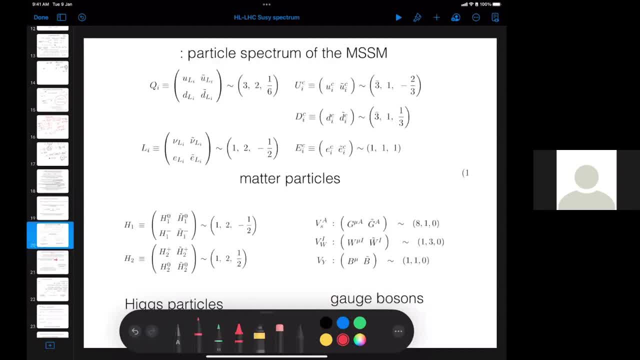 so, professor, uh, i think, uh, ritesh wanted to comment. some has a comment that the second tablet cancel the card. yeah, pardon, ritesh has a comment on the chat box which says yeah, so, uh, okay, i think he is mentioning about anomalies. i don't, i didn't see. i cannot let me see the chat. 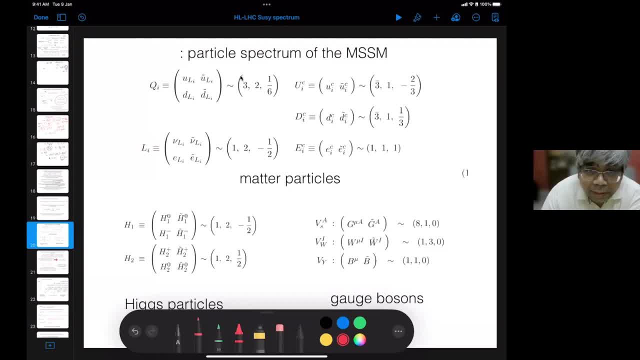 can you go ahead? yes, yes, yes, right. what he's saying is correct, because the if you the fermions, all the fermions, if you take the anomalies of all the fermions, um, if you need to cancel the anomalies- because with one set of anomalies you won't be able to cancel all the anomalies- you need a worth a set of fermions to cancel all the. 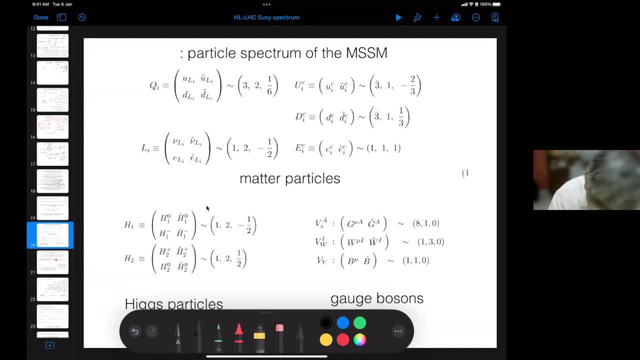 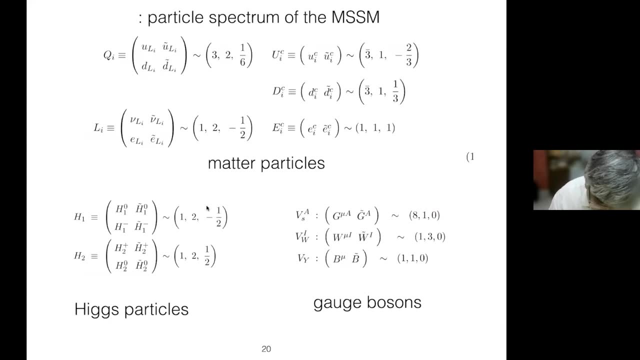 anomalies: the carol anomalies, current anomalies. cancellation also requires two hex doublets. that's an important point to note. thank you for telling us for machines. okay, so this is your higgs particles, this is your gauge boson. so, consistently, if you want, you need at least two higgs doublet models. two exists within. 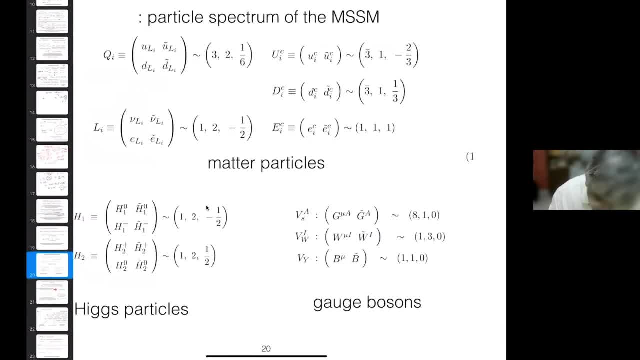 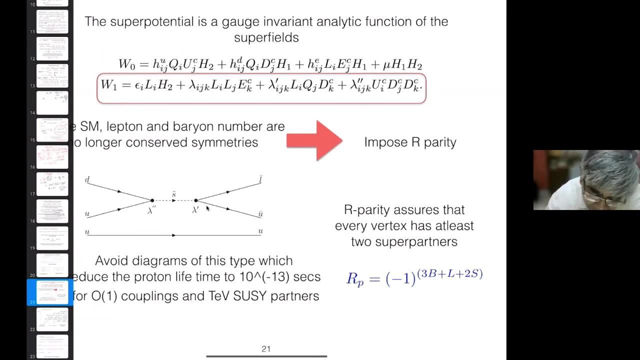 the um, mssm, the minimum number of higgs you have you can have is two hits, because if you want to replicate- and maximum number is your choice- you can do whatever you want. okay, you can do many things. so in addition, now let's come to the w. now the w also is a bit complicated here, because now the 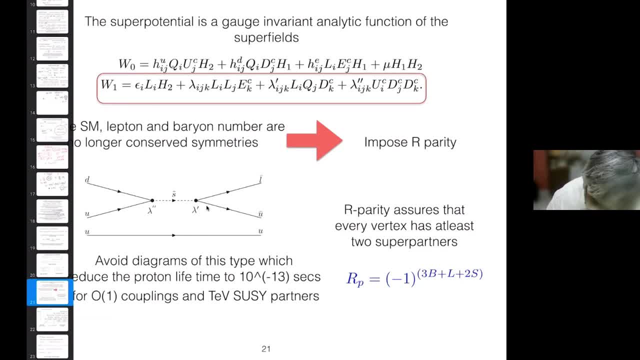 higgs and the fermions are on the same same footing. the higgs and the fermions are on the same footing. so, especially because the l, this l and this h1 carry the same quantum numbers, earlier you can distinguish these two because their spins are different in different standard. 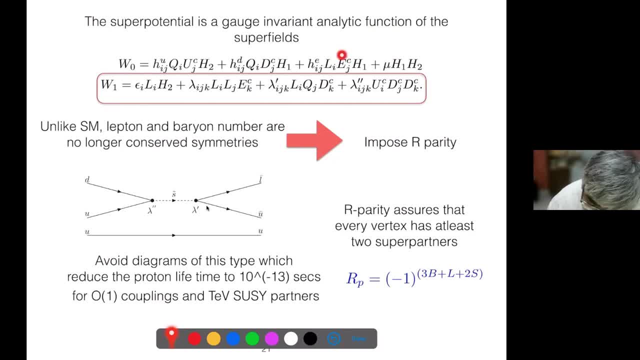 but now the chiral super fields. they carry the same spin, meaning they're all like there's nothing distinguishing between a l super field and h1 super field. so wherever there is an l or a h1, okay, wherever there's a h1 you can replace it with l, say, for example, this: okay, so here you can put. 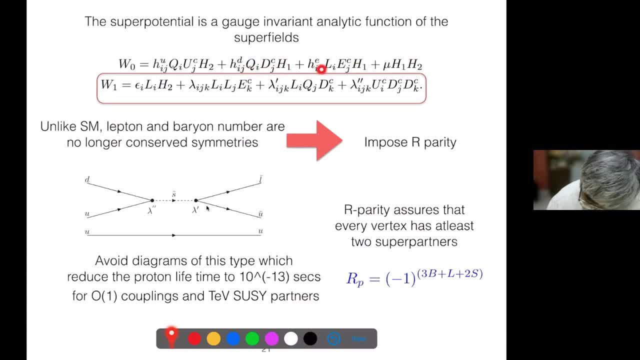 uh, lqd. okay, this is l, l e, this is li h2. so you can write these three terms just by replacing h1 with li. okay, similarly, you can also combine all the three: uh, what do you call fermionic, right-handed fermions, right-handed fermions, and form a c? uh, use, transform as three. 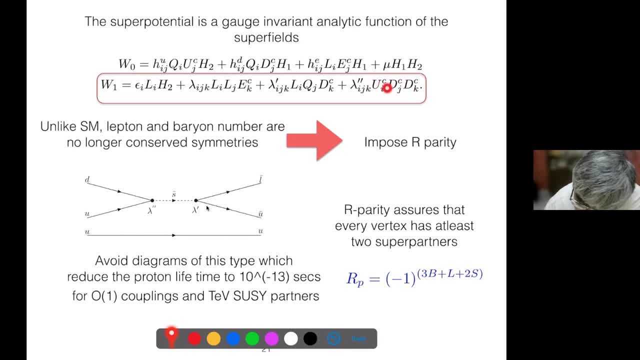 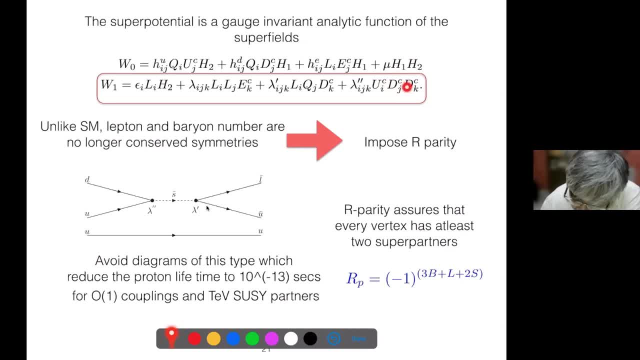 okay, but within the, within supersymmetric theory, this is possible. so these three terms, because they have the same spin, okay, their spin is irrelevant in this case. and these kinds of standard model and supersymmetric standard model, They all have so-called, they're all chiral representations and the maximum number of chiral representations which you 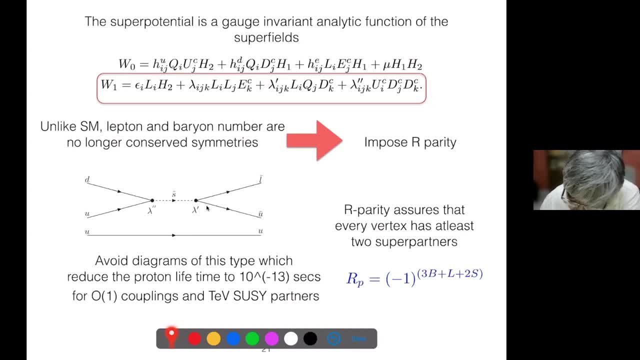 can add within them to superpotential is three fields, So 515253.. 51525354 is non-renewable. If you want to add non-renewable interactions in supersymmetric theories you have to have at least four superfields. So if sticking to renowable supersymmetry, you end up having 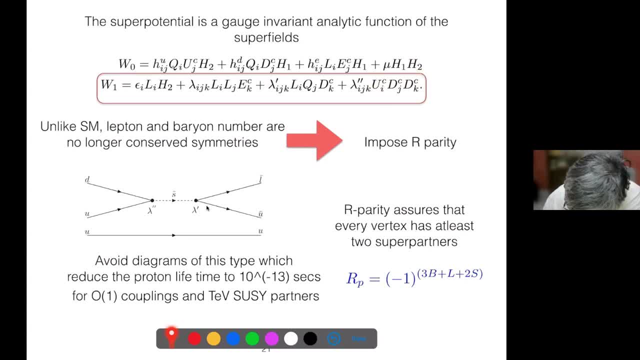 three superfields. So this is completely allowed. But the problem is all these terms breaks, lepton number and baryon number. So it can be easily seen that there is one lepton number breaking Here. there is also a lepton number. All of them, all these things break. 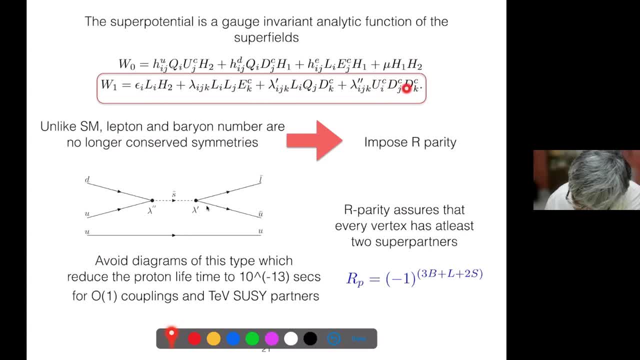 lepton number by one unit and this also breaks baryon number by one unit. So baryon number and lepton number, when they are broken they give to fast proton decay. So you can have diagrams. So for example, here there is a lambda prime coupling and then this one would give me And 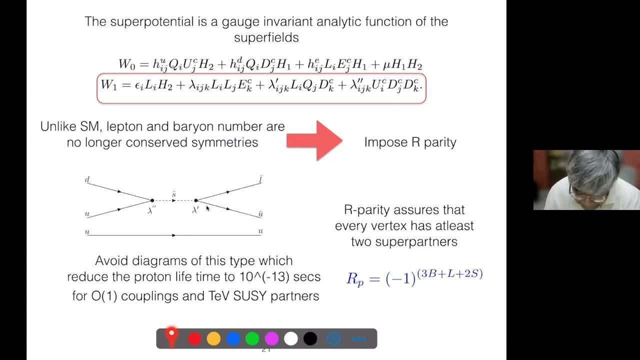 if supersymmetry is of the order of, say, 1 TeV, so you should be decaying very, very fast. Every one of us should be decaying very, super fast. actually, We shouldn't be surviving so fast. So proton will no longer be stable and the lifetimes are of the order of 10 power. 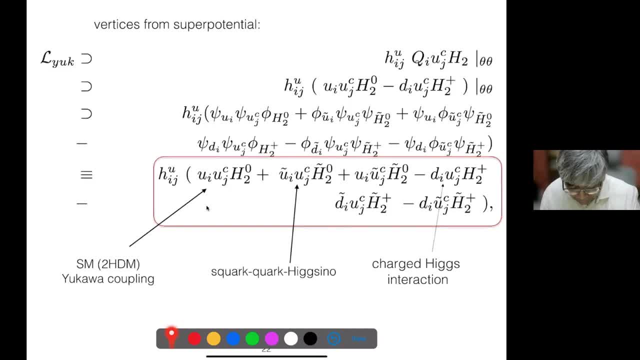 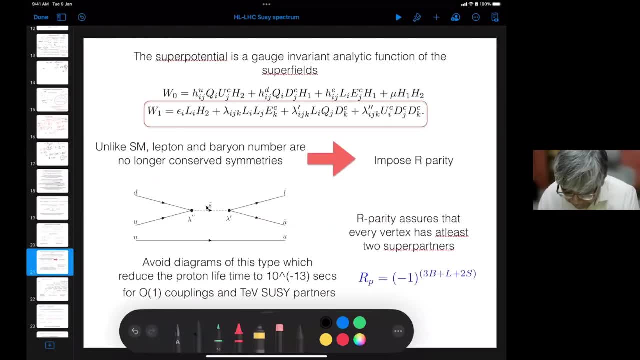 minus 13 or something. If you have order one of this coupling, order one charges. I mean, these couplings are of order 1.. And if you have a TeV scale, supersymmetry or something- Now to avoid these terms, in the super potential in MSSM, what one does is imposes some symmetry. 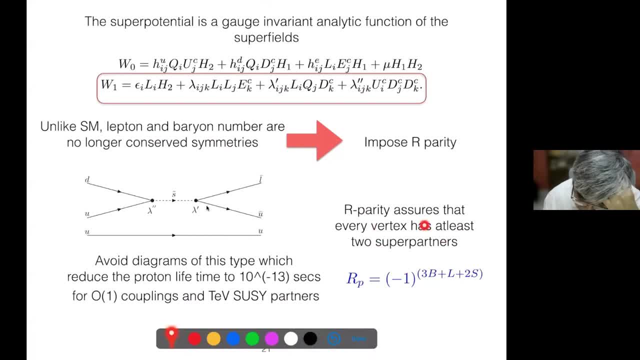 called R parity. It is just some discrete symmetry given by this particular formula depending upon the baryon and lepton number of the individual fields. So imposing this baryon and lepton number conservation. so this is like explicitly in working video on a little left-hand number in new york. 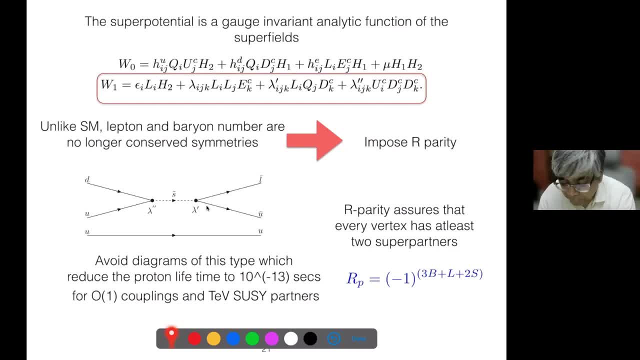 theory. so you say, okay, in the standard model these are accidental supersymmetry symmetries. once you go to mssm, these symmetries are no longer valid and they give you order one, correct? i mean really order one coupling constraints, because these are completely unconstrained. 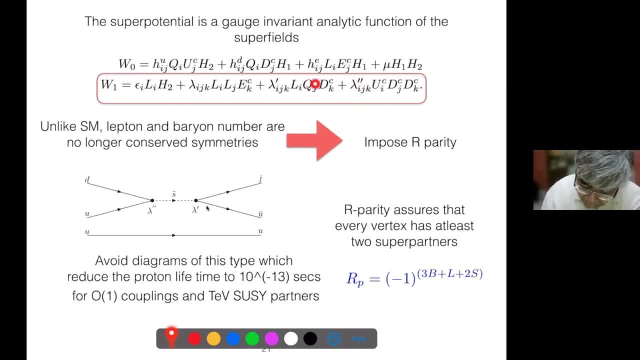 except from proton decay. okay, these are completely unconstrained. of course there are a lot of phenomenological constraints. what i mean to say is, theoretically they are completely unconstrained, so they can be order one phenomenologically they have a lot of constraints. actually they have uh, neutrons w beta decay, they have all these neutrino masses, so on. so, and here the product. 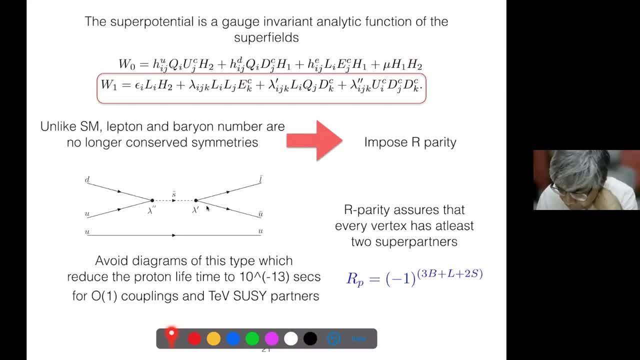 of these two will have proton decay constraints and so on. so so with this, uh uh, okay, you can say them. they are not order one. they can be. they can be very small and so supersymmetry is very heavy, so you can organize it. there is only one coupling. not all of them are coupling. 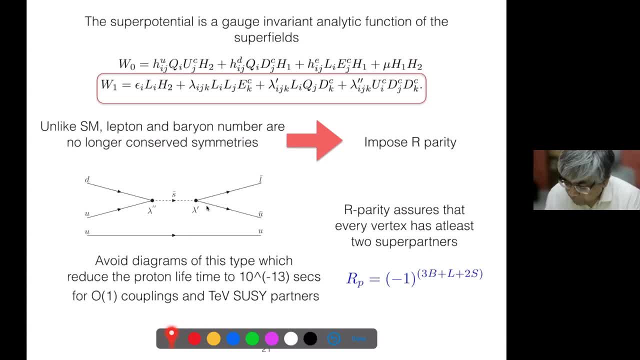 there you can build some symmetries with individual lepton numbers or some complicated z and symmetries or something, so that you can allow only one of them. so that is a different ball game. that is a huge game one can play, but as far as we are concerned we'll just impose this r parity and so 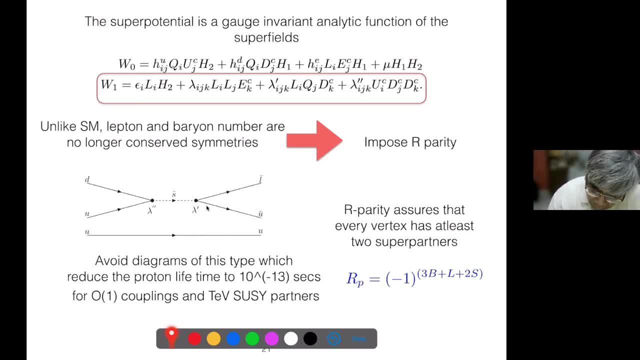 this rules out w1, all the terms to goes to zero. all those terms go to zero and imposing our party. what does it do? it is a symmetry- not because it's very one- and lepton number and also the spin of the particle. so what it does is it distinguishes super partners with partners. so it distinguishes super partners. 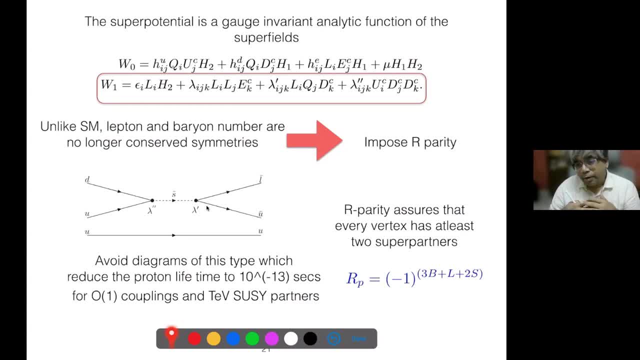 with partners. so it automatically tells that all the partners and super partners are separately concerned. in a way, quote unquote, it conserves the uh super partners. there is some sort of super partner number source, in a way it's like. it's like some sort of a discrete symmetry which protects the super 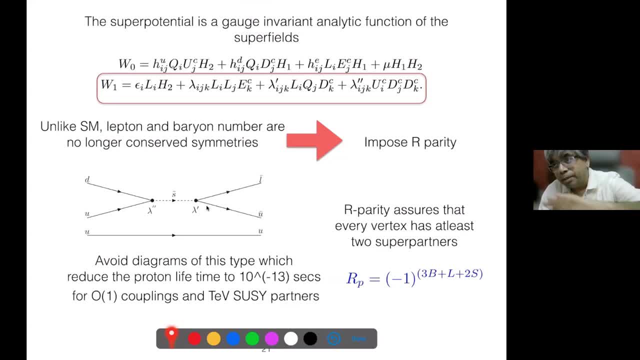 partners alone. so the lightest of these super partners is completely concerned. it's like: imagine that you have a baryon, number or something. the lightest baryon is always conserved. similarly, imagine that this is a r. parity is like something. it's like a very number sort of thing. 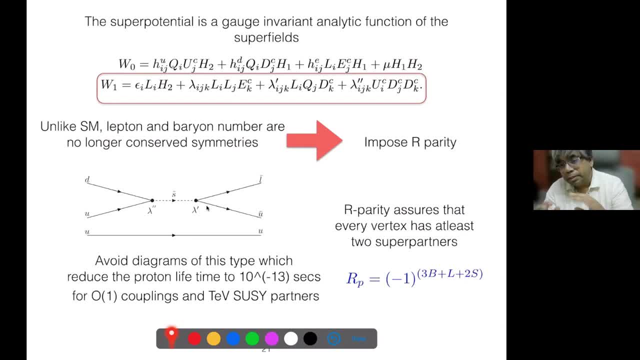 but it's not baryon number, but it's something. so the lightest of this, it's a symmetry which protects all the super partners. so all lightest of the super partners, just conserved, okay, and that is the result of this symmetry. so the lightest of the superpartners, which typically 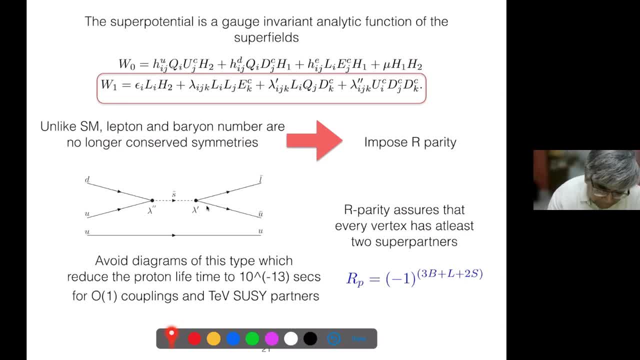 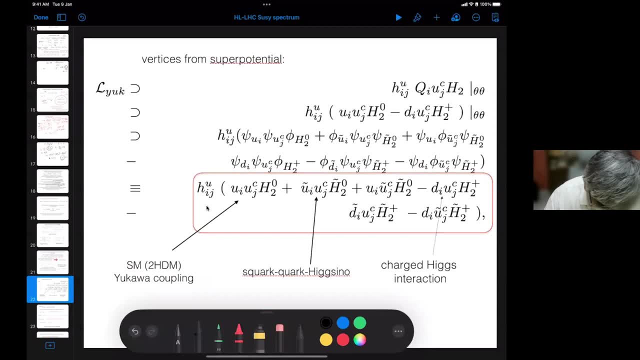 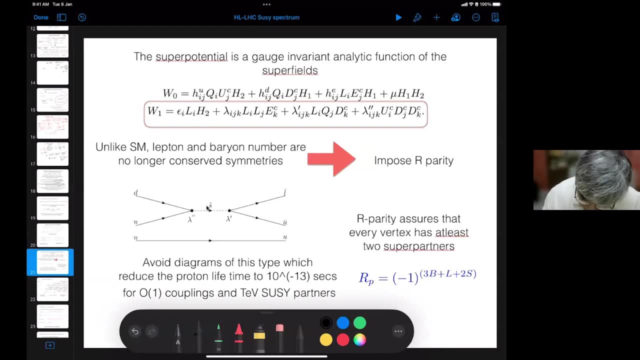 happens to be a neutrino. we'll come to neutrino in a second. actually, okay, oh my god, i'm having trouble with this. so let's look at so. for the present, we'll just forget about this entire set of terms and impose this r parity, and we'll say the lsp, the lightest. 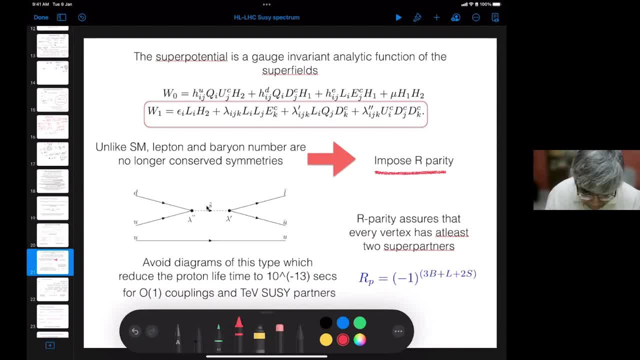 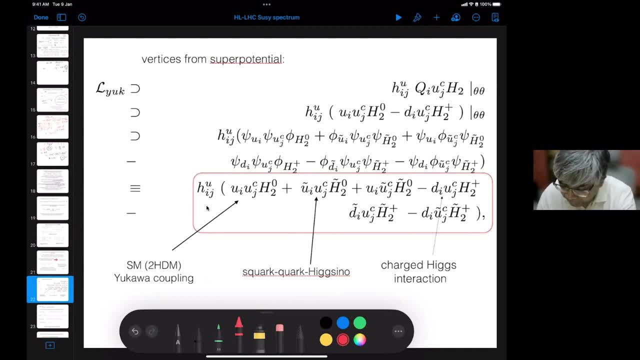 supersymmetric particle is concerned is stable. so let's look at the all possible terms, just like in qed, what we did for supersymmetric qed. so you look at a term like, for example, the most dominant coupling, which we like, and the one which has significant implications on all the 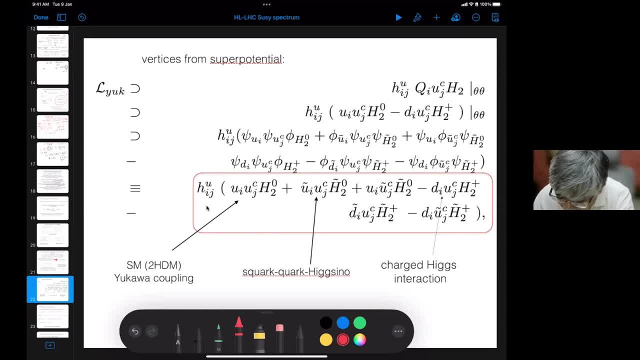 phenomenology is the top core coupling. so we'll just look at the top core coupling. how does it give you the top core coupling? is this one? this is the top core coupling. okay, so when you derive this thing, you mention the top quark. it also gives you the you call mass of the top quark. 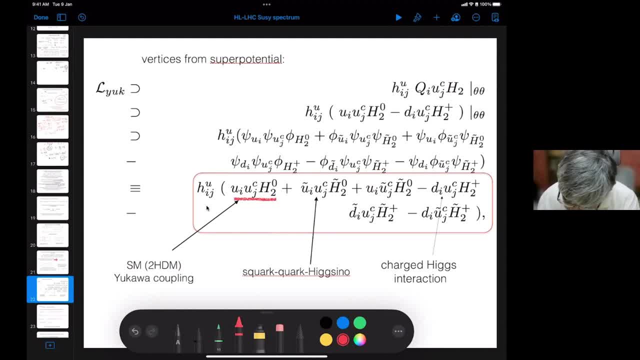 it also gives you: stop stop higgs, you know. okay, top stop higgs, you know, and also that this kind of things. so these couplings play an important role in other things. actually, okay, and this is your top quark, okay, and then these play charge leaves interaction. 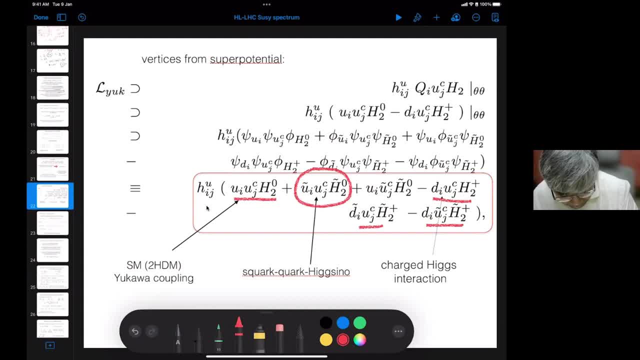 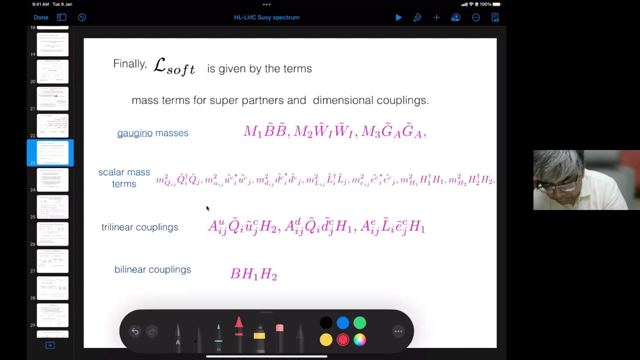 these are your charge leaves interactions. okay, so these are your quark couplings and kinetic parts. like i said, they come from the killer potential as well as from the w potential. okay, the super field. so let's go through. um, the superpartners. okay, all the mass terms for this. uh, the last unknown term, which is the soft term. the soft term, the. 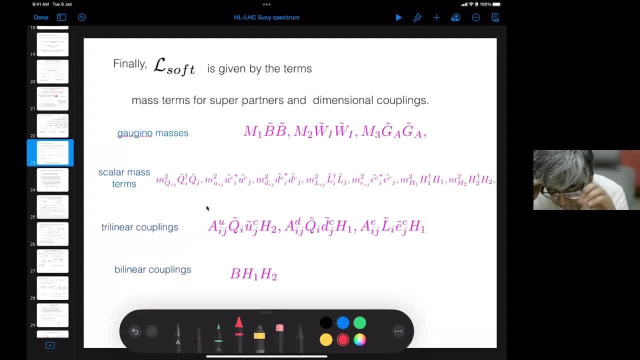 soft potential is supersymmetric breaking. terms which i said, which are resultant from soft supersymmetric breaking, all the let's list out all possible terms which arrive from supersymmetric breaking spontaneously and we don't know how they come, but they are there in the lagrangian. that's the. 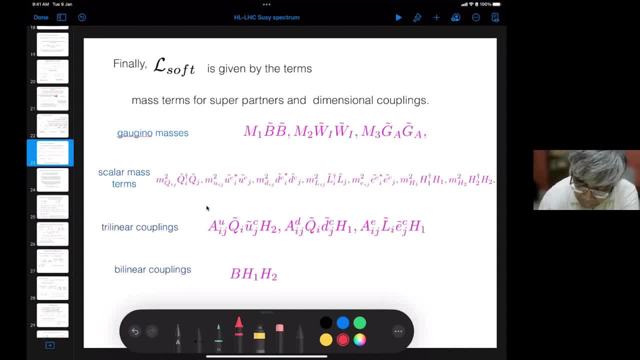 basic point we are going to do so. let's list them out. so these are masses for the gigianos. now the there is a thumb rule to remember what these terms are. okay, so the thumb rule is that the main implications of supersymmetry is that it insists. 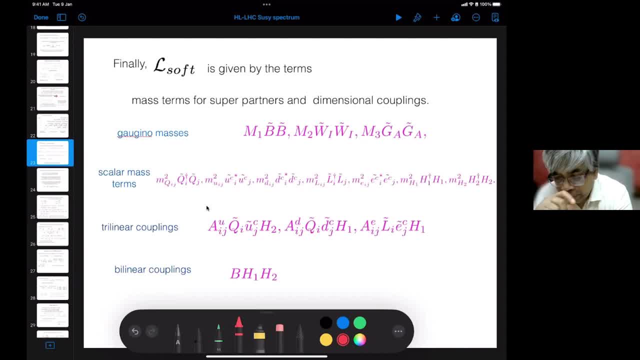 on equal masses and equal couplings for uh particles and their super particles. so since we cannot change the masses of this, so if you want to break supersymmetry you have to break the masses or the couplings. okay, since we cannot change the standard model masses and the standard model couplings, we change. 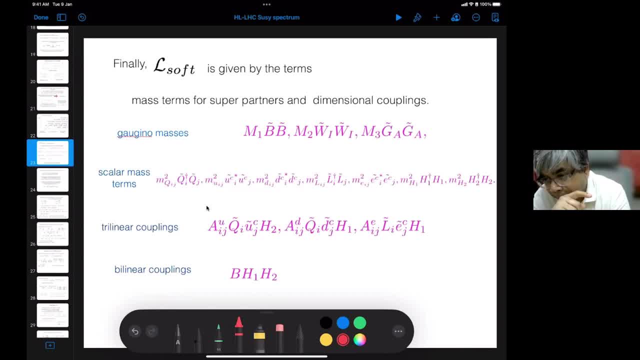 the couplings of the superpartners and their masses. so what we do is we add extra mass terms, mass terms for all the superpartners, because then your supersymmetry is broken. if the supersymmetry is spontaneously broken, all the superpartners will get an extra mass term compared to the what does? 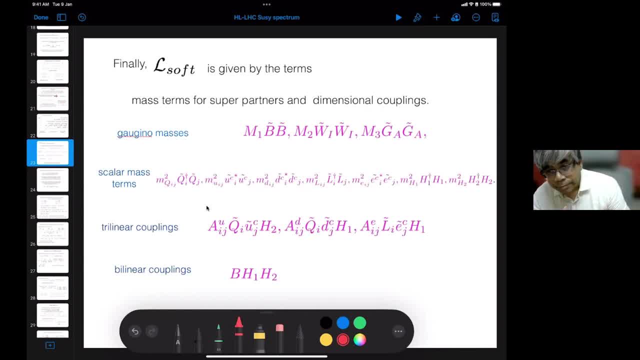 they have already coming from the standard model mass terms. so standard model mass terms are essentially m e square, m u square, like what we have seen right, for example, m e square, m u square, and like we have seen in the qd example, the electron and selectron will have the same mass. 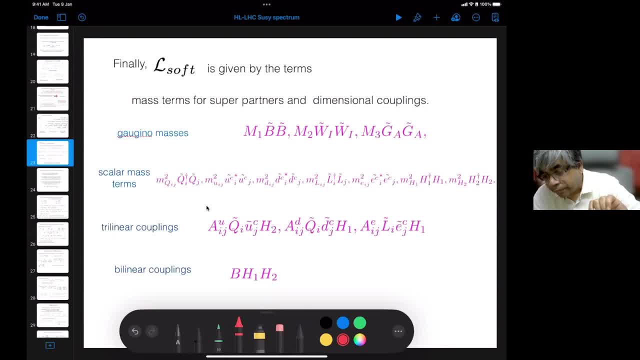 as long as supersymmetry is concerned. but in addition to this, if the selectron is given an extra mass, then supersymmetry is broken. similarly, photon and 14o have the same mass, but in addition to the mass which is, say, zero, say, for example. but if i give a mass to the 14o, then supersymmetry is. 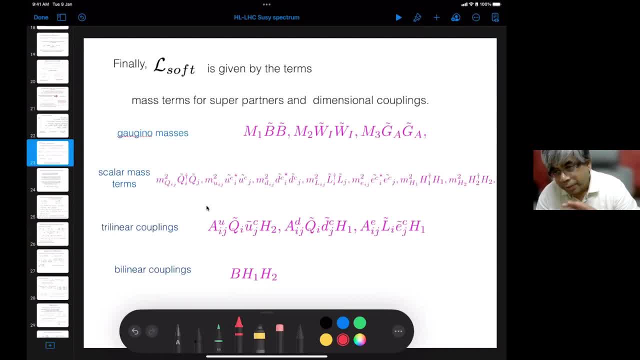 broken. okay, so that is the basic idea. so what we do is we add mass terms for all the 14os or all the gauging. so this is the gluino, this is the vino and this is the vino. all of them have their mass terms. 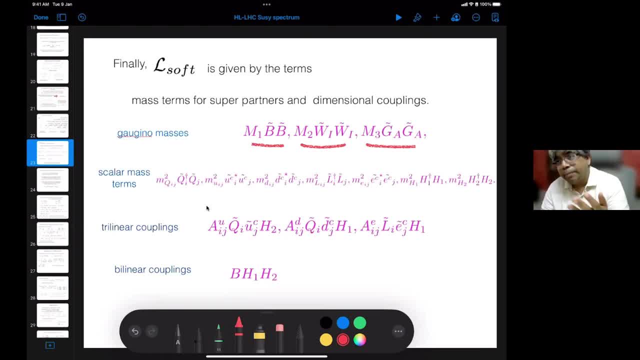 and then similarly for all the matter, receptor particles, the scalar particles, all the scalar particles are essentially your squarks and slept arms. so the squarks and slept arms get their masses. okay, now here comes the interesting part. in addition to this, the higgs mass terms also come as a supersymmetric breaking part. 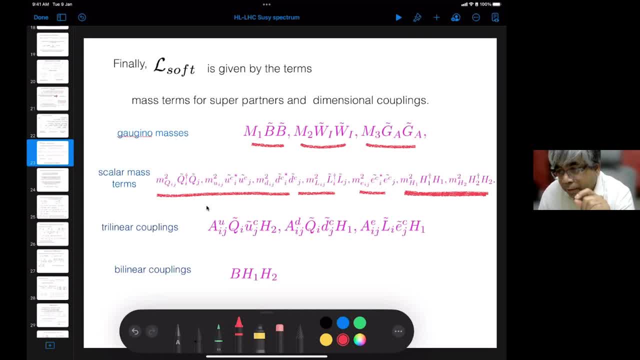 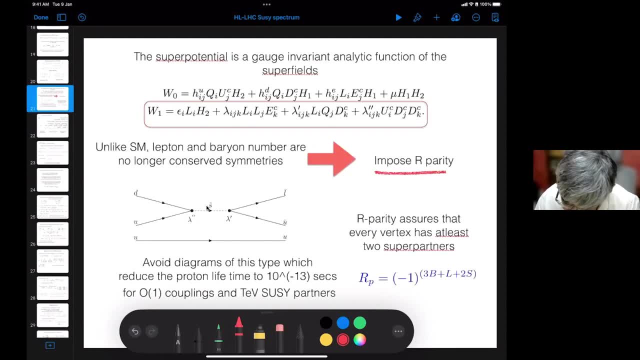 okay, the supersymmetric conserving higgs mass is only something called the mu term, this term, this is only the supersymmetric conserving higgs master. but we have to break supersymmetry, so we add mass terms for the higgs part of the scalar particles. okay, m square, h square, essentially. 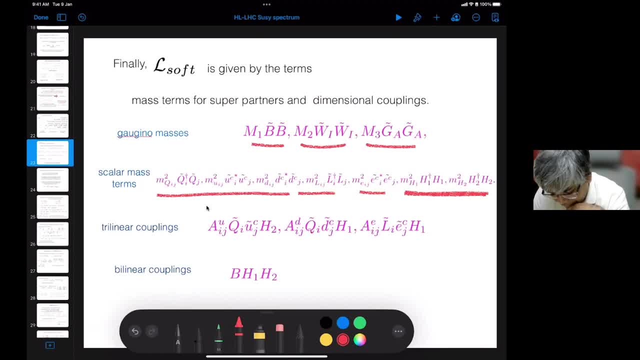 now, okay, so this comes here. okay, these are the higgs mass terms. okay, m square, h square, which are supersymmetric breaking. so higgs mass terms, though they are standard model particles, this is not strictly standard model, because in standard model we only have one higgs. but imagine that the real lagrangian is the supersymmetric lagrangian. 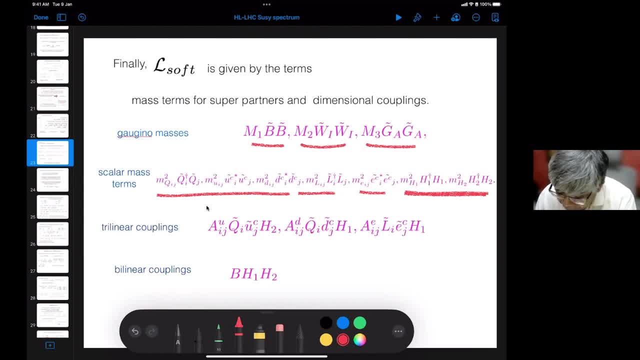 so the higgs mass terms are also part of the supersymmetric breaking, lagrangian, not a part of the standard model. lagrangian or ms's and lagrangian, so is he conserving? then we add extra couplings, extra couplings. we cannot add extra gauge couplings. okay, if we can try. 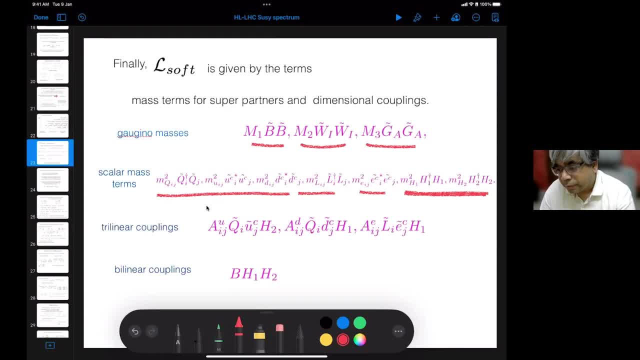 to add extra gauge couplings, then you have to change the gauge theory so you don't break the gauge symmetry. you don't break the gauge symmetry. the gauge symmetry is broken like in the standard model. because the breaking of the gauge symmetry is very, very, uh, complicated, because a tremendous 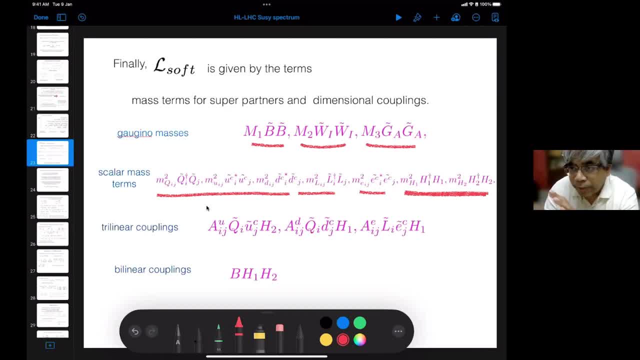 number of experimental results will get modified. so you don't want to modify anything with the gauge symmetry. but the thing you can modify is a ucava couplings. okay, so for the ucava couplings you add extra ucava couplings. ucava like couplings to the supersymmetric partners, made up of only scalars, say for example: 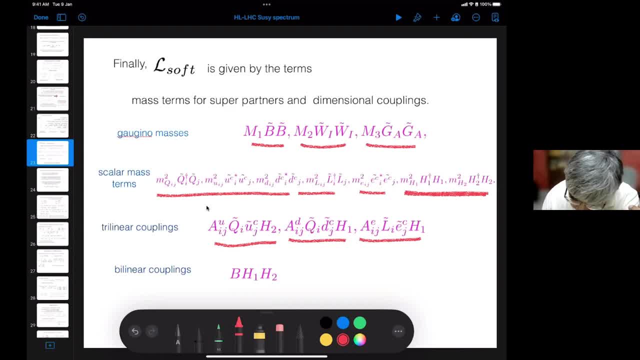 selectron select uh, squark, squark higgs, squarthorpe higgs. selectron selectron higgs or selecton selectron higgs. so and so, these are the extra couplings which you can add them. finally, you can add a higgsino. 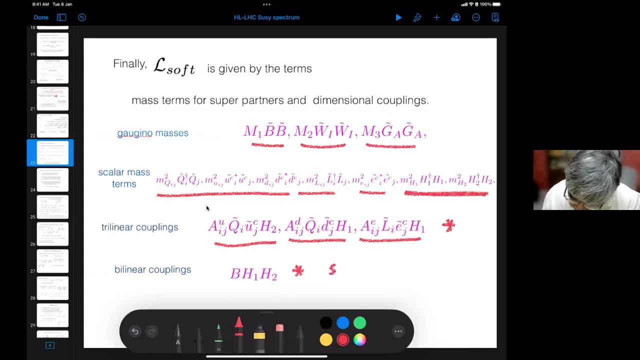 okay, this is a higgs. higgs, so this is a linear term, this was a scalar term which also breaks, which also breaks. now, yeah, you can. um, okay, so so far for all the supersymmetric partners. okay, where higgs is also considered as a part of supersymmetric partner. essentially, you added: 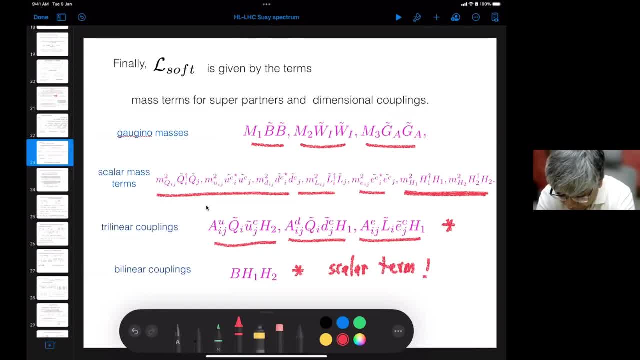 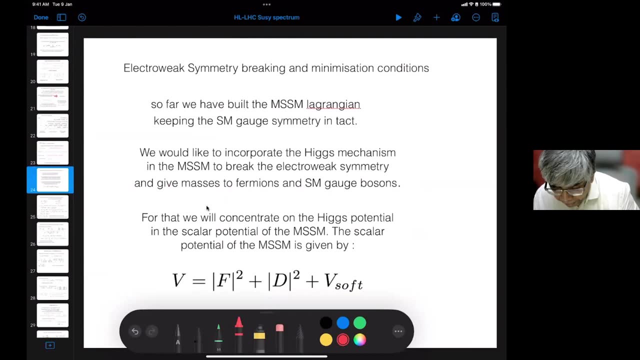 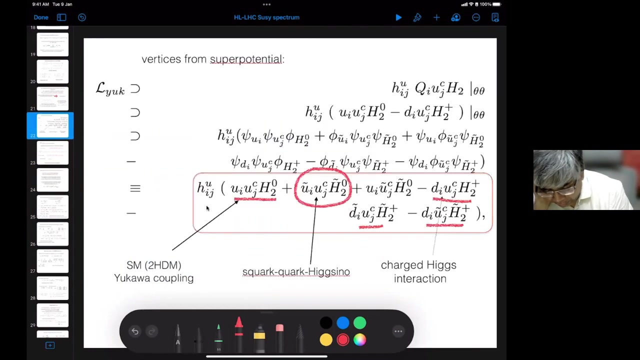 uh, extra mass terms and extra couplings. couplings except for the Higgsian. except for the Higgsian. In principle, you can do it for Higgsian also, but this is a different theory actually. So now the point is that now you have built the entire Lagrangian just by following the 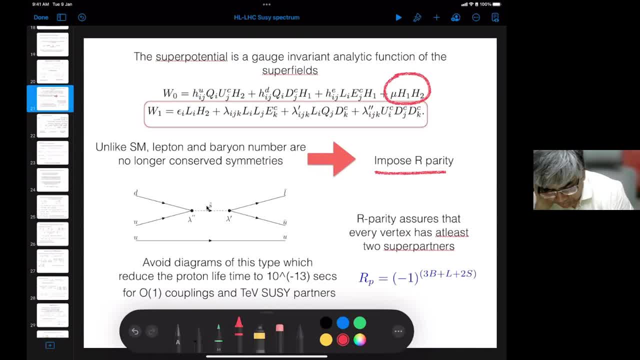 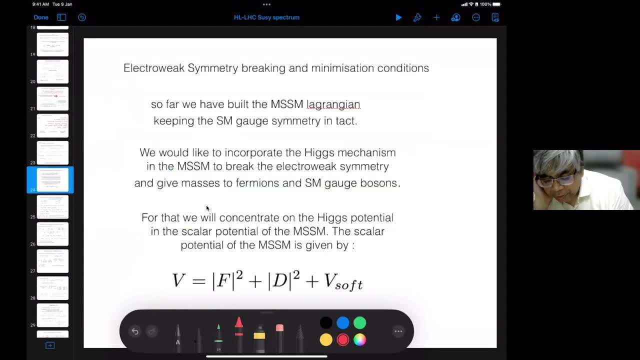 rules like W, K and tilde. you have built the entire Lagrangian. Now you also added L-soft. So far a suit across U1- symmetry breaking- is not broken. A suit across U1 is not broken. So that means you have to incorporate standard model Higgs mechanism also within the supersymmetric. 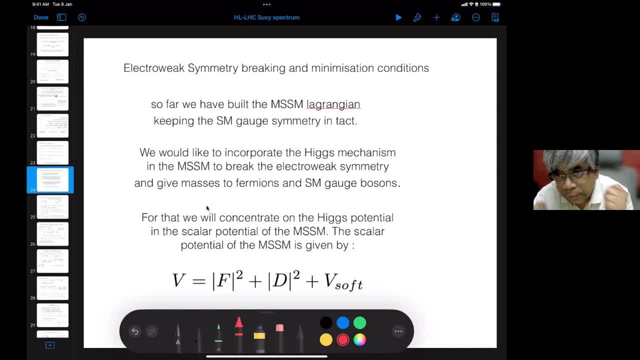 theory. You want to incorporate standard model Higgs mechanism also in this. So to do that you have to consider the full scalar potential, the full scalar potential of the Higgsian, The full scalar potential which is said F square plus D square plus. this is just the. 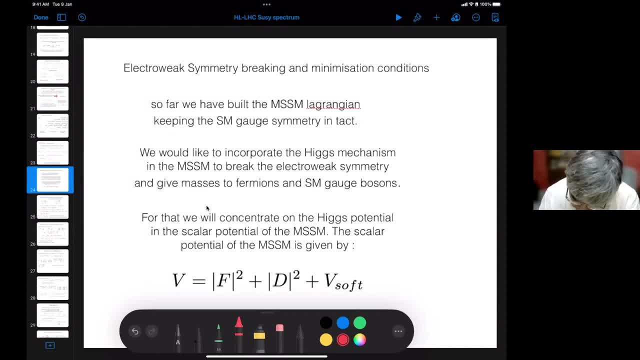 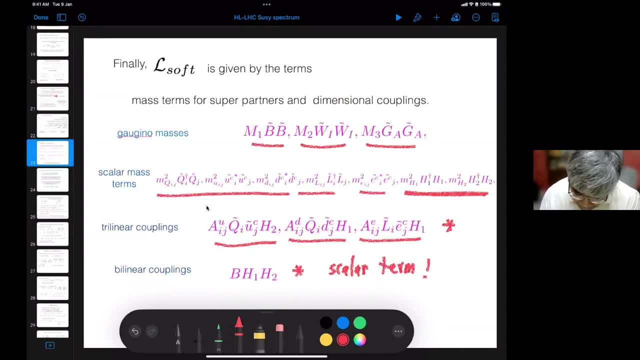 supersymmetric conserving part. Now, because L-soft also has lot of scalars, purely scalar part, the scalar mass terms, trilinear couplings, bilinear couplings, these are all part of V-soft. So all this should be added into the full scalar potential. and then we ask the 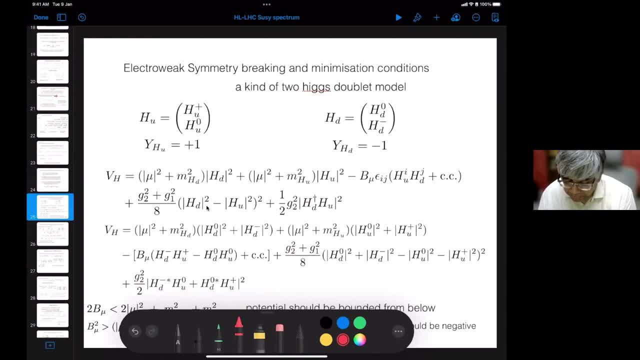 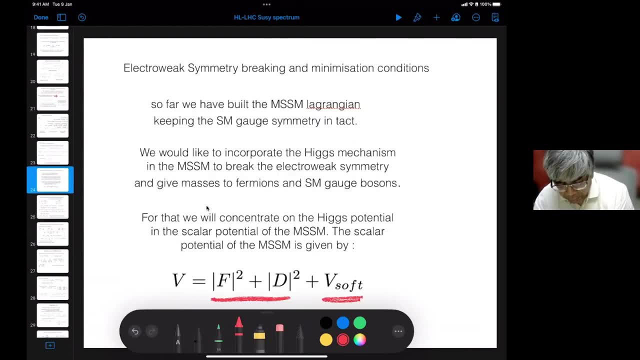 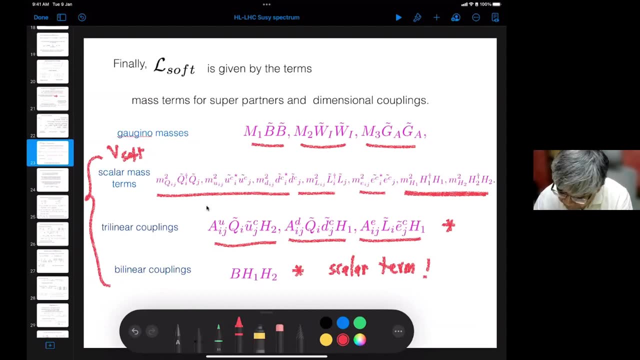 question: how do you minimize this? So, to minimize, you just consider it as a two Higgs doublet model. You don't worry about all these terms and everything except for the Higgs mass terms. So the only things which are relevant for us are, from the V-soft, the Higgs mass terms. 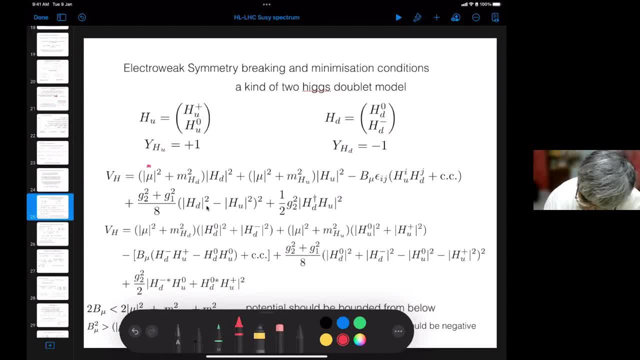 You have the Higgs mass terms and the supersymmetric conserving Higgsian or mu square terms. So the MHD, MHU, H2 and H1. I wrote this in different notation- H, sorry. I am sorry for this. actually HU is equal to H2, HB is equal to H1.. And then you write down only the Higgs part of the potential. 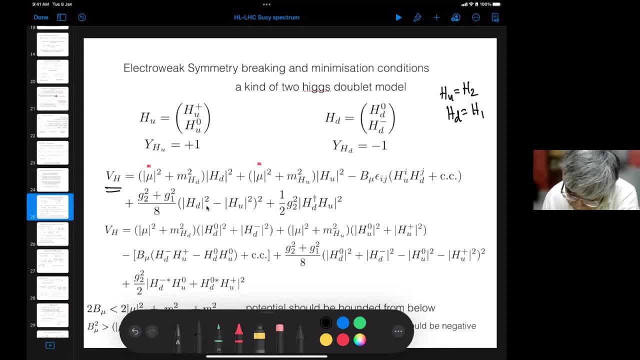 the scalar potential. Now this is different comment. This is an ordinary two Higgs doublet model, because in an ordinary two Higgs doublet model there are n number of quartic couplings. There are five different kinds of quartic couplings. 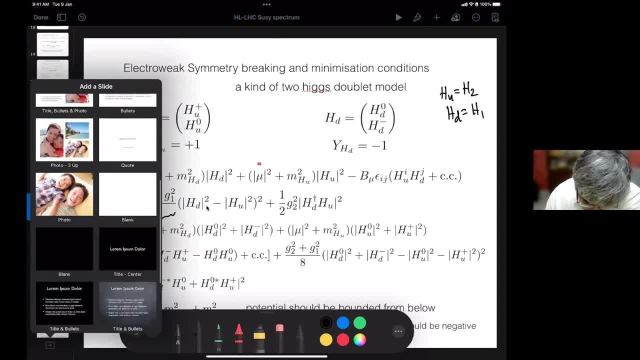 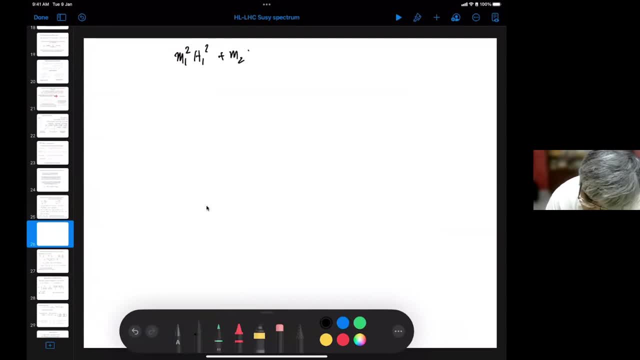 So just to in a two Higgs doublet model, a general two Higgs doublet model, you will have something like M1 square H1 square plus M2 square H2 square plus H1. star H2, M12 plus lambda 1 H1 H2.. 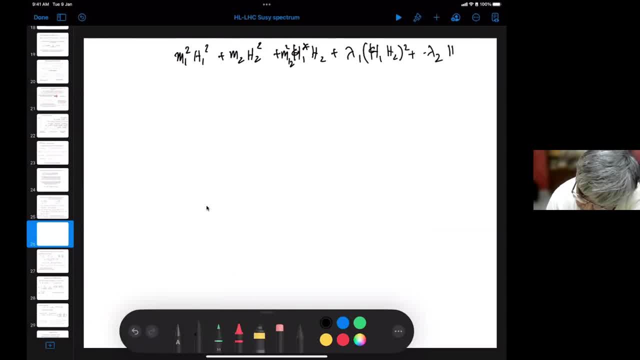 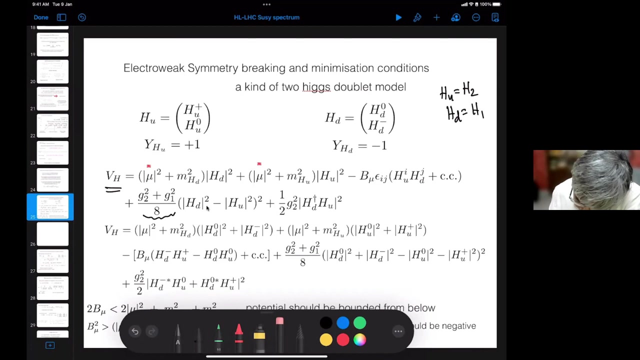 H2, whole square, plus lambda 2, H1, power 4, so on, so on. So there are five of these couplings. These are all free parameters. These are all free parameters, But this is not the case in MSSM. They are not free parameters. 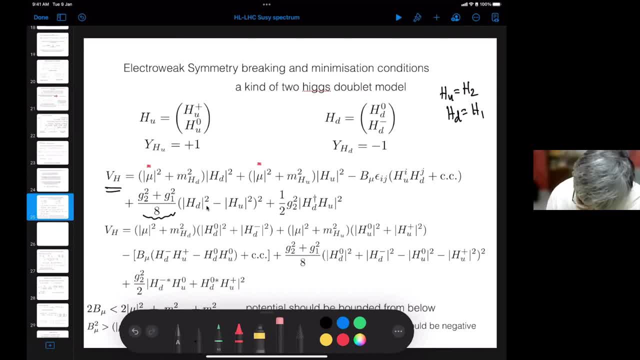 because this comes from the D term. This comes from the D term. The quartic couplings are allowed. Only one quartic coupling is allowed and that coupling is proportionate to gauge couplings And that coupling is proportionate to gauge couplings. 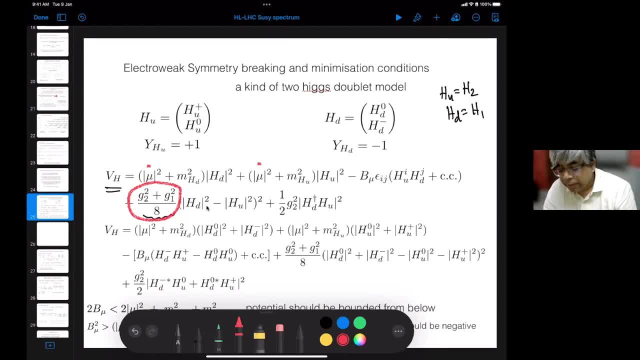 So there is only one quartic coupling. So this is an extremely constrained two Higgs doublet model. if you want that to, it's an extremely constrained two Higgs doublet model, And so when you minimize this, the answers are easy. actually, You only have two simple 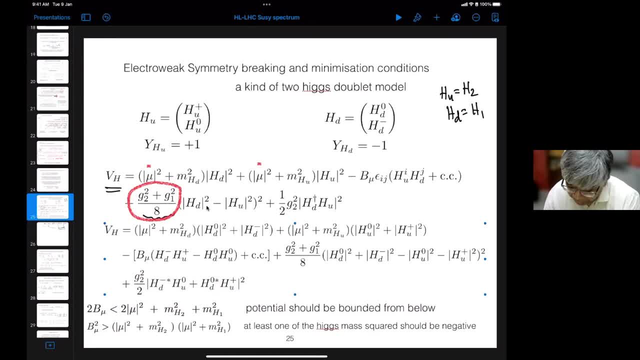 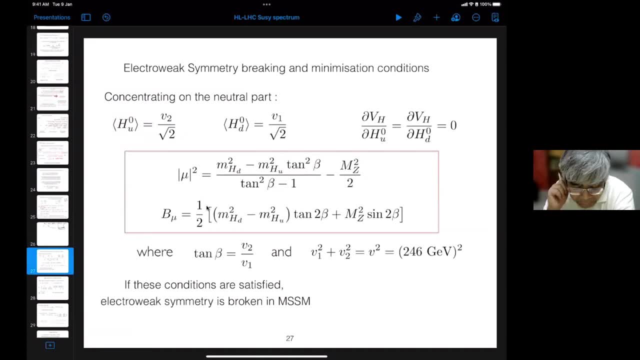 results. So you minimize this, You take the Higgs potential, expand it completely, take the neutral part and in the neutral part you assume some waves for the neutral parts. So V2 is equal to some V1 and V2- two waves- and use the minimization conditions and you 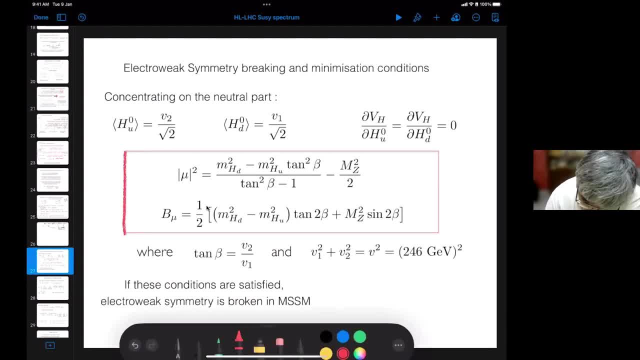 end up with two formula which have to be satisfied for successful electroweak symmetry breaking. So from this formula, what you get very interesting result is that. So you get a very interesting result. You get a very interesting result. There is an MZ square coming here, because MZ square is 1 by 4 G square plus G prime square. 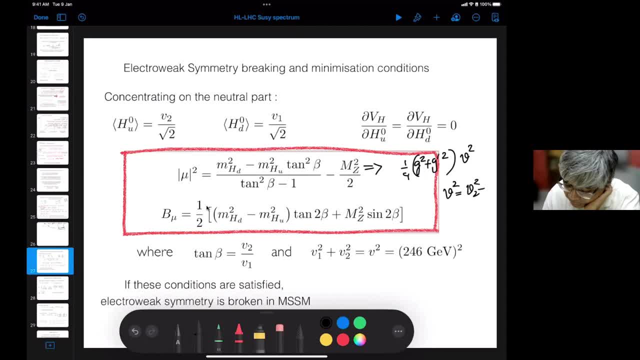 V square and V square is nothing but V2 square plus V1 square, or VU in our notation, VU square plus VD square and tan beta. here I have written. I have written here, sorry, tan beta is equal to VU by VD. 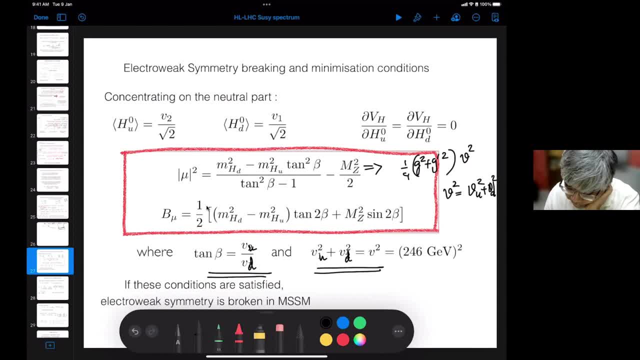 Now see this formula. this relates the supersymmetric conserving U square term with soft terms, meaning supersymmetric breaking terms and a completely irrelevant meaning. completely not irrelevant, completely irrelevant only. what I meant was completely unrelated quantity which is coming from standard model, which is MZ mass. 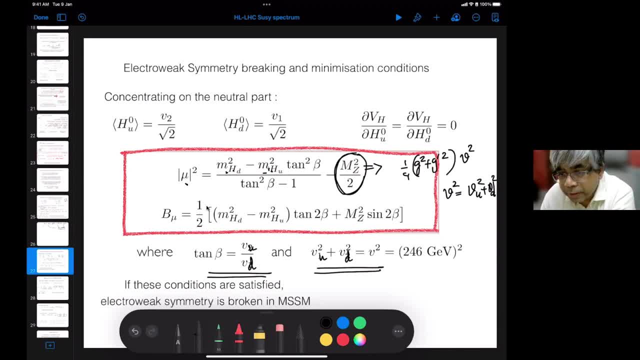 So this is the origin of all the entire fine-tuning argument in supersymmetric theory. this is the origin of all the fine-tuning arguments. So, but this condition, which relates a supersymmetric conserving mass with a supersymmetric breaking terms and MZ square- there is a minus sign here- is these two conditions, if they are. 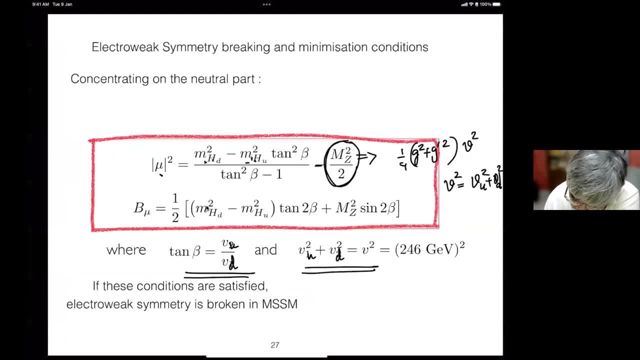 satisfied. this is called these minimization conditions. if they are satisfied, then only electroweak symmetry is broken away from the standard. So this is the origin of all the entire fine-tuning argument in supersymmetric theory. So the origin of all the entire fine-tuning arguments. 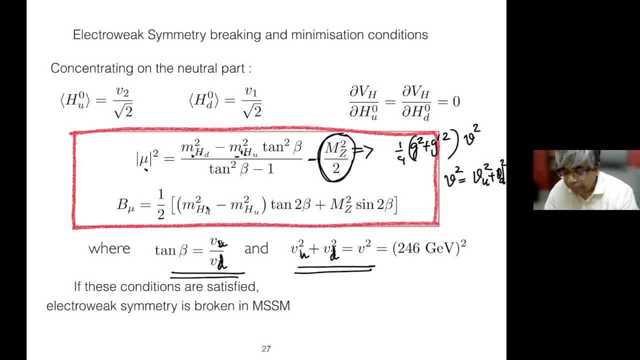 So if you had a supersymmetric sign model within the minimal supersymmetric sign model, that means you have implemented successfully the Higgs mechanism within a minimal supersymmetric sign model. only then, as long as these two conditions are satisfied: the minimal supersymmetric. 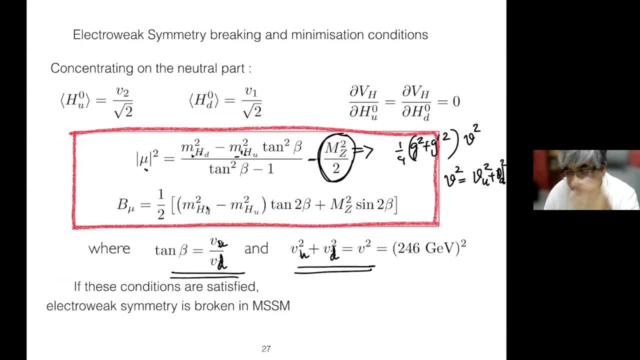 sign model satisfacely incorporates Higgs mechanism. So you get all the features of the Higgs mechanism, like Eukalka planes and the mass of the fermions and that's it, the masses of the gauge bosons and so on. so you can get it from here. 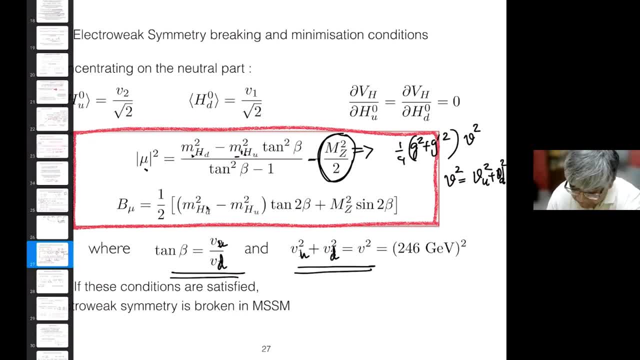 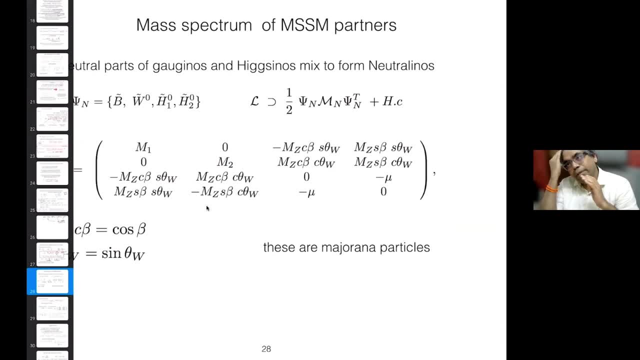 now, once the higgs is- uh, the higgs gets vacuum expectation value, um, the spectrum completely changes. okay, so once the spectrum first changes, uh, the mass pattern first changes when supersymmetry is broken, then after supersymmetry is broken because the mass spectrum earlier had equal, 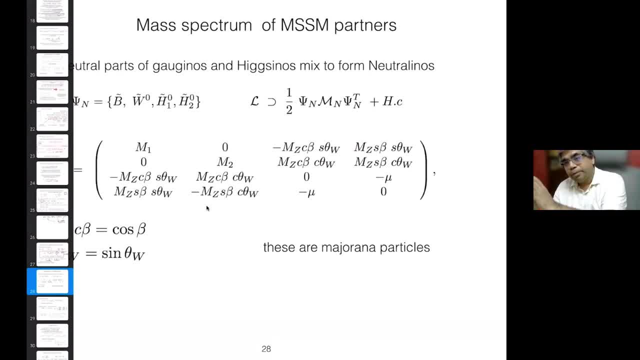 masses for all the particles. okay, once you break supersymmetry, the mass pattern changes because you have mass differences between particles and superpartners. and now after supersymmetry is after electroweak symmetry is also broken, meaning after supersymmetry. so there are three steps. 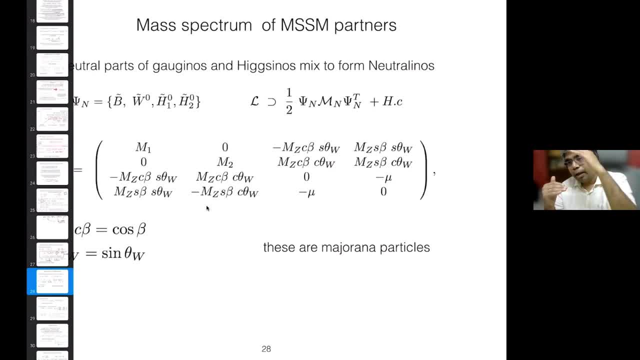 supersymmetry breaking, supersymmetry conserving, supersymmetry breaking and then electroweak symmetry breaking. after that, the mass pattern still further changes. for example, the. we know, we know these are your soft terms, these are your soft terms, but- and this is also- 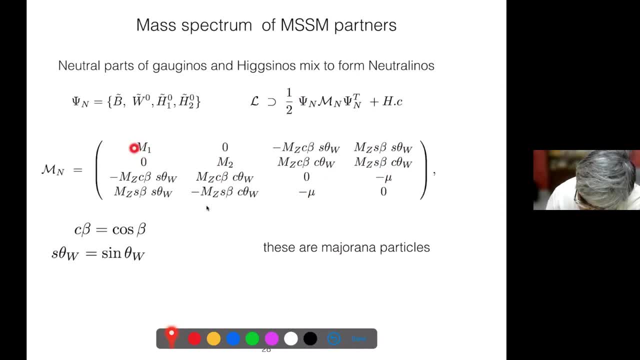 the supersymmetric conservative term. so these two are your supersymmetric breaking terms. this is your supersymmetric conservative term and these bunch are your electroweak symmetry breaking terms which are proportional to mz. so they start mixing. so we know, we know which are unmixed. earlier they start mixing with the higgs units. 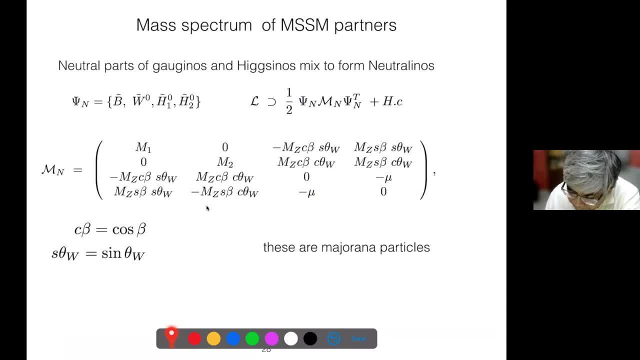 so these are higgs, you know, this is the down higgs, you know, and they start mixing with the up and down higgs units, and so, if you diagonalize this, these lead to some bunch of particles which are called neutrinos, which are called neutrinos, okay, and then similarly, uh, okay, okay, i am moving. 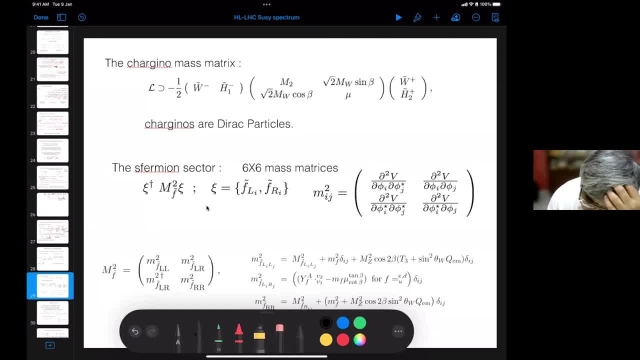 okay, then similarly, the charge partners of the we know, and we know this is again very similar. you have a supersymmetric conserving mass here, mu term, supersymmetric breaking term, m2, and these two are unrelated. earlier these two terms are decoupled earlier, but once electroweak symmetry. 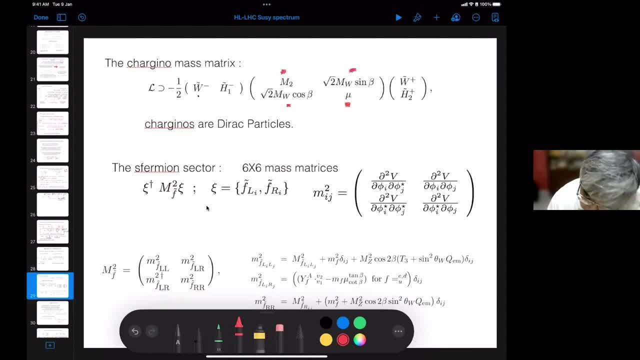 is broken, you end up having terms which break the electroweak, ending up in the lagrangian in their mass term, and they mix and they lead to something. on the charge units: these charge units are essentially derived particles, whereas the neutral units are neutral particles. 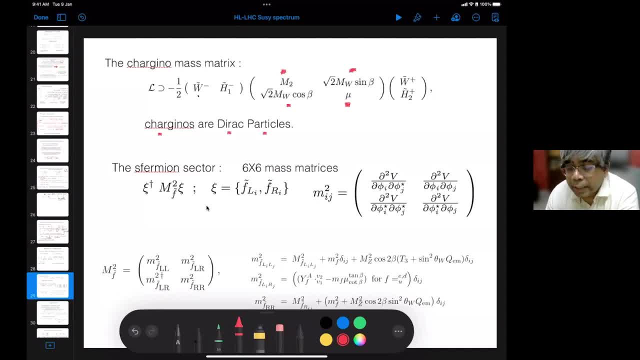 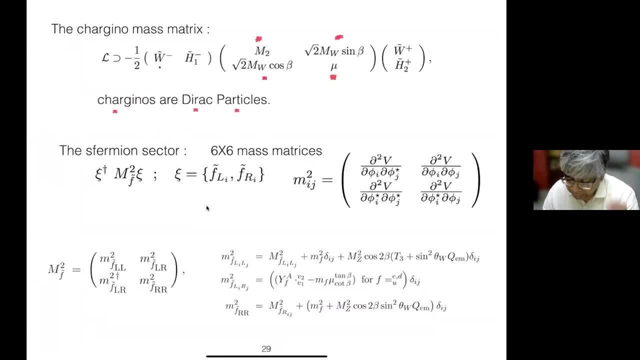 this happens to the full selectrons also. selectrons completely mix with each other. okay, if you write down the full terms because of the uca couplings or the selectrons, selectons, okay, selectons. and squawk mass matrices. they become six by six mass matrices with mll, which is given by, again, soft terms of this. 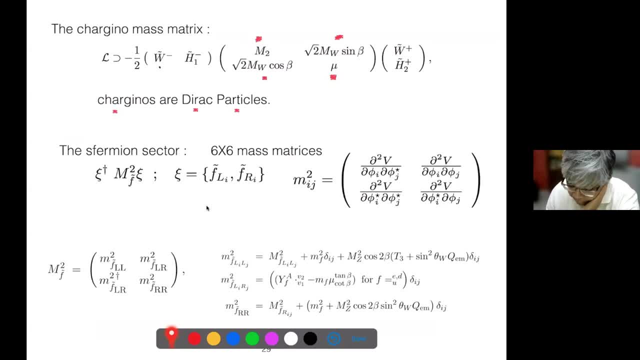 particular type. i am assuming no flavor violation. if there is flavor violation, this soft terms could also have some off diagonal entries. okay, if there is no flavor violation, the six by six matrices can be written in terms of three, two by two matrices. okay, three, two by two matrices, because 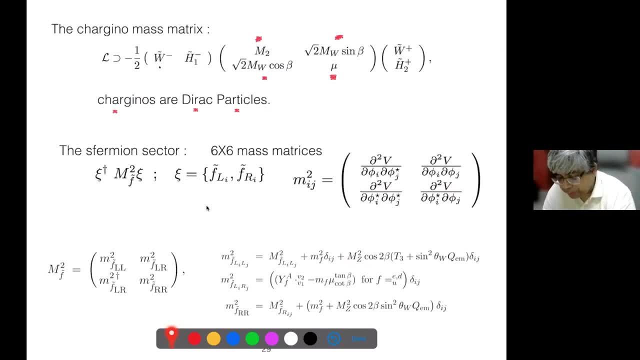 there is no flavor violation. this is six by six in full generations: first, second, third generation, left-handed and right-handed, and the left and right start mixing the moment you have electroweak symmetry breaking. given by this particular term, this is purely left-right mixing term purely generated after electroweak symmetry is broken. okay, after electroweak symmetry is broken. 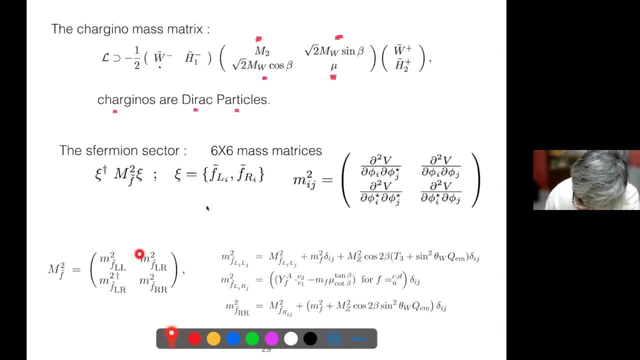 so these are your mll and mrr. this term is zero if electroweak symmetry is not broken. but the moment electroweak symmetry is broken, this term becomes non-zero. this is your left-handed soft term- right-handed soft terms- which contains supersymmetric breaking. 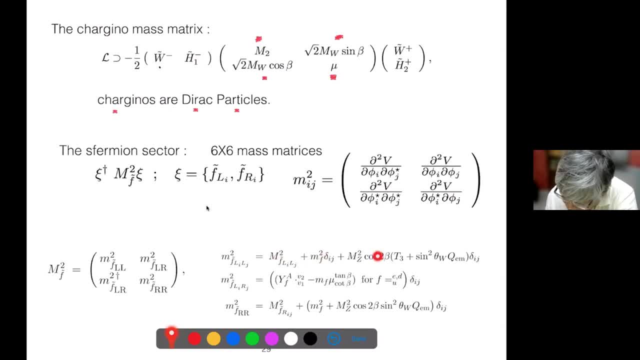 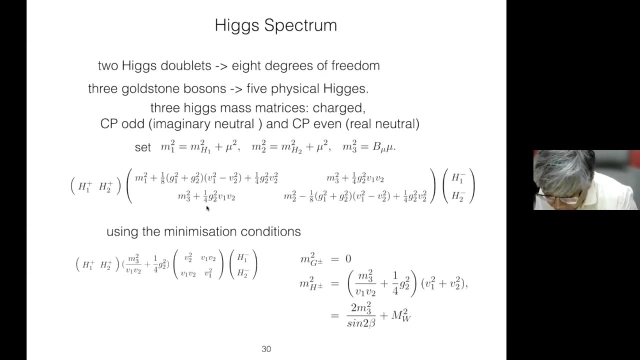 term, the supersymmetric conserving term and something called the d term. same thing for right-handed center, actually. okay, now let's look a little bit more into the heat spectrum. i think i have to run fast. so let's look a little bit more into the heat spectrum. i think i have to run fast. 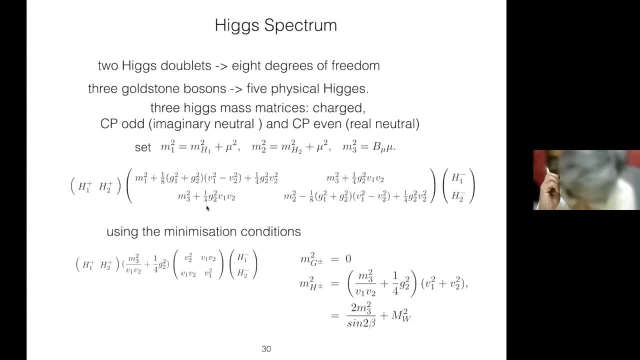 uh, so the two hexes will have eight degrees of freedom. so there are three goldstone bosons and five physical hexes. okay, so three goldstone bosons are essentially the charged part, two of them and one neutral. so there are three higgs matrices. one is a charged higgs. 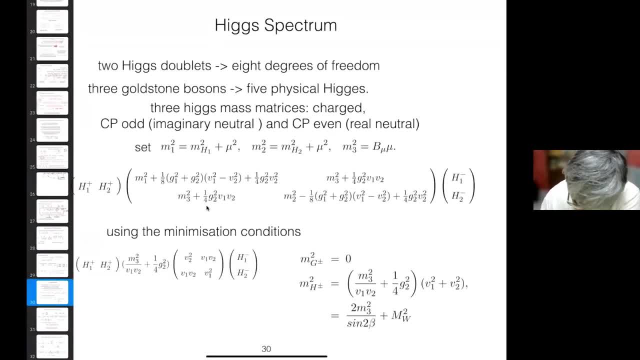 uh, one is the charged higgs, the neutral cp. odd higgs means the pseudo scalar higgs and cp even h, which is essentially um a real part of the, not the imaginary part. so this, let's start with the charge higgs part, the charge higgs part, if i set the subsymmetric. 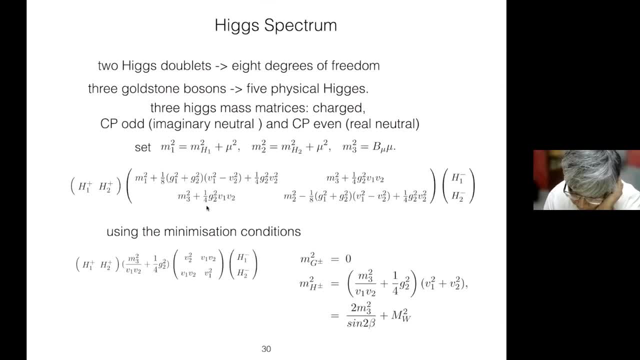 breaking plus, uh, supersymmetric conserving mass, to be mn square, supersymmetric breaking. okay, and this b mu, i call it as m3 square. i have this kind of a mass matrix and in this mass matrix, if i impose the two conditions which are the minimization conditions, okay, okay if i impose the minimization. 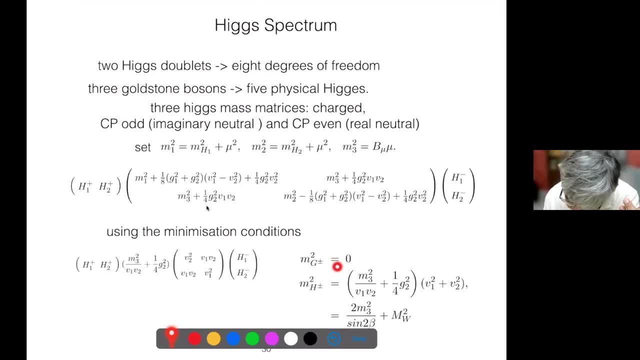 conditions. i end up with one of the term which is essentially called m square, g square, term which is essentially uh gold's. you know mass, uh goldstone goes on. this is one of the goldstone bosons are two charged goldstone boson and the charge higgs mass is given by this particular formula. 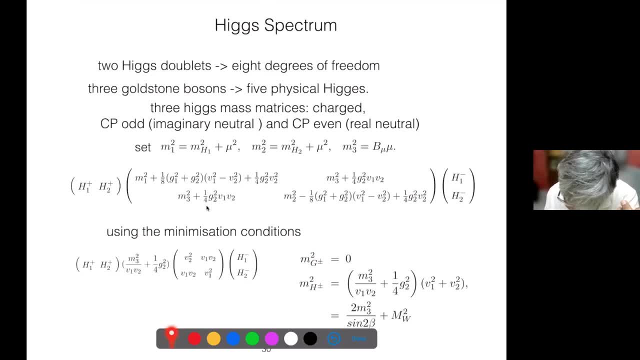 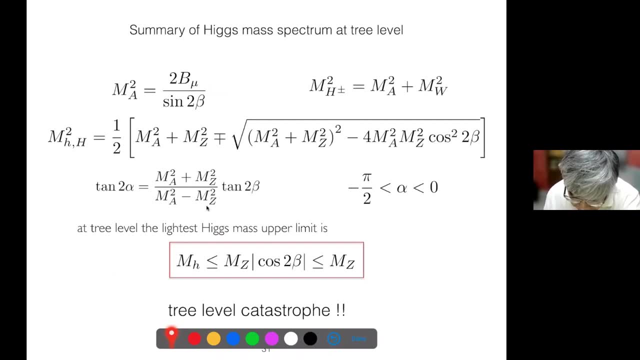 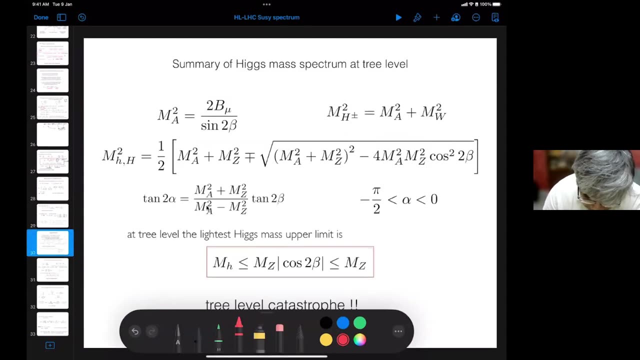 which is nothing but 2 b mu by sine, 2 beta plus mw square, the neutral hexes are given. the same thing will also happen, sorry, the pseudo scalar higgs has also very similar form, uh, very similar form, with one goldstone boson and one, uh, one, and pseudo scalar mass term, which is 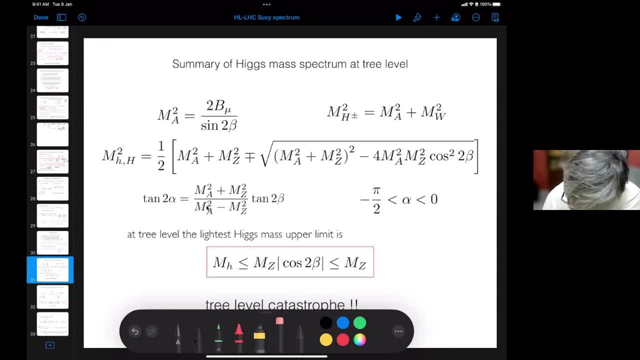 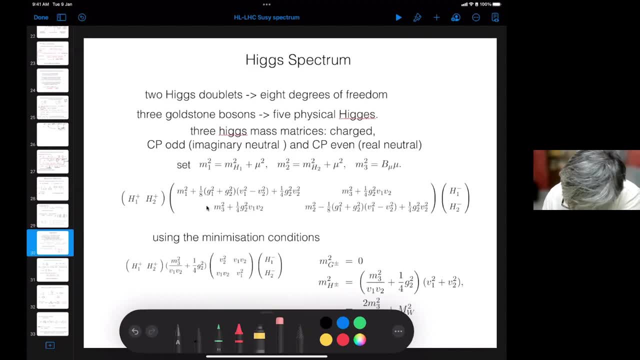 given by m a square, and this is given by m a square. okay, this m a square comes out to be to be mu by sine 2 beta. it has almost the same form. it has almost the same form, uh, the pseudo scalar master. except, instead of the it's not charged, it has the neutral part. so this is given by the sqaure term. 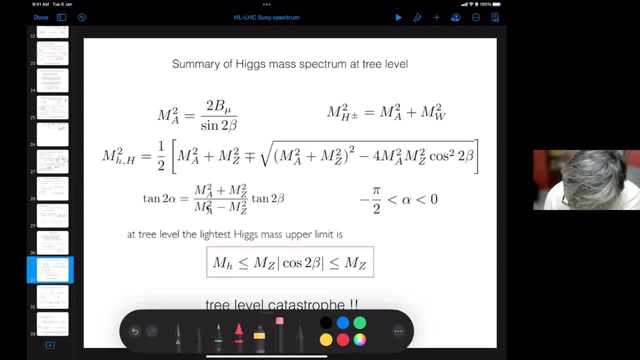 imaginary part of the Newton. Now, if you substitute, do the same thing for the real CP, even Higgs mass, you end up having this particular 2 by 2 matrix which has solutions with two eigenvalues of this type. Two eigenvalues of this type: one gives you the heavy Higgs mass and one 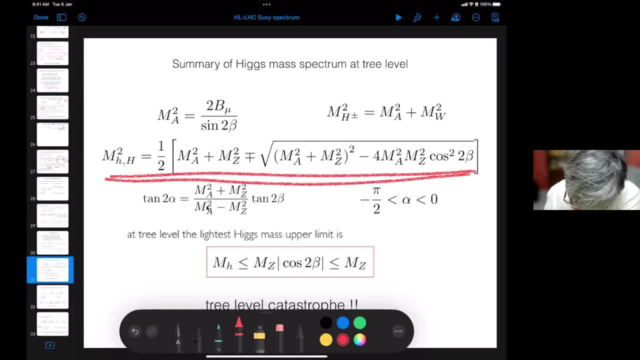 gives you the light, Higgs mass. And you see that the lightest of the two eigenvalues, the lightest of the two eigenvalues, has an upper limit of mz. There is an upper limit of. you can derive this upper limit. In the limit, ma tends to infinity. also you can derive. 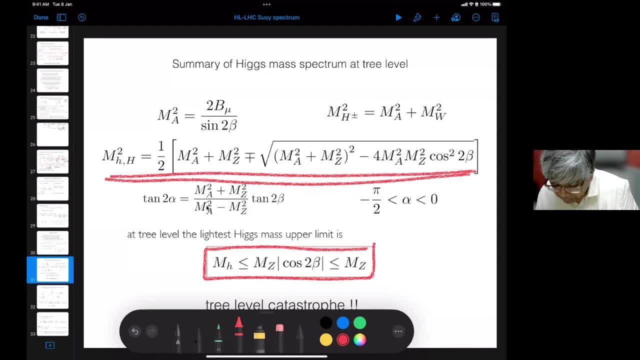 this upper limit And you see that at the tree level. at the tree level, the Higgs spectra predicts that the Higgs is as an upper limit. At the tree level, the supersymmetric theory predicts that the Higgs is mz. But then there. 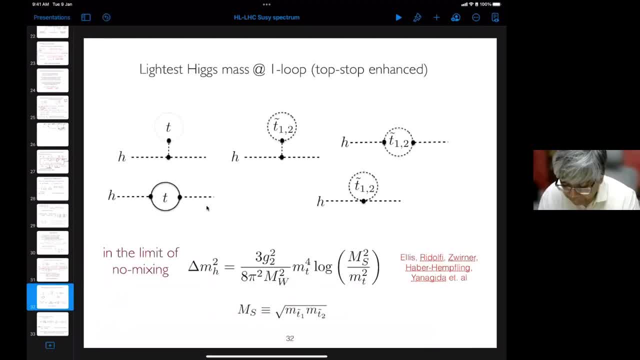 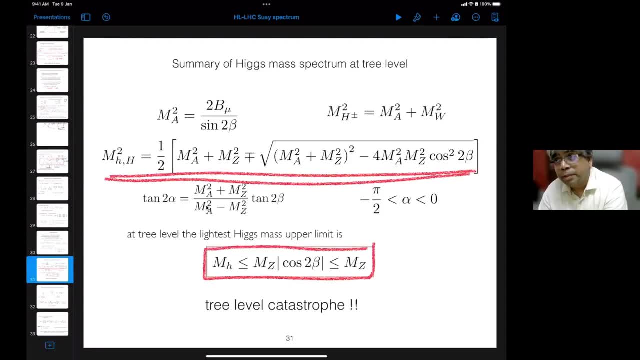 are calculations one has to do You have to do one loop, corrections and the one. so this is called the tree level catastrophe, and once this was discovered, people thought that supersymmetry is invalid. Like, like, like what they are thinking now They, they, started thinking. 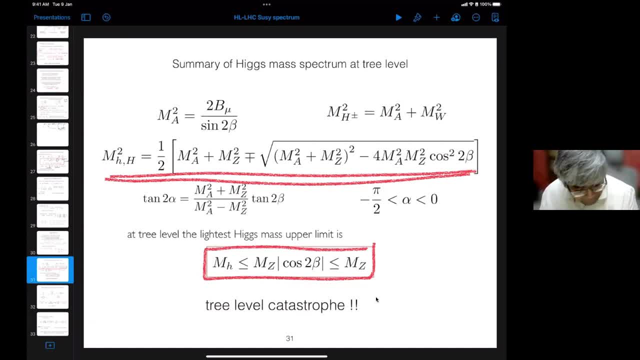 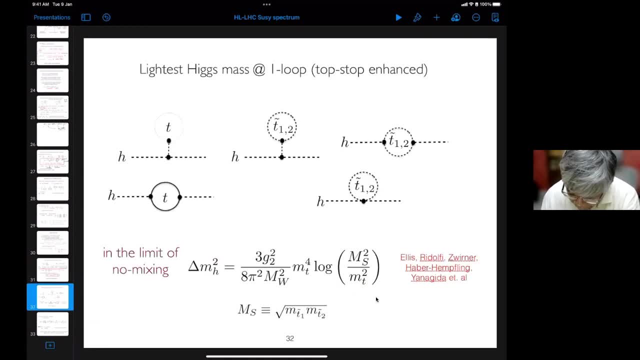 that supersymmetry is dead, it's not working, it's not possible, and so on. So but then it turned out that if you compute the one loop corrections in this case, the one loop corrections are extremely, extremely large. They are more than 100% actually. So 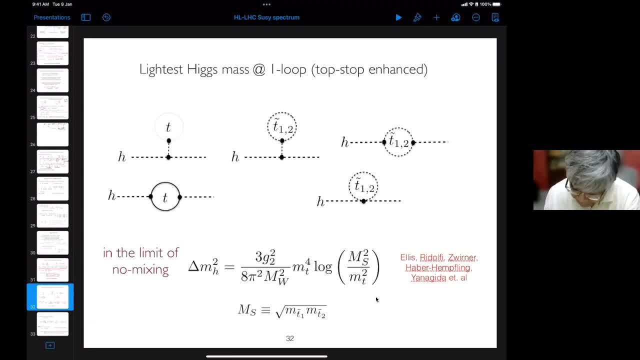 the correction goes as the fourth power of the Higgs mass. The one loop correction goes as the fourth power of the top mass. sorry, not the Higgs mass. Remember the example I gave you in Yukawa theory? In the Yukawa theory the corrections to the Higgs are not proportional. 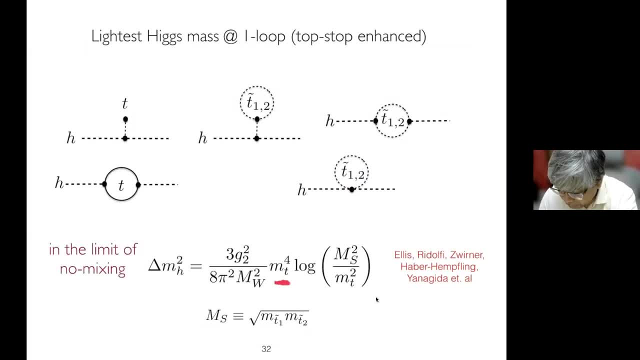 to themselves, but they are proportional to the Higgs mass. So the Higgs mass is the same as the Higgs mass, but they are proportional to the fermion mass. So exactly the same thing is happening. This is the Yukawa theory. The corrections are proportional to the fermion. 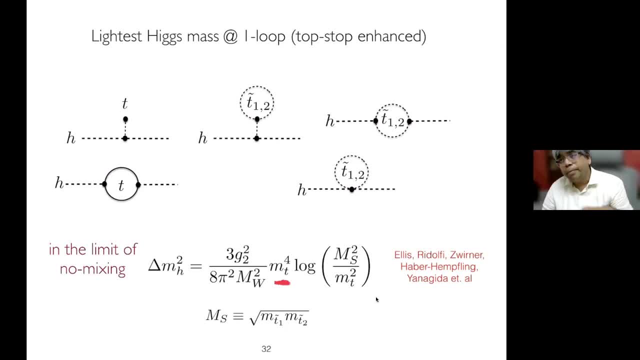 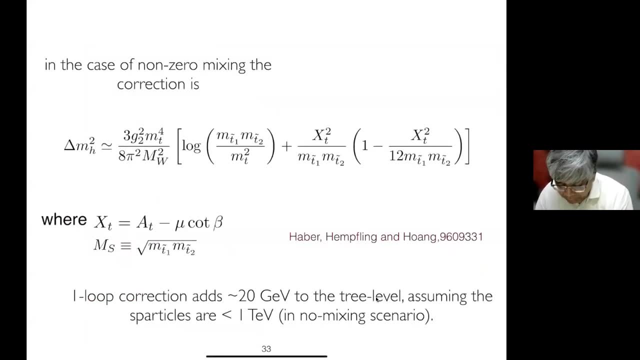 mass and because the fermion mass is very, very large, which is the top mass, so the corrections are also extremely large. Okay, they're extremely large, and these corrections keep adding very, very large numbers, all the way up to. so, from 90 GeV they can push the. 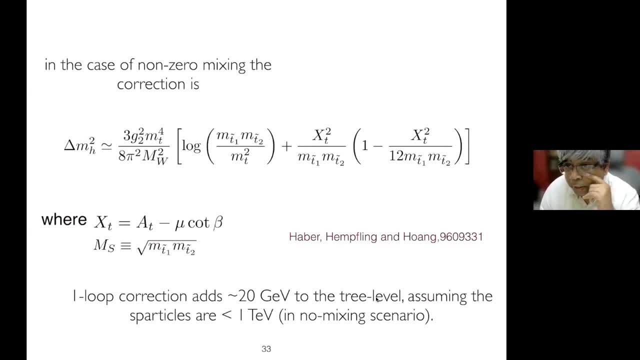 fermion mass to be around 115 GeV, 120 GeV depending upon Xt. Xt is the left-right mixing in the top-stop plane. Okay, So this is an effective theory calculation. This is an effective calculation for this term. So here I wrote 20 GeV, but it can add all the way up to 30. 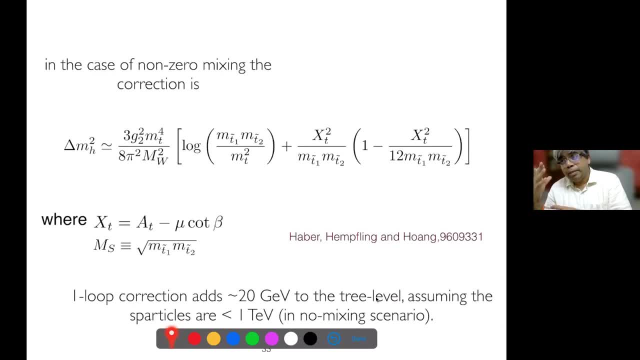 to 40 GeV. correction to the 3-level mass. So you remember, this is added in square because this is scalar mass, So this is added in square, So you can take the left-right mixture. and this is added in square because this is scalar mass, So you can take the. 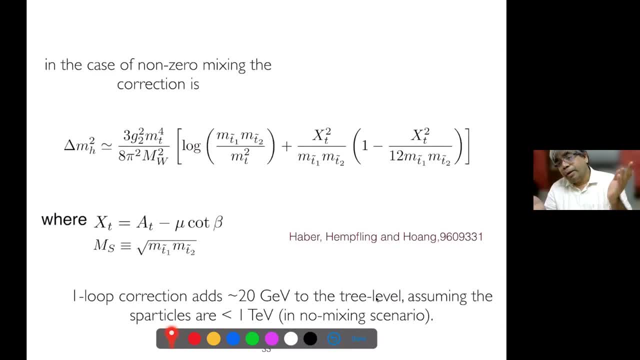 scalar mass. So if you don't take the square, it can now add almost 130.. So it can push the mass from 90 GeV to almost 130.. So if you want to get a square root 2 factor or 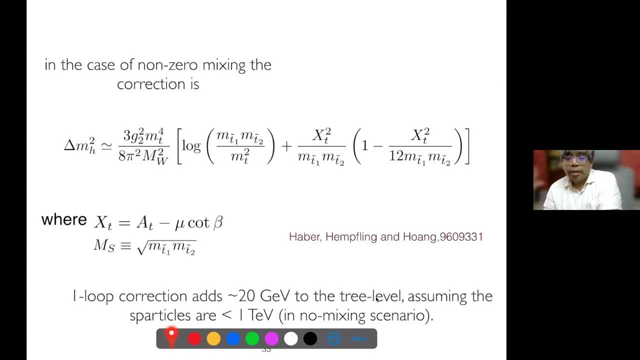 effect onto the H mass. so you really get that kind of an effect with a very, very large mixing. If you maximize this Xt, if you can maximize this Xt and take stop masses to the order of 1 TeV or 2 TeV, they can give you the correct Higgs mass. They can give you. 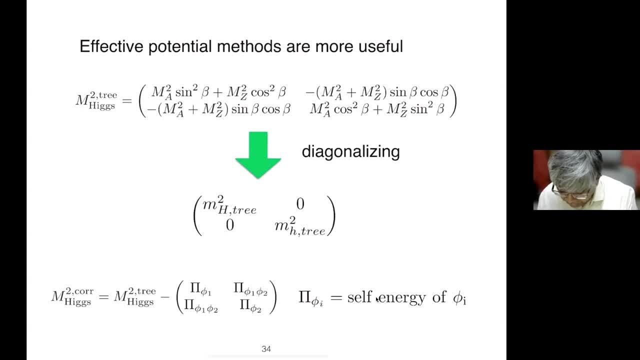 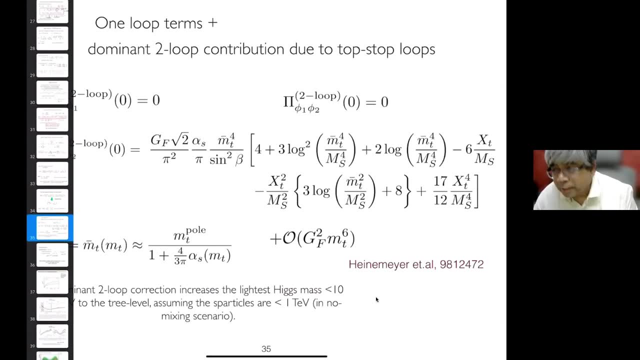 the Higgs mass. Then there are two-loop corrections. I think Petro Slavich will talk more. I think These two-loop corrections are also very, very important. Here I am talking about the dominant two-loop correction. Here I am talking about the dominant. 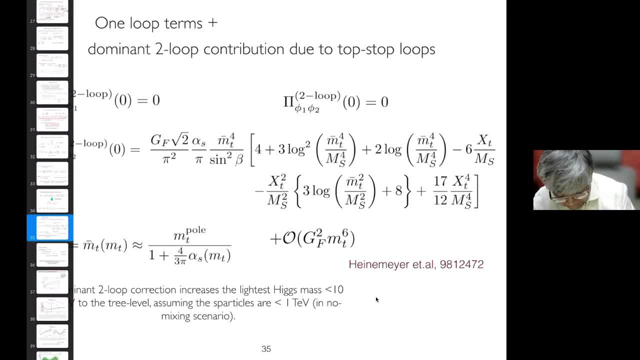 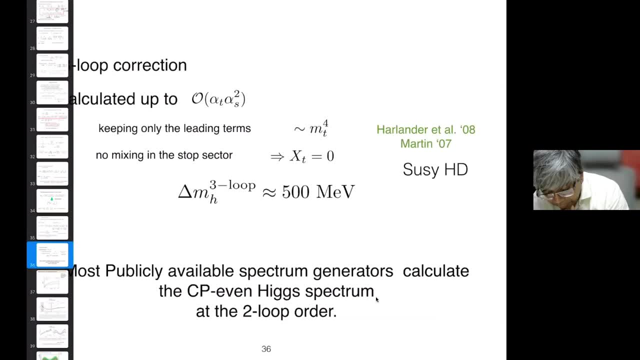 two-loop corrections, But I think he'll talk about various other effects. essentially, And in the last four, few years ago, five, six years ago- work has started on working on three-loop corrections. Purely using one method is actually using effort to feel 3D. 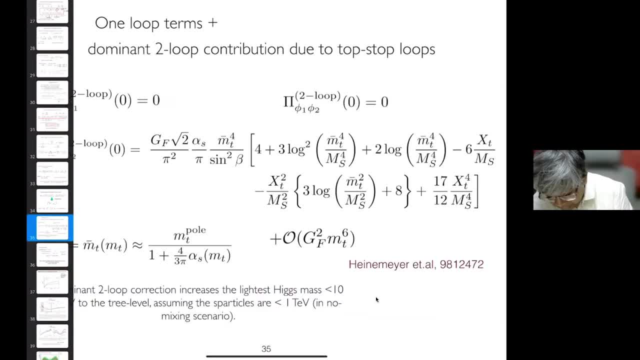 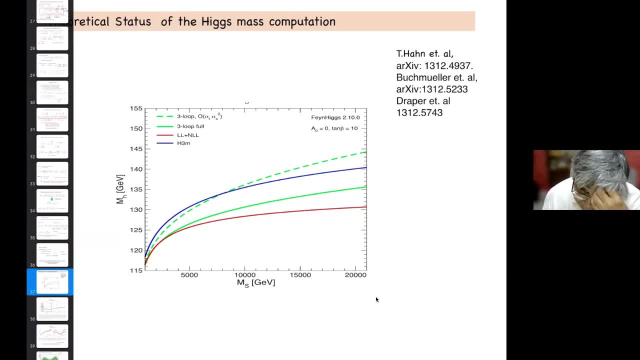 Now, to put it more clearly, we take sequences by Poisson over the Yorkyan sliding to a certain amplitude, and that indicated what our P sort 같습니다 convention was actually being. shouldn't be the same difference? okay, you see it makes it, because the higgs mass is now being pretty accurate. 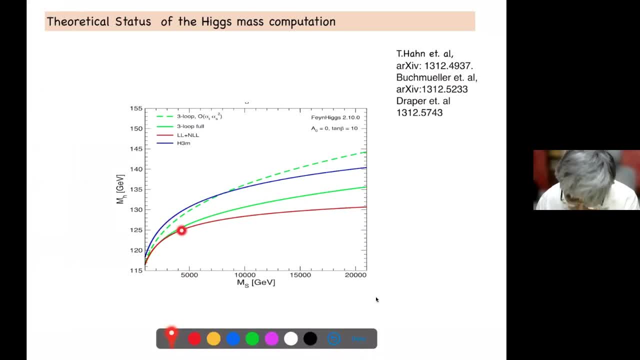 it is around 125 gev now at this region. you see, it makes a huge difference whether you are using a full three loop or whether you're using h3, meaning leading log effects, or whether you're using any of this thing. so the higgs mass computation is one of the most important. 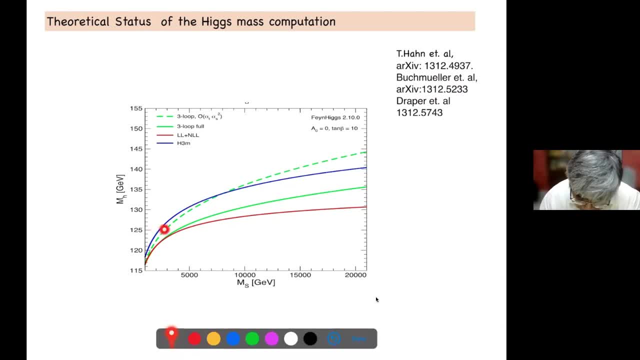 computation right now, because from the higgs mass you can relatively easily estimate very well what should be your uh stock mass, uh required to satisfy the data. okay, just from the higgs mass itself. so the higgs mass put a very, very, very strong constraint on supersymmetry data, of course. 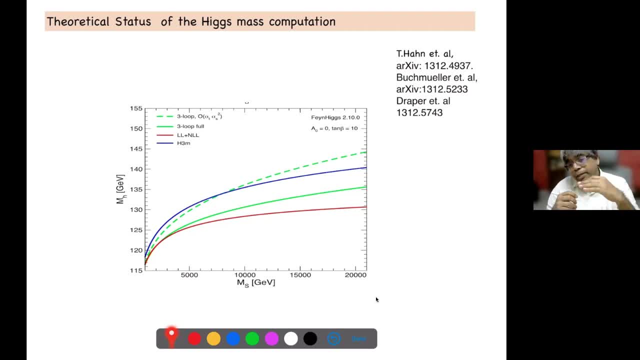 it puts not just on stock masses but also on the gluino masses, because the two loop corrections contain gluilo masses and so on. so so it's a combination of various things, okay. so if one plots in the stock gluino plane, i think that would be a good thing. 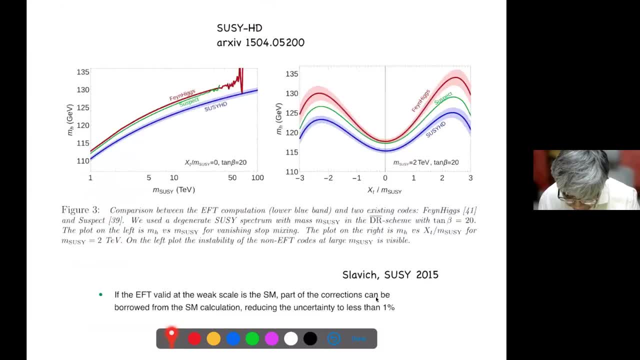 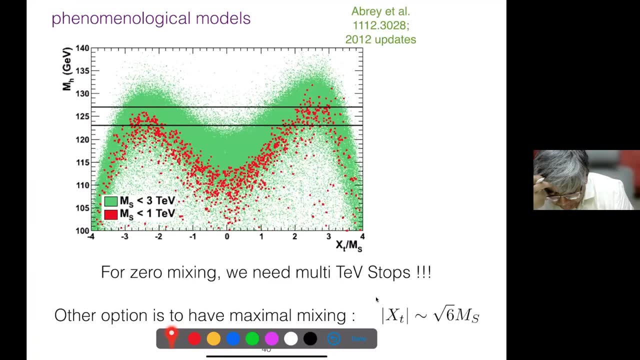 here. this is just the stock. masses and people have been looking at various difficulties in this particular case. i think this part i leave it because i think what i try to tell you, i'll just tell the result actually. so this result tells you that yeah, so how much more time do you need? i think another 10-15 minutes. is that okay, because we will go for. 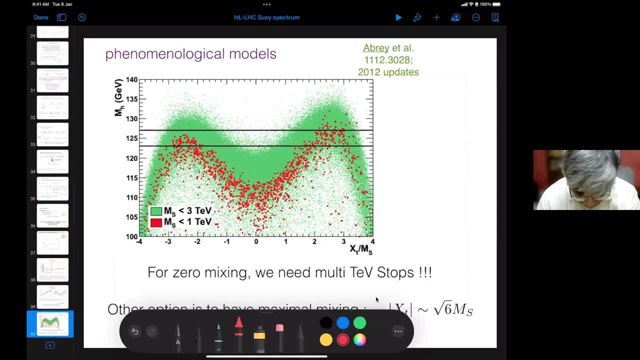 the coffee after that. in that case, okay, uh, maybe i'll stop uh soon enough. yeah, so, maybe five, ten minutes. yeah, ten minutes is okay, please go ahead. yeah, ten minutes, okay, thank you. yeah, so, uh, i'll just tell the results because i think there will be a lot. 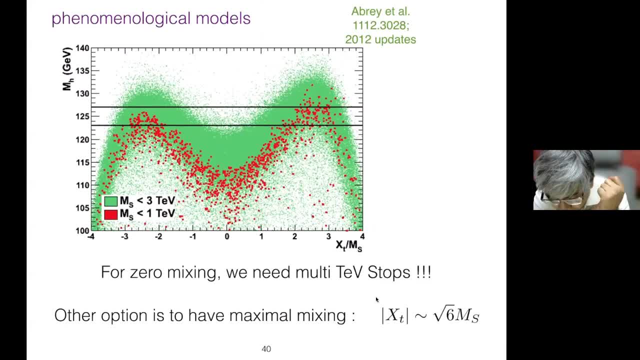 there are going to be another talk on this by slavich and company. so the main result of the higgs is that if you have one tv stops, you cannot explain the higgs mass. if the stops are one tv, you cannot explain the higgs mass with zero mixing. so we are already reaching that limit in lhc. 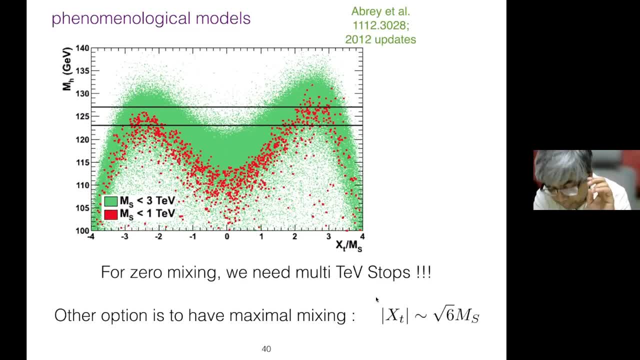 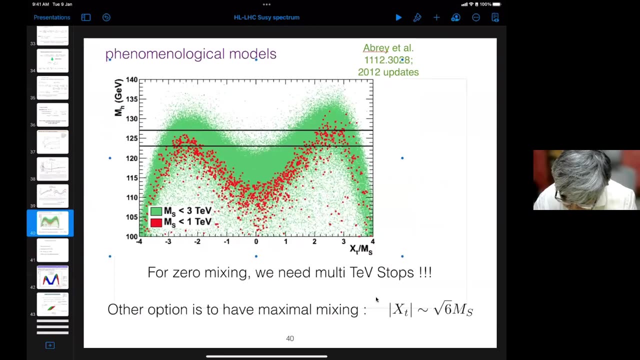 so one tv stops. if you want to have one step, one tv stops, you need to have extremely large mixing. uh, and this is a very good, good, good prediction. so one tv stops will require very, very, very, very large mixing. okay, as you can see from the uh red points here. so, on this plot, what is the higgs mass on the y? 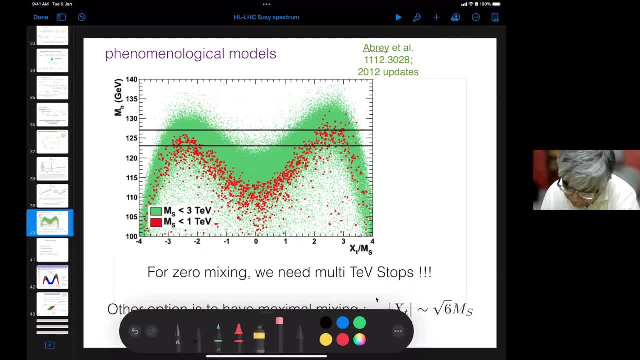 axis and the mixing on the x-axis. okay, if the mixing is very large between within the stop left and stop right, which is because of the coupling and the a term, and the a term is very, very large, this means a prediction that the a term is very, very large. so you already have. 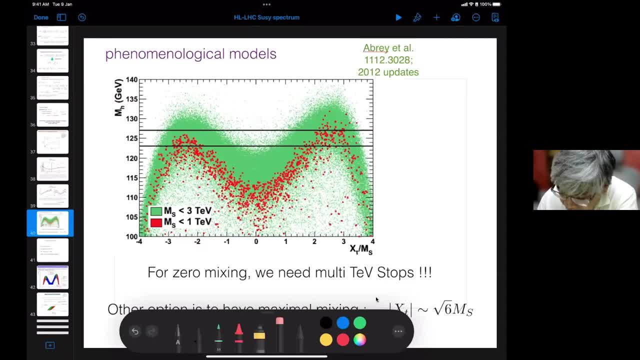 a prediction for the higgs mass, saying that if the stock mass is around 1 pv, so maybe hlhc will see it. okay, if hlhc will see it. so it gives you a prediction for the stop mixing to be extremely large. on the other hand, if the higgs, the mixing is very, very small. 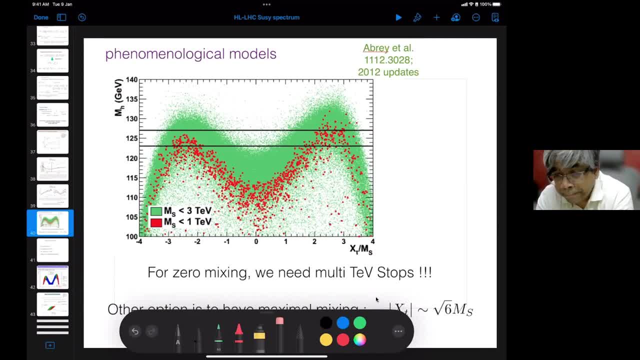 the stops could be very heavy- 3 tv or 4 tv, okay. so for a mix with zero mixing you need, if you want to sit in this region, you want to sit in this region of 125 gb, you need only the green points. okay, only little bit of green points exist in this particular case. 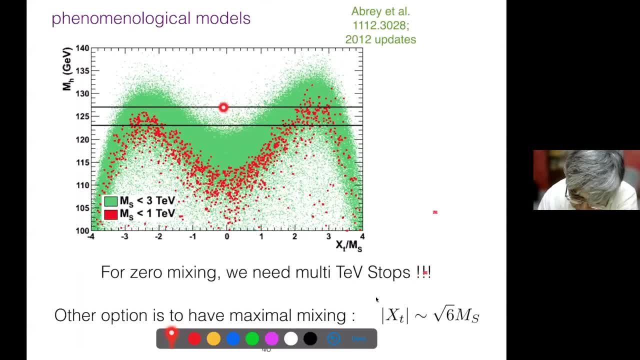 okay, only only the green points exist within this region, small, small green points actually. so multi-tv stops with zero mixing are possible, or so there is some sort of a no, no go theorem here, which is an important theory. uh uh, important thing that there is either multi-tv stops. 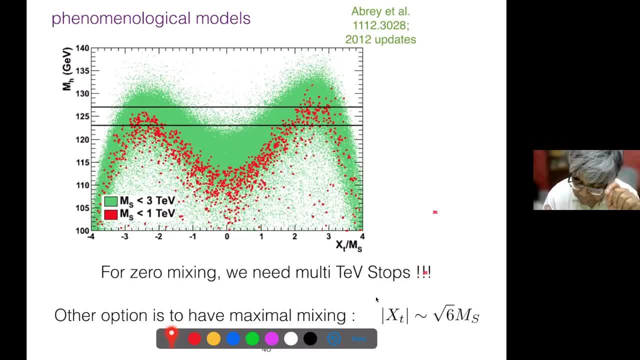 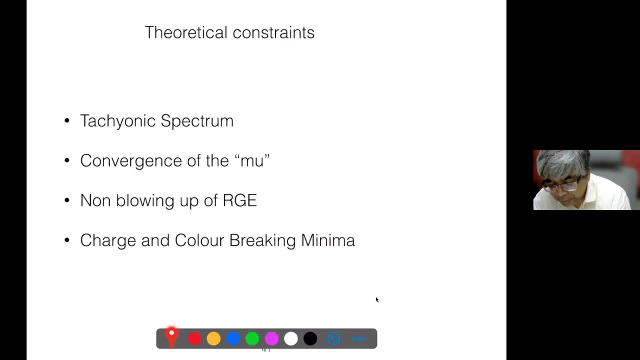 with zero mixing or, uh, large mixing with tv scale stops is something. so the stops will be found, hopefully at hlhc. they are, they are within the region. hopefully a betterment on the stock mass will be there at hl. let's see, but not so significantly. but let's hope that the hlhc will be helpful in the future. 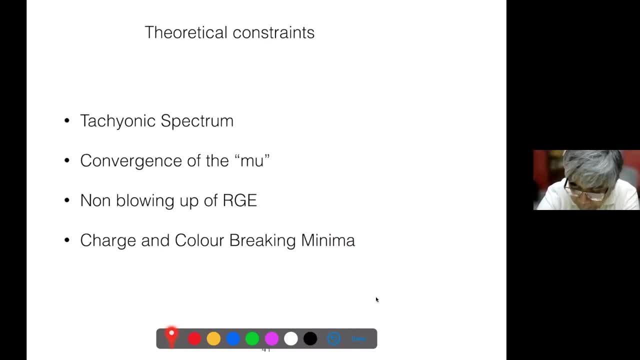 that there will be something in the telekinesis. So now, so far I have derived you all the spectra, meaning all the parts of the Lagrangian. I told you how now we had to compute the spectra. You have to come to compute the spectra. let's just say that I don't know where the 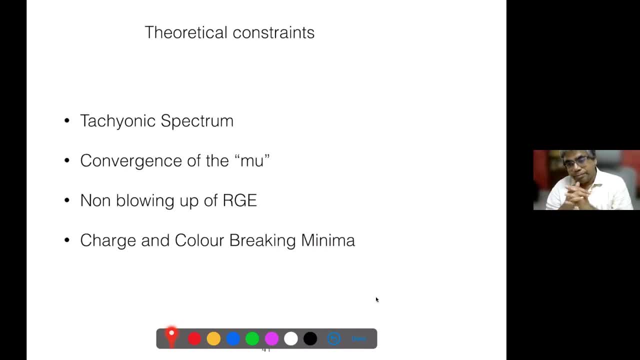 supersymmetric taking is now that is a completely so. the way one does is computing. the spectra is a part of the parameters are well known in standard models. so you take those parts in the standard model then convert it into supersymmetric partners, meaning in supersymmetric theory, and then run something called the renormalization group equations of these. 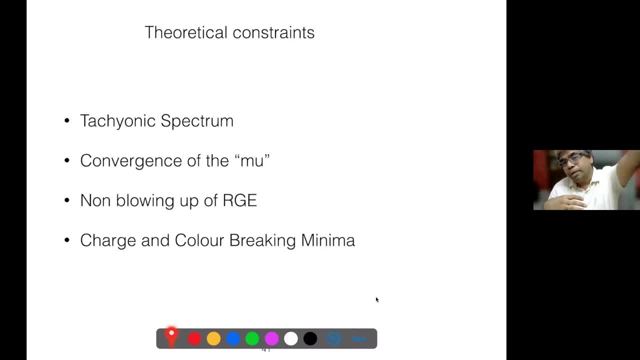 parameters, from the scale of supersymmetric breaking to all the way to the gut scale or Planck scale, and then bring them back, compute the corrections. So this computation of this supersymmetric spectrum is a complicated numerical program. one has to come to compute, actually one has to write down this complicated numerical program. 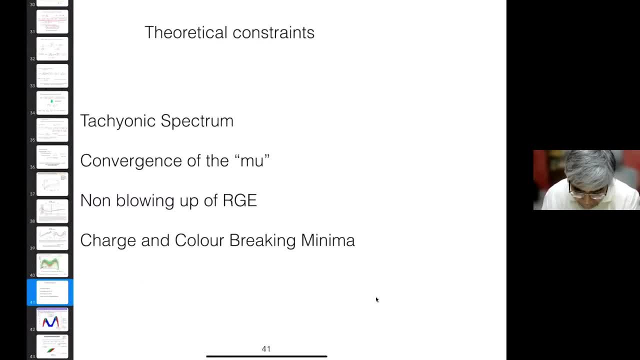 it meant. for us. it took some couple of years to write it down, okay, and then compute, compare, okay, and then something like that. and then going back and doing these operations, you can see that actually we can also compare it with exponential results, like, for example, you check what happens at the spectrum or give a result in spectrum, we compute and compare it with. 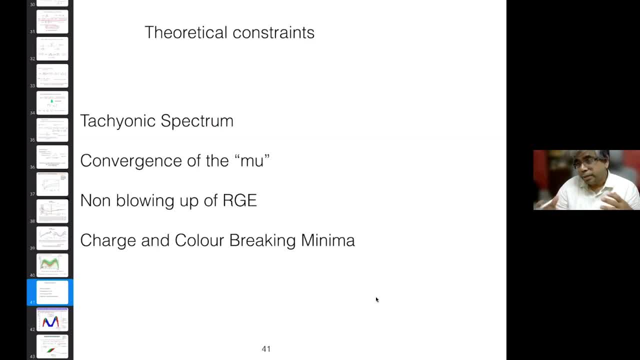 the LHC spectrum. like you check for a given supersymmetric model whether it satisfies the minimal models or results, or something. you had to do this, something called nowadays it's called recasting of results for every model, let's say, for example. but just to say one thing: 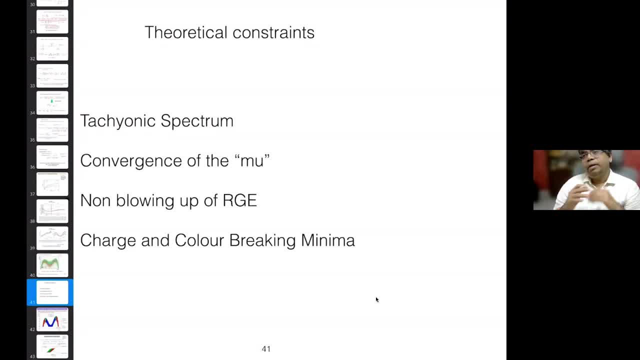 so there are a lot of difficult technical aspects, uh, when you are computing spectrum actually. so first of all you have to worry about, uh, the regularization scheme, because all the standard model parameters are given in ms bar, then you have to compute into dr bar and then you have. 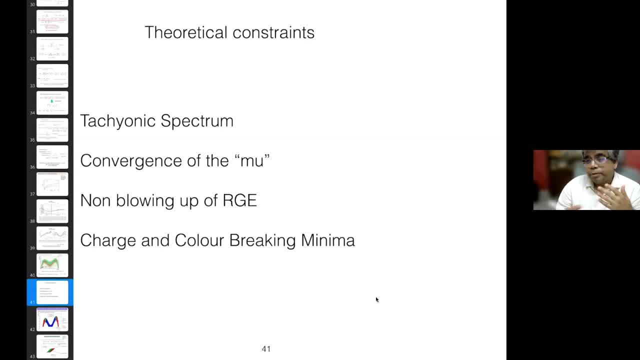 to run the rg equations inputs. okay, because if you change the regularization scheme, it changes. it gives you something called the threshold corrections to your parameters, the parameters, running parameters. so these have to be done. after doing all that stuff, before matching the spectra with the theory, with the experiment, you still have to satisfy, uh, some theoretical constraints. 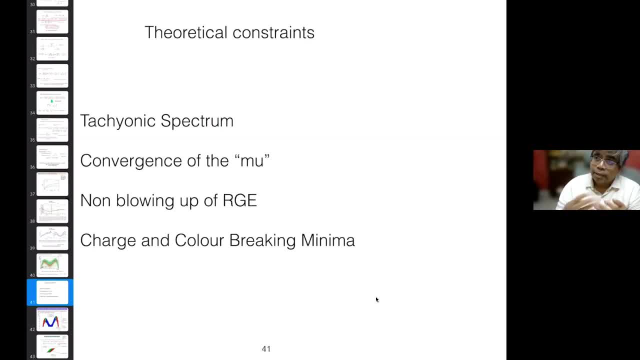 like. for example, you should not have any accounts in your theory because accounts are unphysical. you should have the convergence of the new correct. electronic symmetry breaking is correct. the convergence of new essentially means that electronic symmetry is broken correctly and you are not blowing off your rg. that means if you choose. 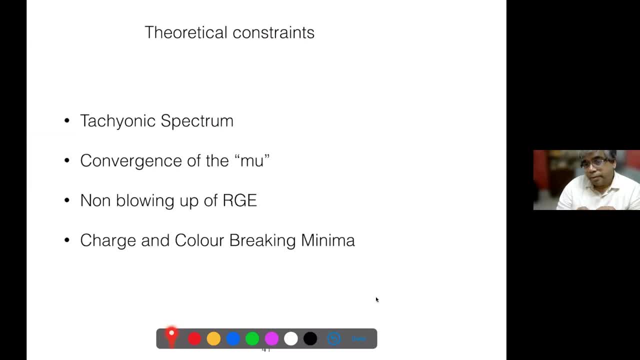 some tan beta or something which is very, very unphysical. okay, uh, you can blow up the top mass in your running of the parameters, you can block, and the final thing is charge and color breaking minima, like, for example. this is relevant nowadays because, um, like i said, if the mixing is very, very 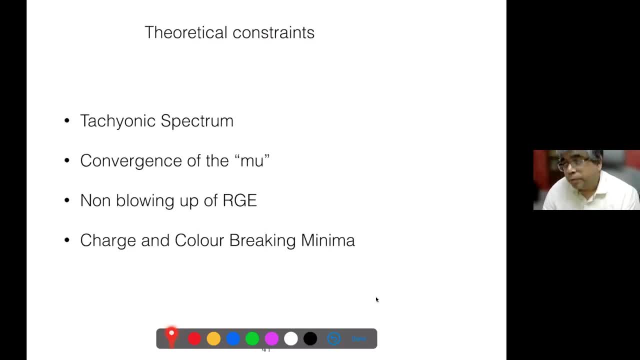 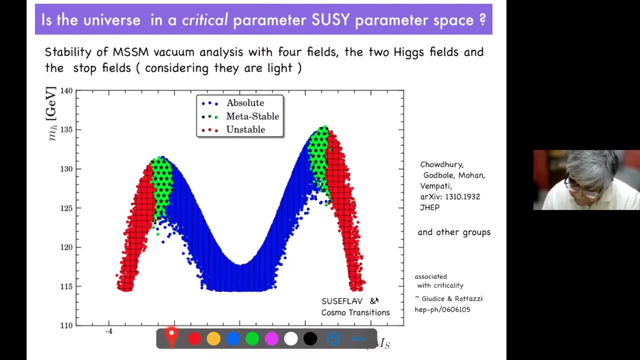 large in the stops, then the stops could get a vacuum expectation value. if the stops gets a vacuum expectation value, they break color and charge: color charge and electric charge. both these charges are breaking so you have to worry where the higgs mass it sits okay, and whether in the region where they sit. 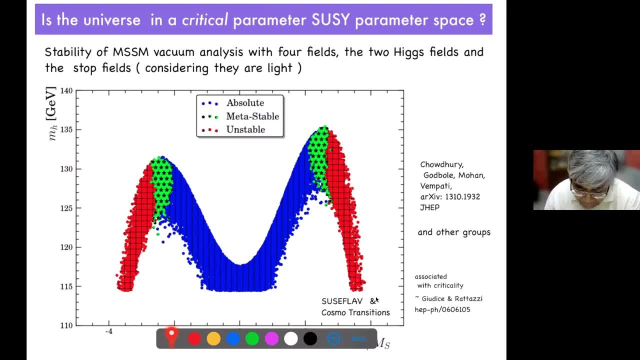 whether you're breaking uh, the color charge or so on, or electric color charge. if you break color or electric charge, it becomes the universe's is unstable or metastable. say, for example, in this region we have plotted those regions which are unphysical. now you see this peak, this in m peak, exactly the peak in. 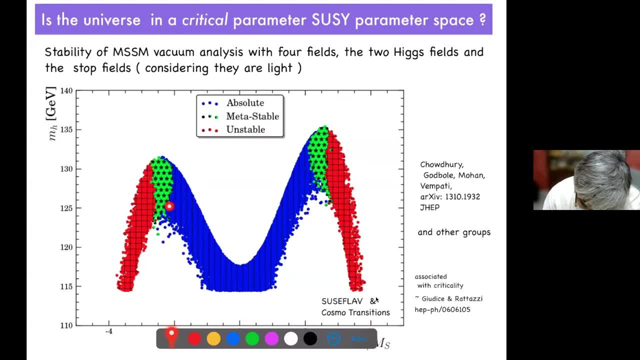 which the higgs mass is valid. so this is around 125. you see, there are large regions which are unstable, large regions with large mixing which are unstable, and regions which are absolutely stable, which are a little bit inside, a little bit inside. this is the same plane as before. so this dotted. 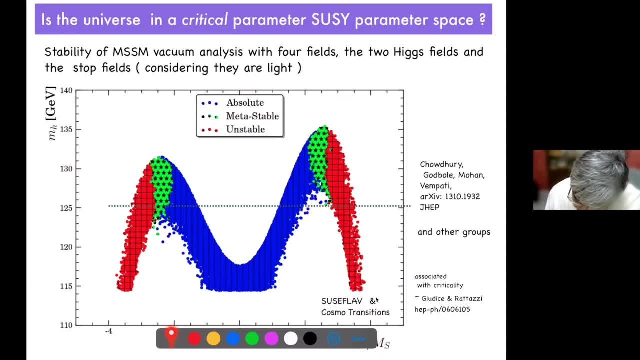 is the line in which the higgs mass is satisfied. so you can also know which region of the parameter space you are lying. so the stock mass cannot lie. uh, the stock mixing cannot lie in the red region because that would mean the universe is unstable. it cannot lie in the green region because it 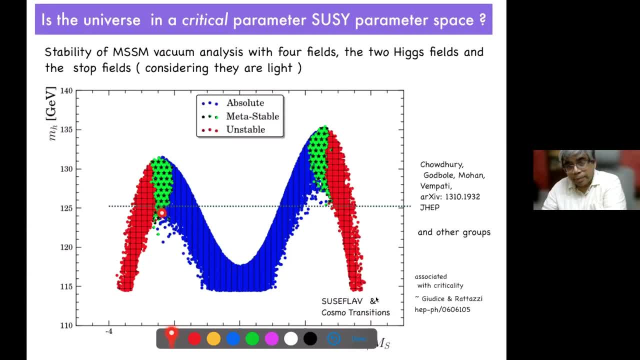 only can rely in the left hand side of the green region, because it means that the universe is metastable, but the stop parameter is negative, okay, and if it lies in the blue region it will not like it's fine and good, because that's. it can lie only between the green region or the blue region. 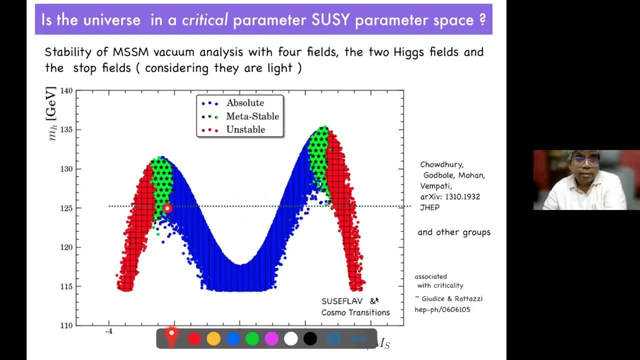 so you see that the regions, the theoretical constraints and the higgs mass constraints already tell you if the stops are around one tv or so, as they can be discovered at actual lse or something, or if they're heavy, it's fine. okay, this is up to two tv or three tv. 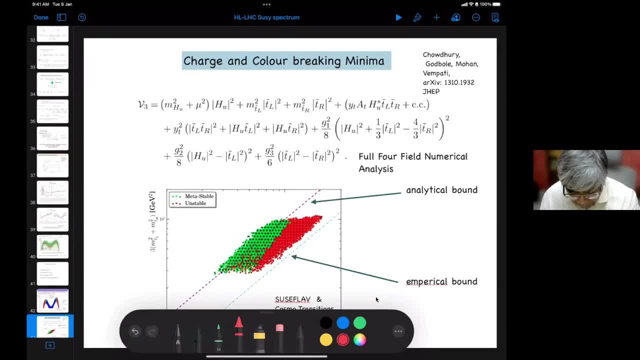 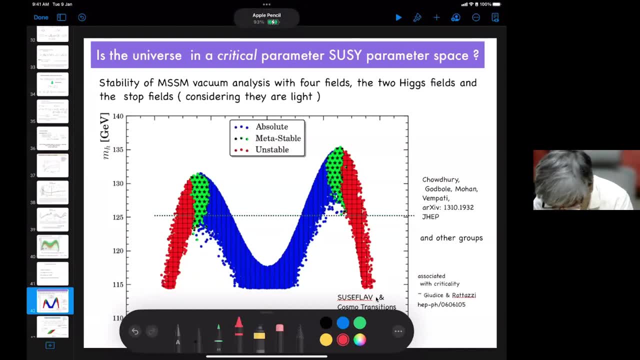 uh, it shows that, uh, uh, you already know what is, uh, uh, the reason of the parameter space where the higgs is valid. okay, now, okay, let me stop here, i think, and then before. okay, if there are any questions, i'll take it that much, yeah, all right. thank you so much again, professor, for this. 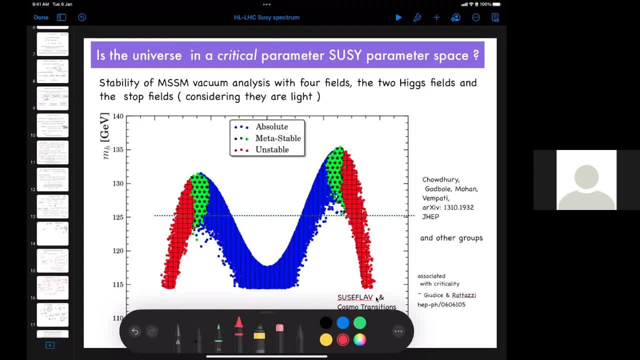 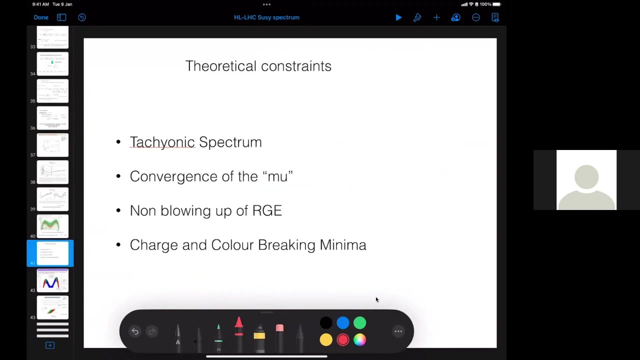 marvelous um talk on covering the particles generation and also the higgs sector in the sushi. so time for questions, especially the students, please. one wants to ask the question. he has patiently derived everything okay, anybody else from, from the audience the other people like, apart from the students. 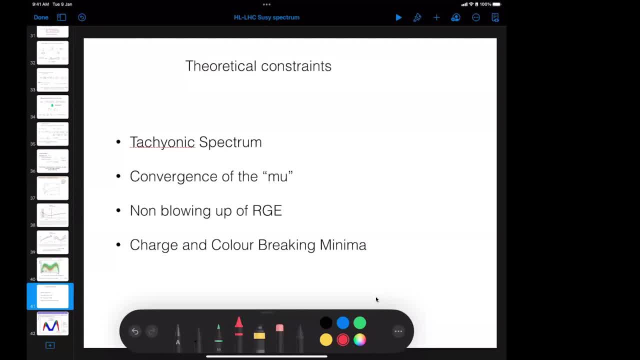 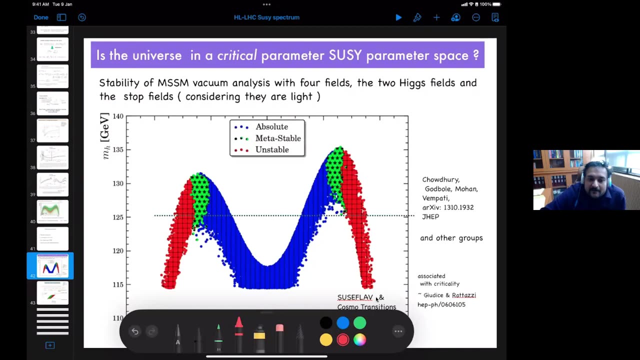 hello. so just one question. so could you please comment a little bit more on the last plot. so it's about the stability and the higgs mass and the allowed range of the stock mass, especially when it is on the left side. so in in the interface of this metastable minima and the absolute minima. 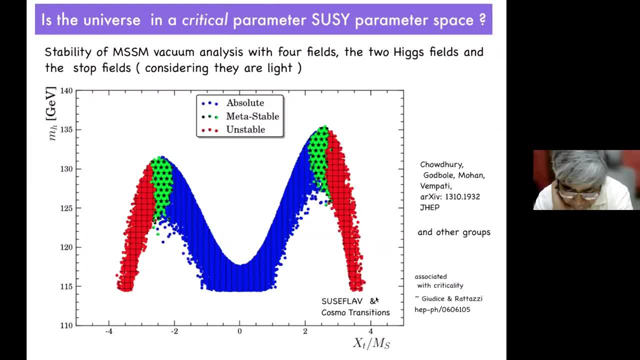 right. so the point is that this analysis, we have done it with the numerical. it's extremely challenging, okay. so the point is that what we are looking at is we, are we computed, uh, the lifetime of the vacuum? okay, lifetime of the vacuum. if it so, there are two things. one is: 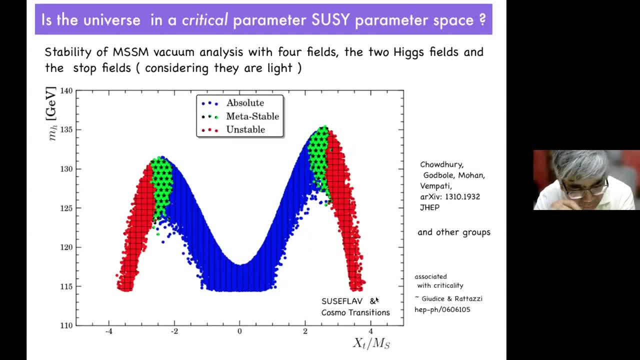 you're looking for a deeper vacuum and if there is a, uh, there is a global vacuum, and if there is a local vacuum, okay. so the question is, if you, if you have a local vacuum and a global vacuum which is deeper, if the global vacuum is deeper, deeper inside, which is which is color and charge breaking? 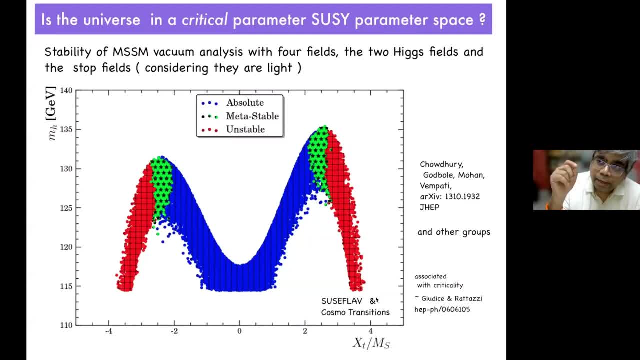 then there could be uh transitions between the deeper back to the color breaking uh normal vacuum, which is not color, and uh charge breaking through the deeper vacuum. there could be transitions between these two. okay, so the red region is those reasons in which the deeper vacuum lies, which is color and charge. 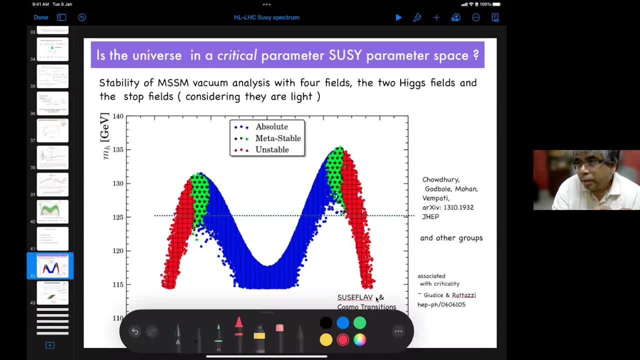 breaking, okay, okay, and the green metastatic. uh, the green regions are the one where the global vacuum is just about such that the lifetime of this vacuum is metastatic. The red regions are completely invalid. Now, the reason why there is a small misstep between the left. 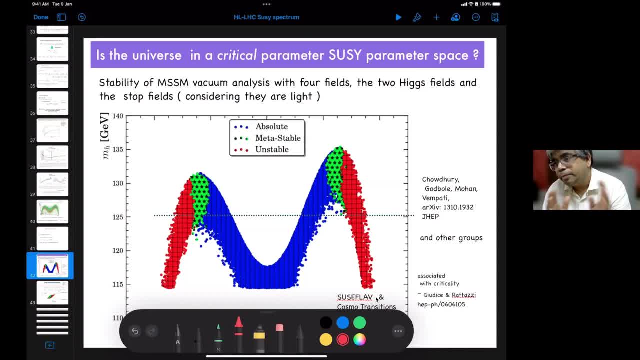 and right is essentially because of the cancellation of the mu term. in the Higgs potential. There is a small effect, essentially, which is coming up. So the left wing, the left M and the right M are not exactly symmetric in the computation of the Higgs mass itself. 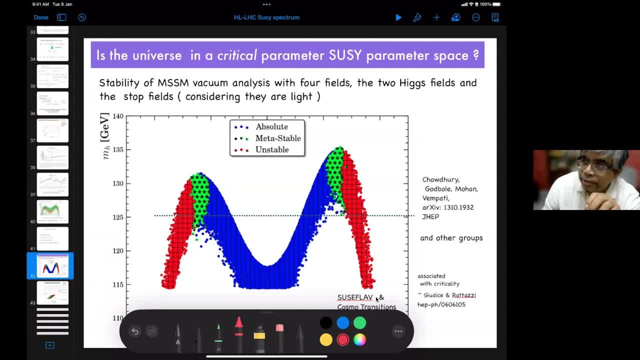 This is not a bigger effect of the vacuum transitions, This is an effect of the Higgs mass itself. So because all these points are set by the Higgs mass, So within the Higgs mass itself, you can see the previous plots also. There is some asymmetry in the M's. They are not exactly 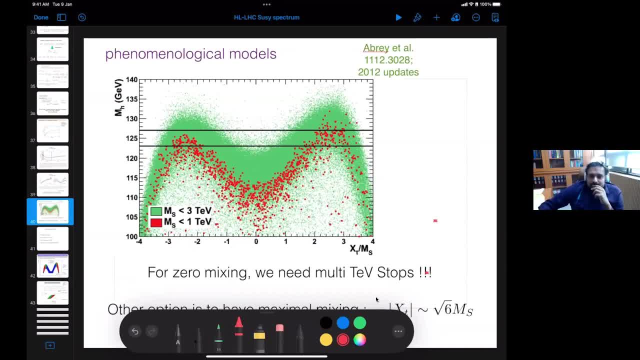 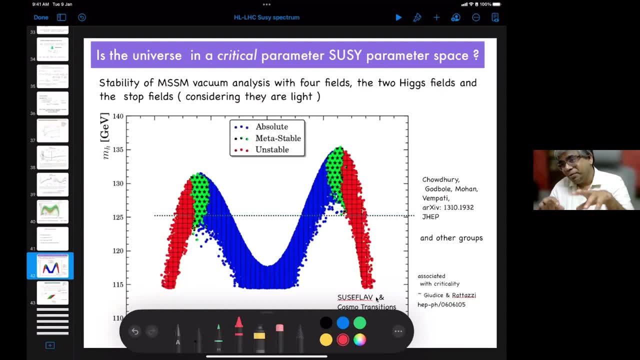 symmetrical. As the A term changes sign, so this also changes sign. But remember that this is a four field analysis, 4 scalar fields. But if you do more scalar fields, this has a will. In principle you can do it for. 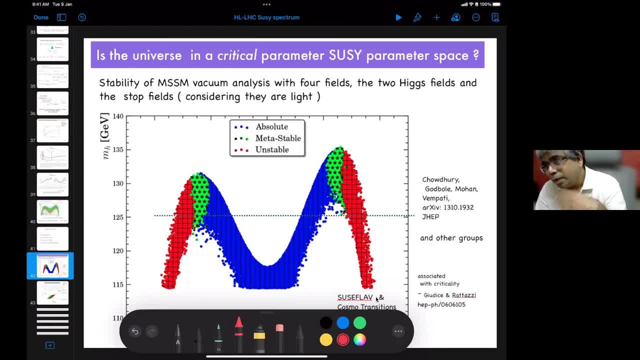 the bottom also, because in 2 loop corrections you also have the bottom And for the 3 loop you also have the bottom and the top. So if you do this analysis for 6 field or 8 field, you had to do it fully for the 6 field and 8.. 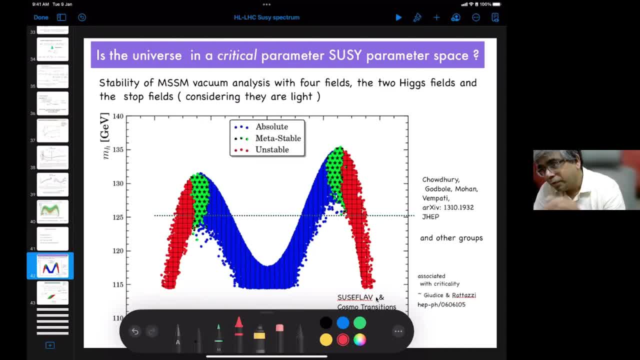 There will be corrections also coming from the A terms. If you have to do it correctly, you have to do it. You have to do this. works what there? So we canceling you will get to 13.1. fibonacciастper Einheit permchlussd� 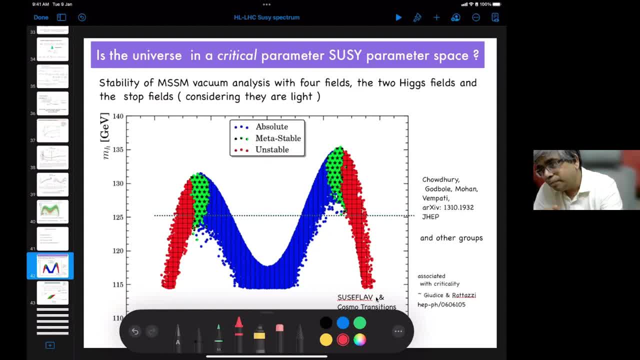 constraints also for the A terms for the, not only for the stops but also for S bottoms, for S tops, S tows, Especially for the, including the higher loops. Yeah, exactly, Because coming from the two loop we have this connection. But of course, 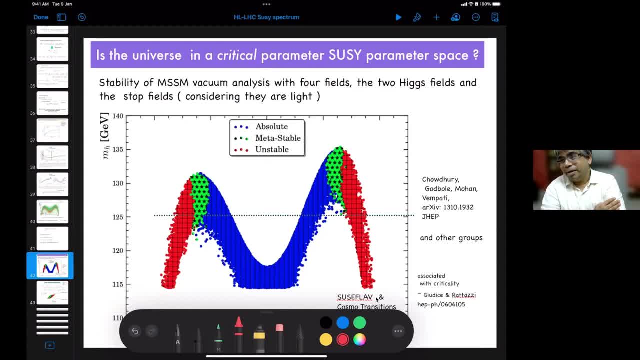 that's numerically extremely hard, Extremely hard, Thank you, Thank you, I think. next Ritesh has some questions. Ritesh Hi, Ritesh, Ritesh, Hello, can you hear me? Yes, Yeah, Okay, Let me just make sure my audio input is yeah, okay. 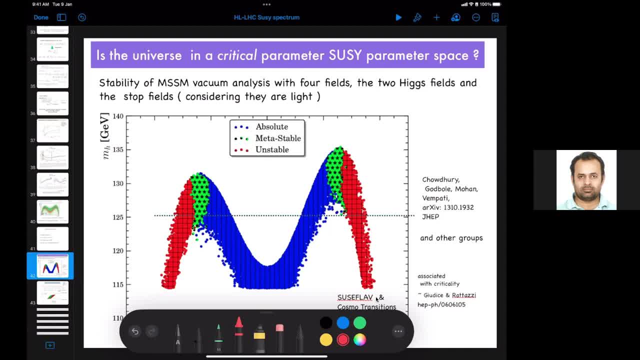 So, yes, So the masses that are involved in this computation, are they one loop or two loop, Or is it the Higgs is two loop and others are one loop, or something like that? In which calculation you are meaning I'm in this plot? 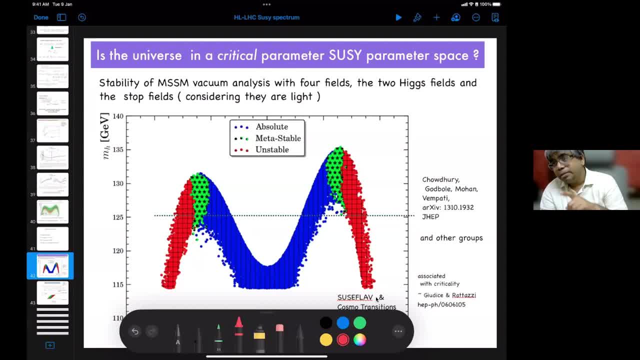 In this plot. They are all one loop. They are all one loop. The Higgs mass is the maximum possible. three loop Higgs mass Total for two loop. Yeah, So best one can do Corrections: Yeah, Yeah, Best that one can do is there. 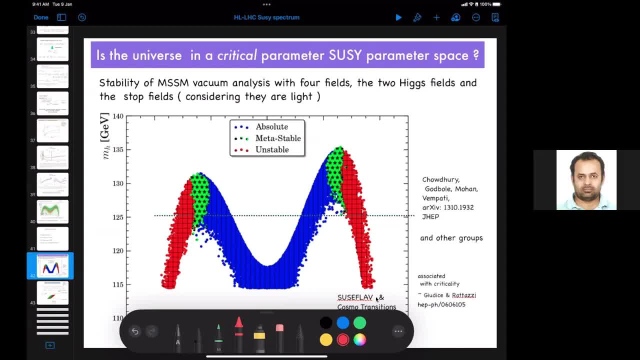 Yeah, Yeah, Okay, That's just confirmed. Yeah, One loop corrections to all the S fermion masses, Yeah, And two loop for the Higgs. Two loop for the Higgs. And this is using effective potential, Using effective potential approach, or just the minimum. 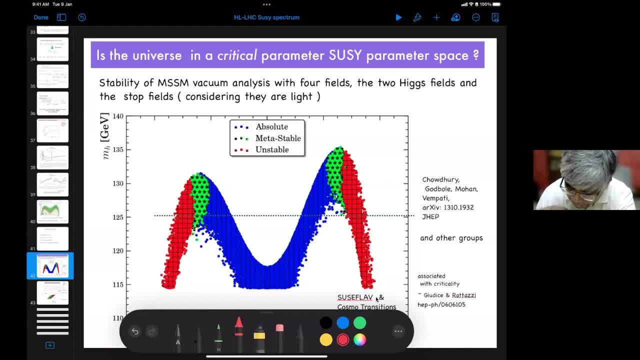 No, actually we did it in a brute force method. We didn't have this new technology at that time. And now there are this analytical calculations by Spinoza and the Japanese person. Okay, And now I think one can do it In principle, one can do a much more better calculation because we have this is purely numerical. 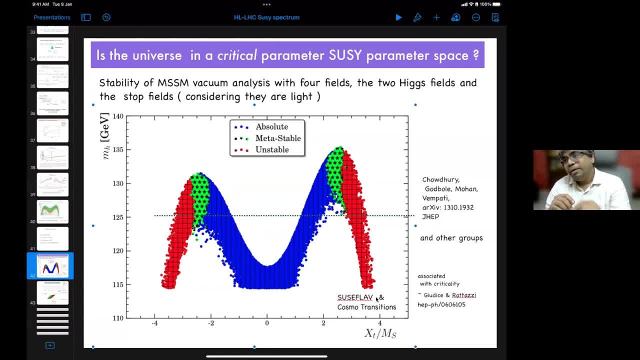 So you take the four field and then look for all possible vacua, step by step, make it into a grid and you know, Yeah, Yeah, It's just super complicated, But I think now there are some analytical techniques for the bound solution. 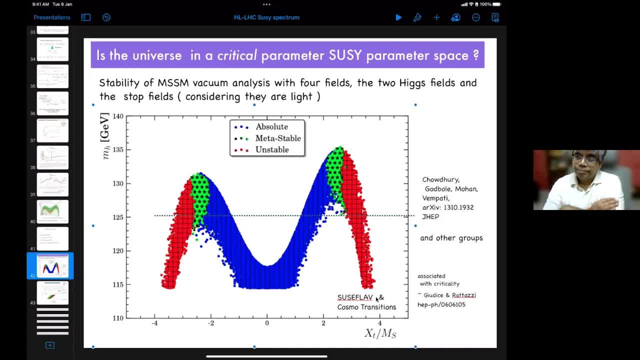 And one can do far better than this. But supersymmetric version, I don't know. They're doing it for the standard model, Okay, But supersymmetric for multi-field, I don't know. I hope it works very well, I don't know. 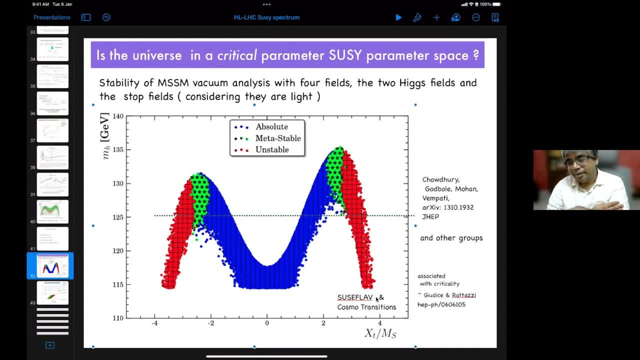 Okay, Yeah, For single sequence, it's far better. Thanks a lot, All right, Anybody else? Any other last question? If not, I don't see any raised hands, So if not, let's thank him again, Oh. 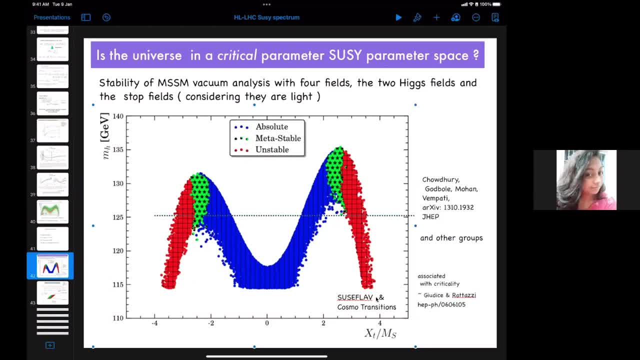 That's the last. Yeah, Go ahead to the corner. So is there any physical interpretation- I mean deeper physical meaning- in the asymmetry of the curve? Hello, Hello, I lost you the last. Okay, I am asking: is there any physical interpretation in asymmetry of the curve? 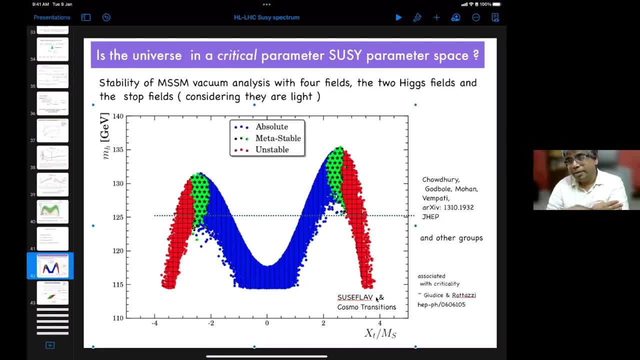 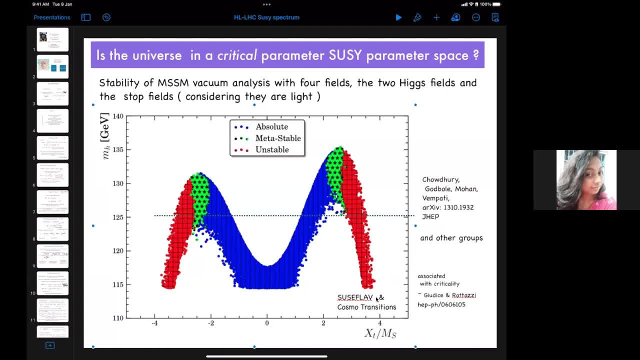 Yeah, Yeah, Yeah Yeah. That is how it is. So what themedenality is workthink the symmetry of day. In this curve, the right-hand side is a. I mean the peak is quite higher than the left one. 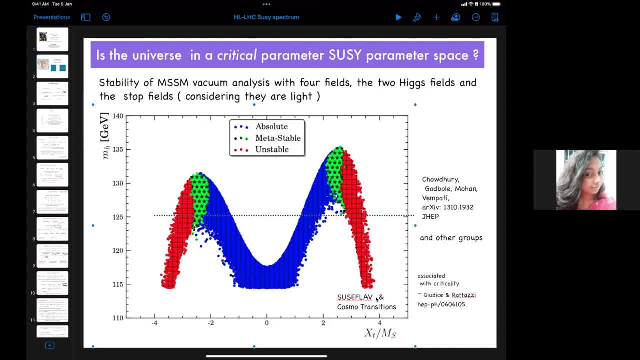 I know meaning you mean to say this wing, the two, many wings. Okay, 0121 is left-hand side and right-hand side. They're not in there. There's no physical significance, It is Just How, Oh. 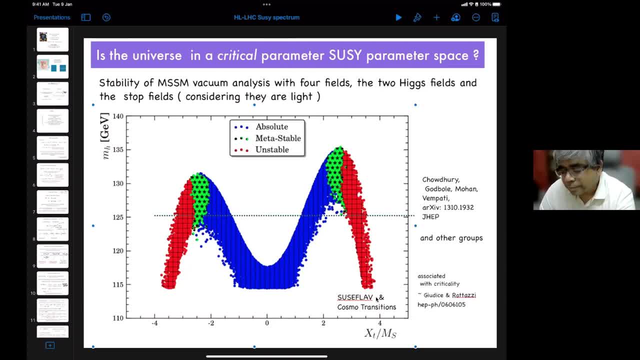 um, if you find supersymmetry, of course there will be some physical significance. okay. so if you want, uh, the stop production cross sections, if you link into, so normally what you do is you don't link the higgs mass calculation with the stop production class calculations, okay, 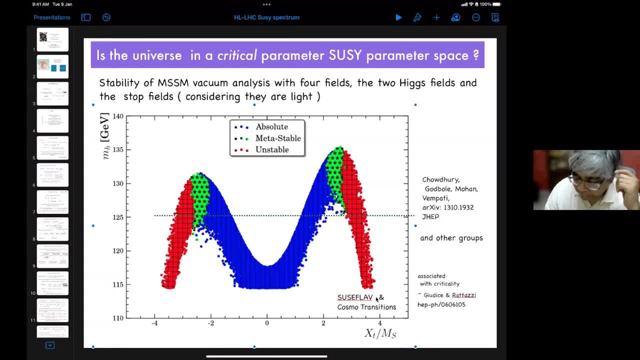 uh, so you are you actually? you're right. there is a very interesting question actually. so, suppose, if i want to know in a supersymmetric theory if supersymmetric theory is real, and so on, so if i want to know whether the universe is stable or unstable, okay, if you want to know the super, the theory is, universe is, uh, stable or unstable, then what? 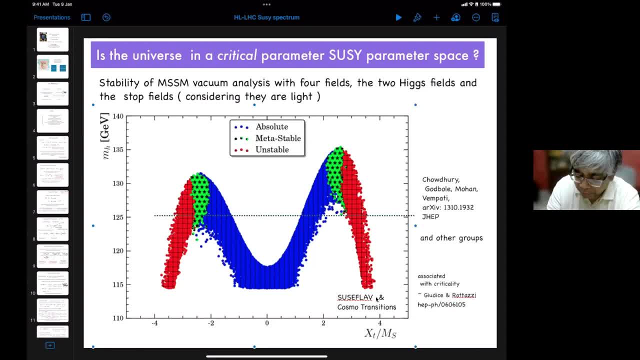 i look at is production of stops and the stops decaying into tops, and i have to find out, uh, the polarization of the tops such that i know the mixing in the stops. so if i know the mixing in the stops i can tell what is the mixing in the stops. 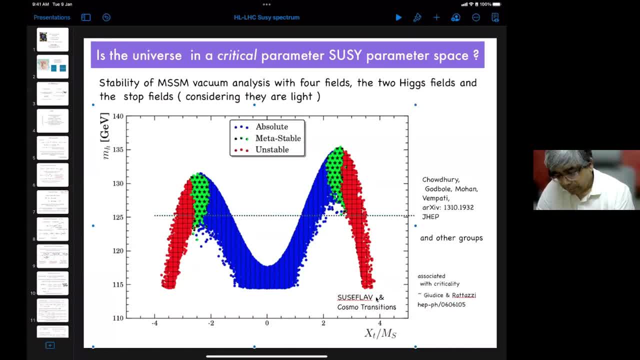 so if i know this mixing in the stops, if i detect tomorrow, if i detect stops, okay, and if i know the mixing in the stops, i will know where i stand actually, whether the universe in the supersymmetric is uh, quote unquote. this is called the study of the criticality. if it is lying within the critical, 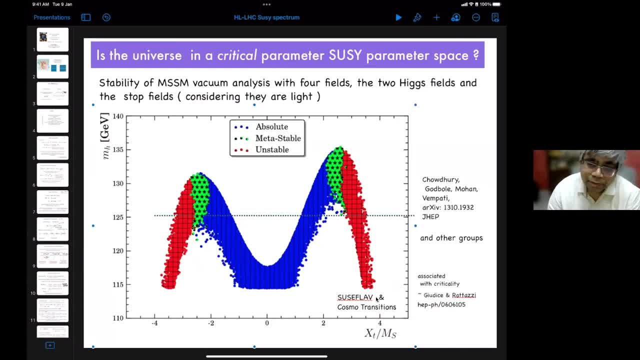 regions of the parameter space or not. but for that one has to study the um tops, meaning you've gotta produce stops enough. stops in the in the lchc, yes, but that is uh. that is actually. i think rictish can answer more because he has. 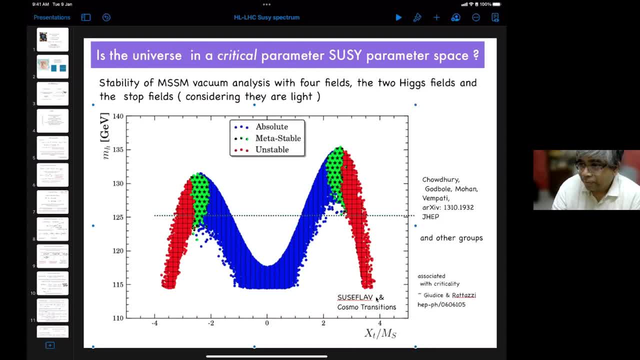 studied the top polarization and everything and converting from top polarization to the candyها think it can be done actually. so if you can get the stop mixing, you'll have really uh know whether what kind of universe you are living in: unstable, stable or metastable universe. 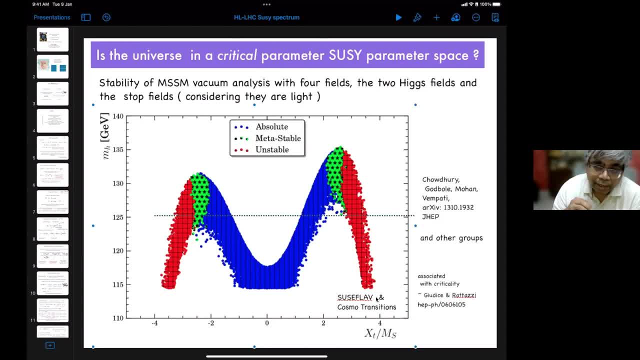 so that is one important aspect of the study. actually, one can actually study this one, but, yeah, i don't think there is an analysis done in this direction. the test can tell it more about it. yeah, to the best of my knowledge, yeah, this distinction is, uh, still at large. the one doesn't. 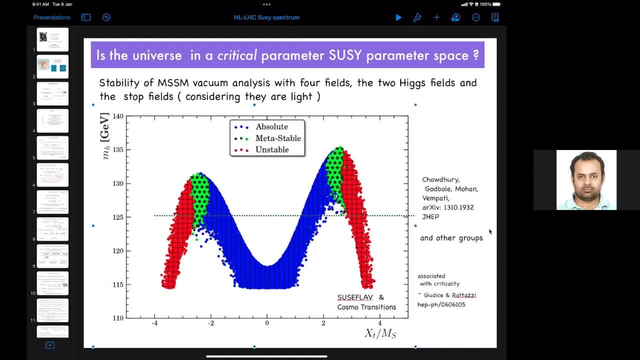 have. i mean, first of all, there is no result, positive result, of finding susie. yeah, this thing makes sense only after we have found this stuff and from the current constraint, it looks like stop is going to be the heaviest of the. all this firmness, yeah, so yeah, like i said,